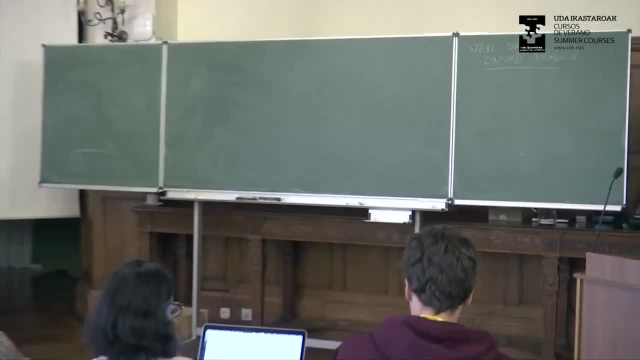 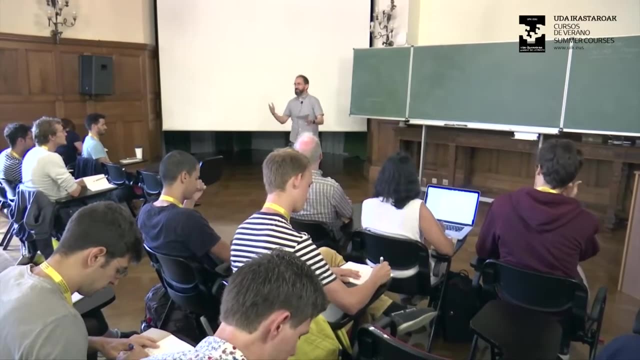 school And you can click on that and you can find all the homework assignments which I'm going to assign to you. You don't have to do them, but they're fun problems and you learn something from doing them. So I'm encouraging people to try to work through. 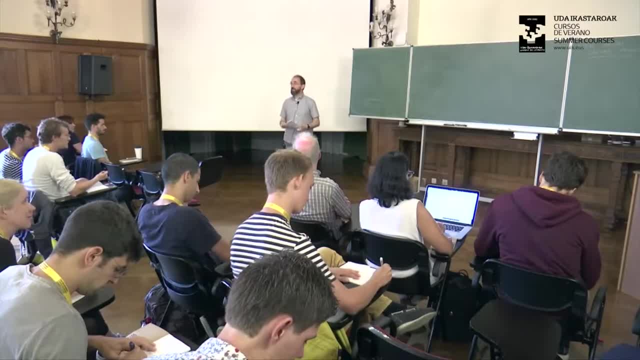 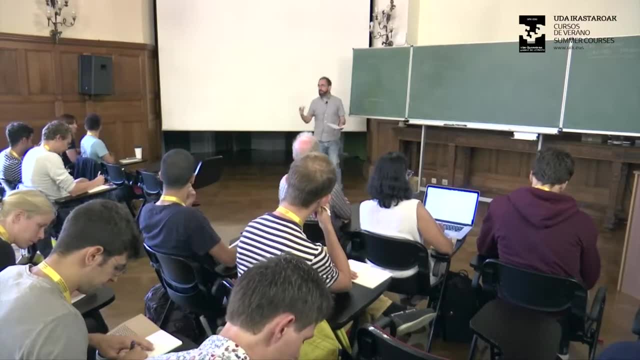 some of these things that I will assign to you as summer school problems, And they're all written out nicely, with all the details in them, on the website. So in this lecture I'm going to talk about integer quantum Hall effect, And we heard 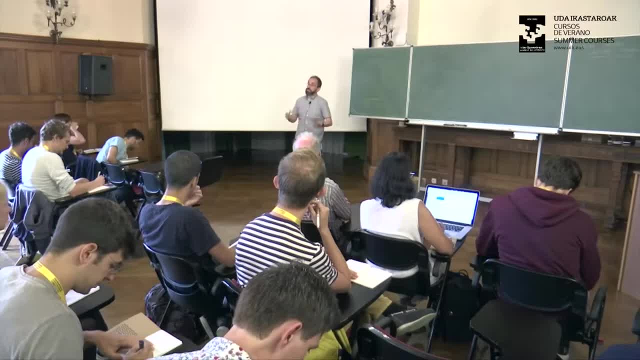 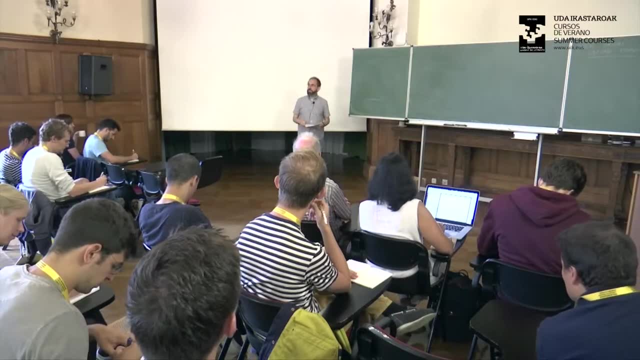 a little bit about that from Charlie earlier. It's one of the simplest, if not the simplest case of topological insulator in two dimensions, And in the next lecture I'll talk about fractional quantum Hall effect. So integer quantum Hall effect is sort of a prerequisite to fractional 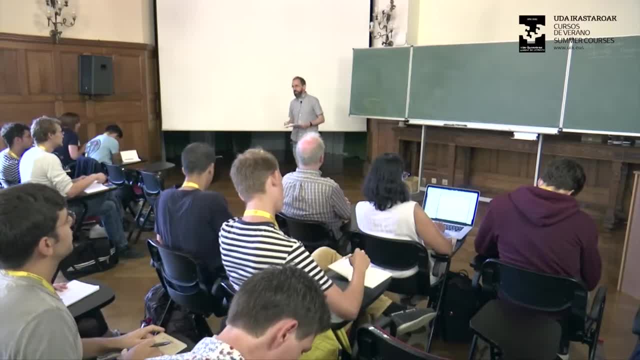 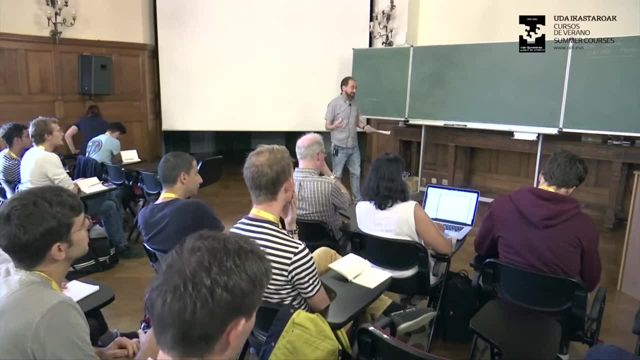 quantum Hall effect. But before we even get to integer quantum Hall effect we have to go all the way back 150 years to 1870., 1879, where we have the classical Hall effect that probably everyone has heard about somewhere in their life before. But I'm going to remind you what it is. So this is the experiment. 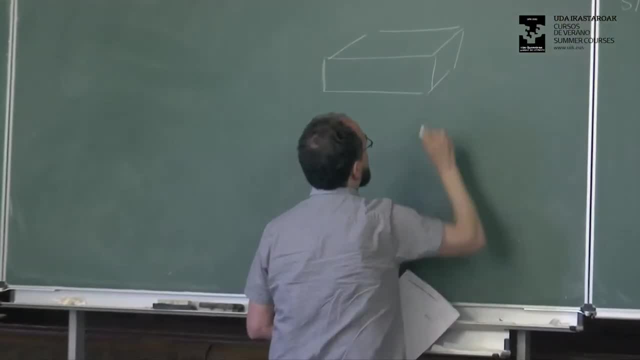 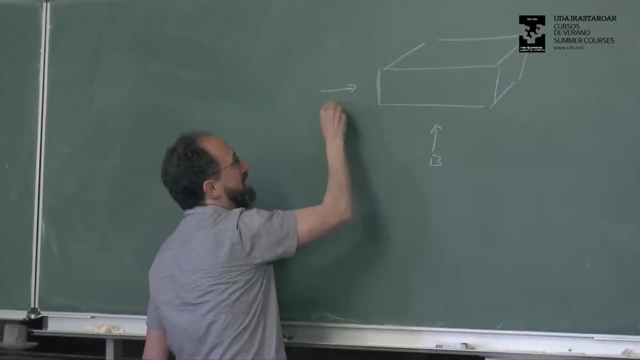 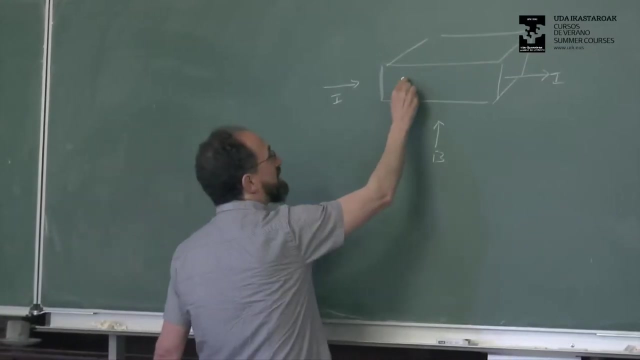 done by Edwin Hall 1879, at Johns Hopkins University. He had a block of metal. He applied a magnetic field to the block of metal, He ran a current through the block of metal like this, And then he can measure two voltages. There is a longitudinal voltage, v1,, v2,, v3,. 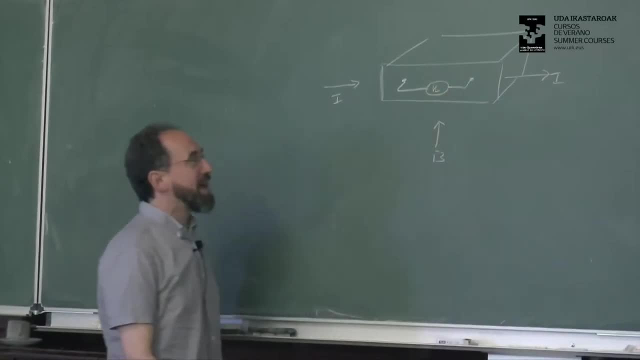 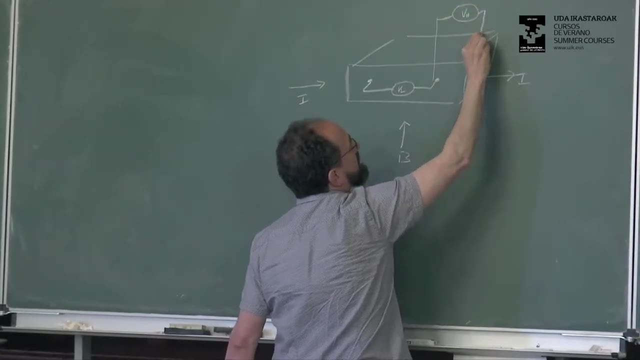 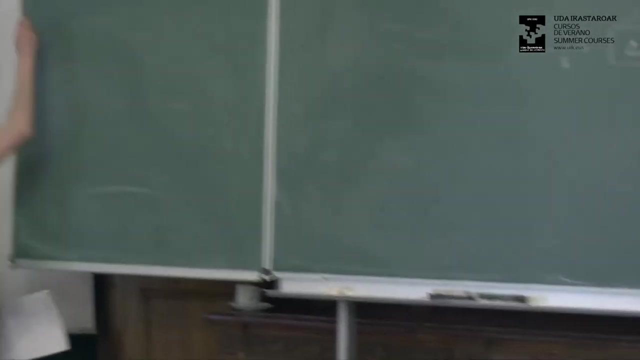 v, sub l, like this, in the same direction as the current, And then there is a Hall voltage which is now called- well, it's now called Hall voltage after Edwin Hall- in the direction perpendicular to the current, And what Edwin Hall measured is kind of like this: a magnetic. 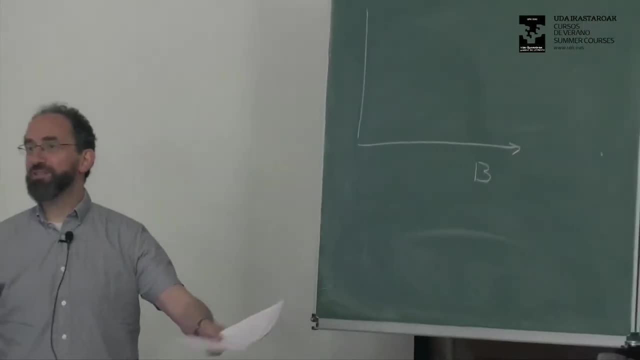 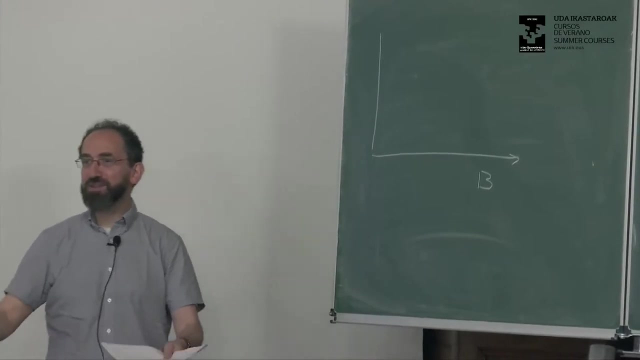 field. Many people will have seen this before. I was told to start from the very beginning, so I will. If you need to fall asleep for a while, please feel free to do so. I'll wake you up when I say something you haven't heard before. 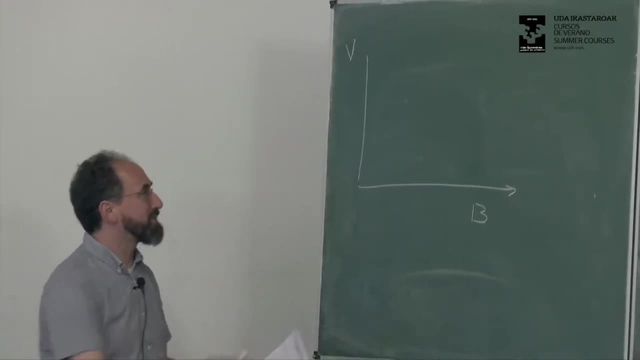 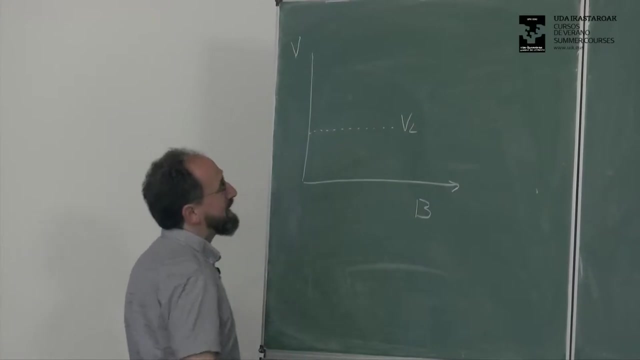 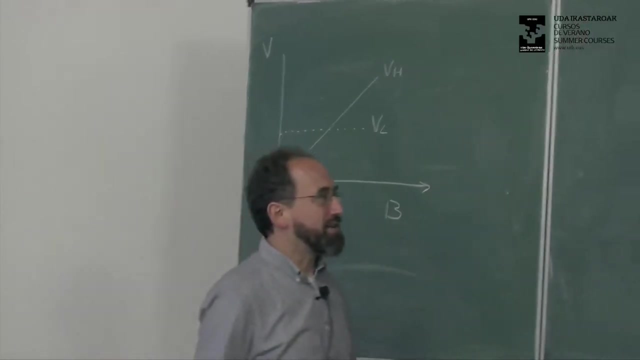 OK, So you can measure these voltages as a function of magnetic field. And what Edwin Hall measured in 1879 was the longitudinal voltage is roughly independent of magnetic field, whereas the Hall voltage is roughly linear in magnetic field. And we understand now through, basically through Drude theory, which is just classical. 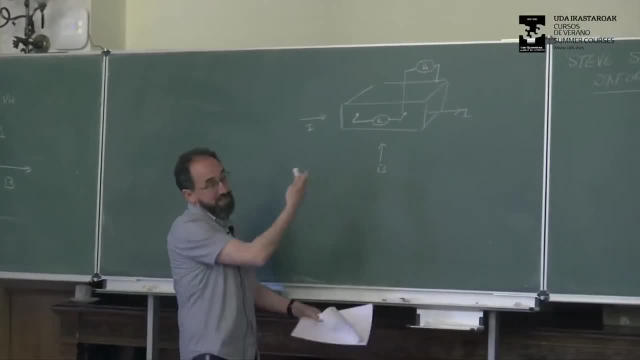 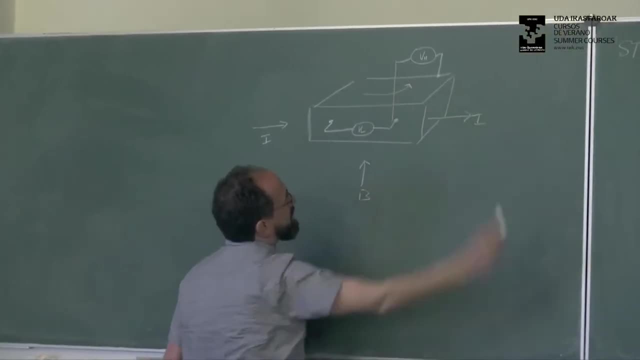 mathematics of electrons running around in the solid. the reason for the Hall voltage being linear in magnetic field is that there's a Lorentz force on moving charged particles. The Lorentz force makes the particles curve to one side of the sample. It builds up a Hall. 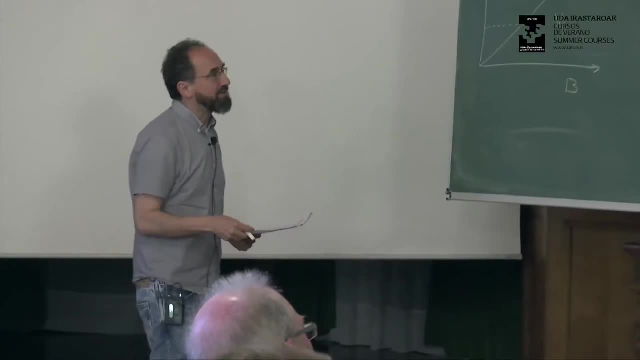 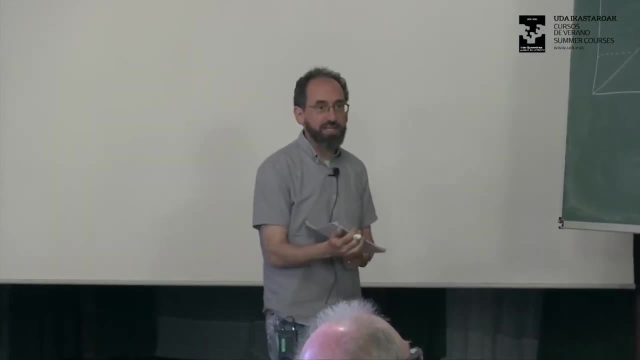 voltage, and that's what you measure proportional to the magnetic field. OK, Now we jump forward in time almost exactly 100 years to 1980.. And in those intervening 100 years two important things happen. So we have two questions. The fundamental answer: how long ago does that begin? tama anything? 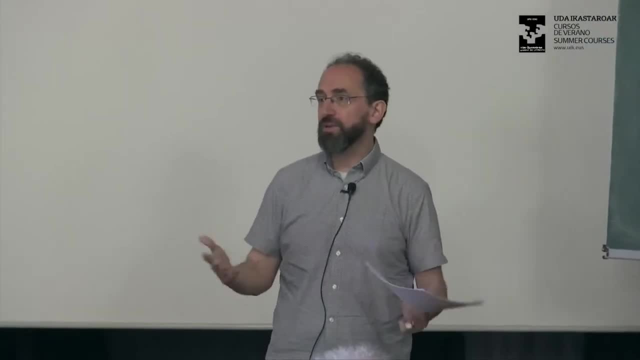 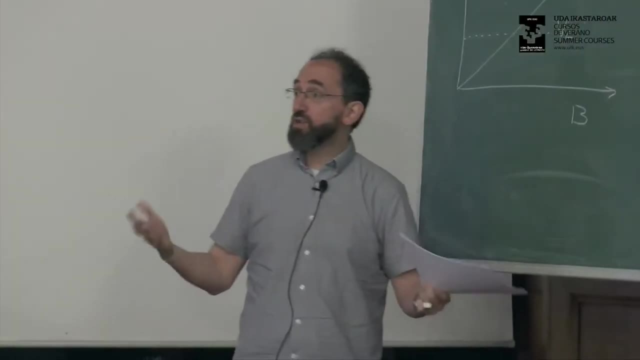 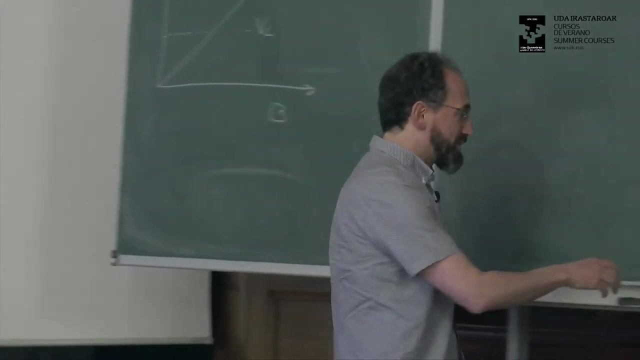 happened? The first important thing that happened was the development of cryogenics, so you can do experiments at very low temperatures, And the second important thing that happened is that two-dimensional electron systems were developed so you can do experiments in exactly two dimensions. So let's change this picture of the sample from a three-dimensional sample. 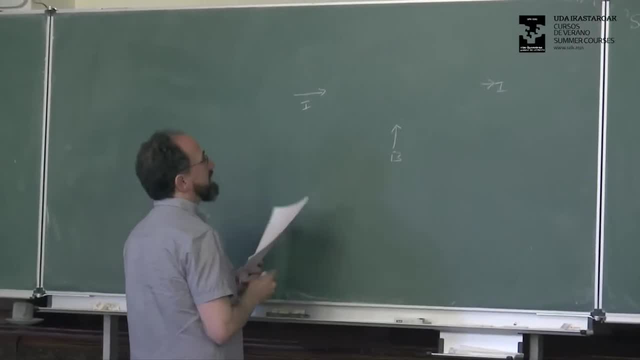 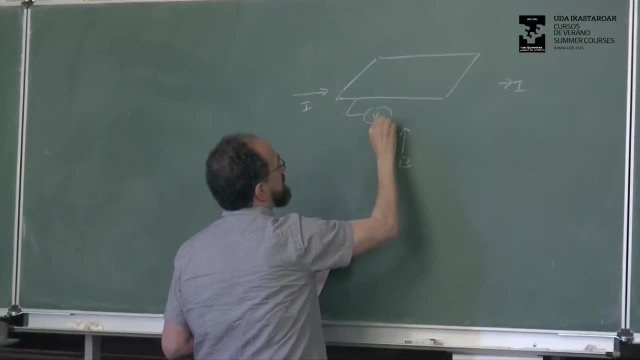 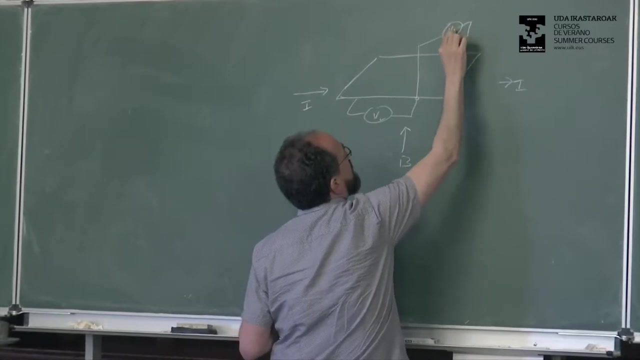 to a two-dimensional sample like this. So now it's a plane. We're going to basically do the same experiment. We're going to measure the longitudinal voltage in the same direction of the current and the Hall voltage perpendicular to the current V Hall, like that, And I guess. 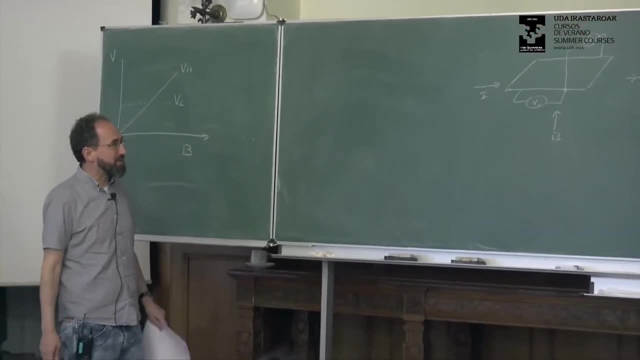 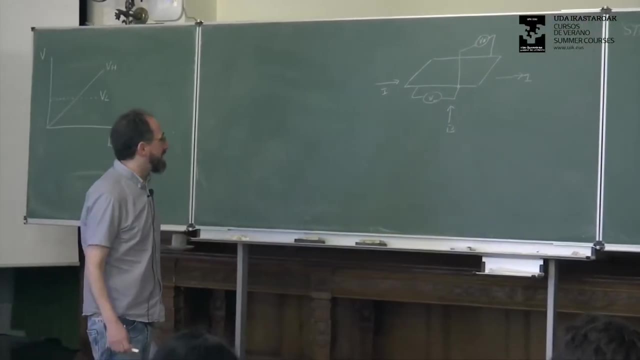 maybe I should just mention, since we're going to hear from Modi about the actual experiments, or some of these actual experiments later on- how is it that you get your experiments to live in exactly two dimensions? What you do is okay, so this direction here. 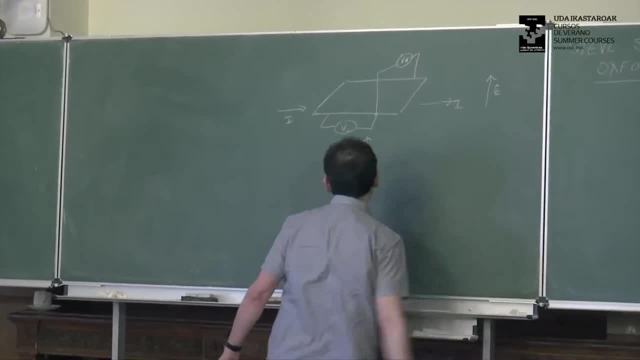 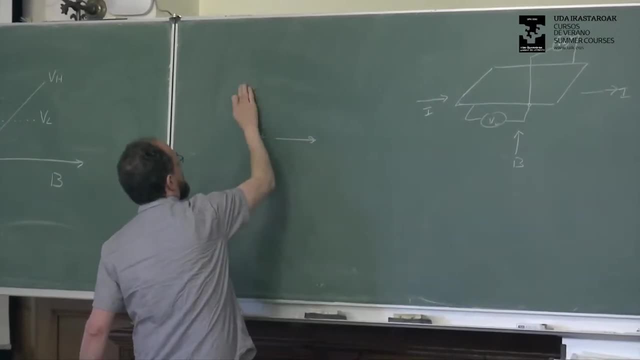 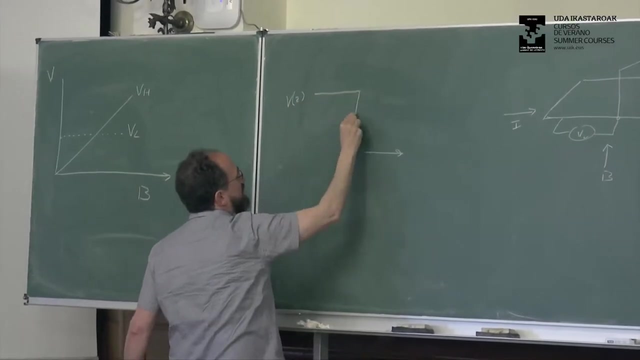 we'll call the z direction out of the plane and let's draw the function of z? z. going this way, There's some potential that the electrons feel called v of z that looks like a particle in a box. potential like this And the way you construct that potential is. 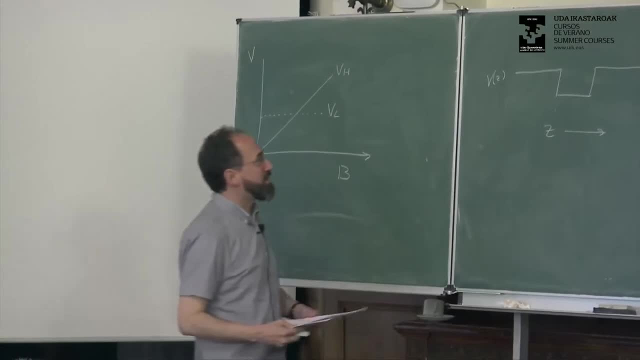 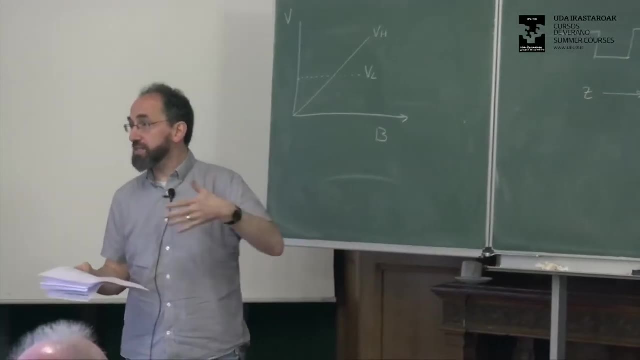 by using mod z. This is modern semiconductor technology. Modi samples: it's gallium aluminum arsenide, gallium arsenide, gallium aluminum arsenide. So the energies of the electrons change as a function of their position. Back in 1980, when the experiment was done by Klaus von Klitzing, 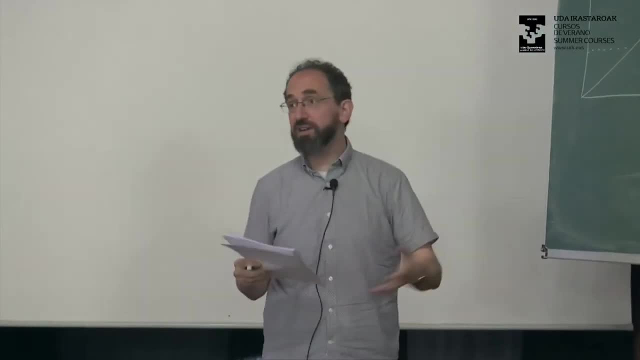 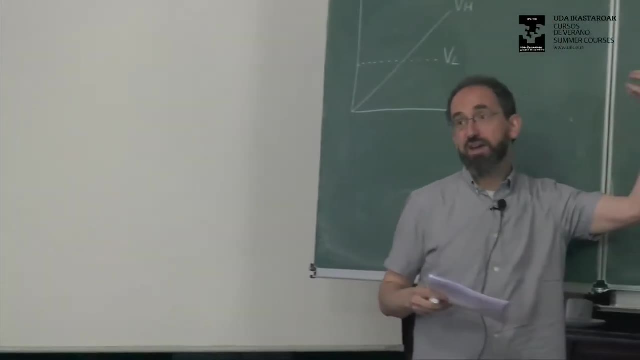 it was actually a silicon sample, slightly different construction, And in modern era it could even be just a single layer of graphene where the energy is lower if the electron sits on the two-dimensional graphene layer and the energy gets very high if you try to. 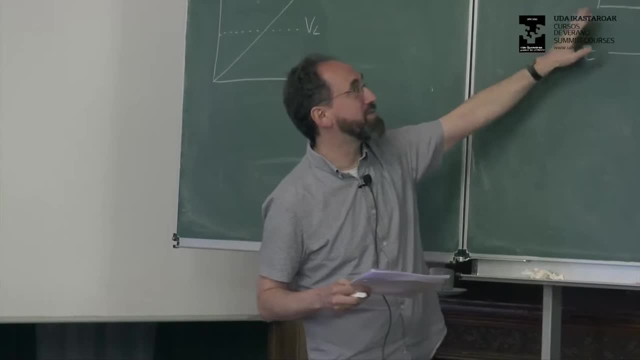 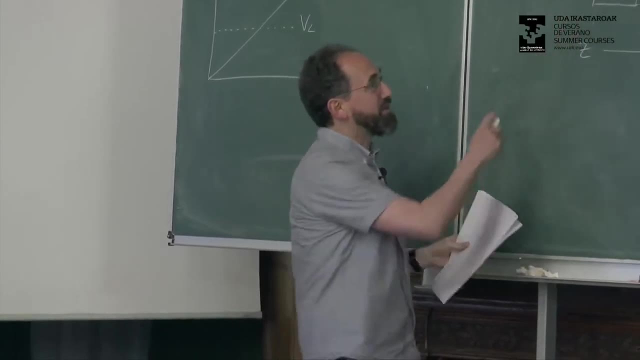 take the electron out of the two-dimensional layer. But either way you look at it, there's some sort of particle-in-a-box type potential, or some potential well, for holding the electron in a particular region of the z direction here, So you can have a lowest wave function. 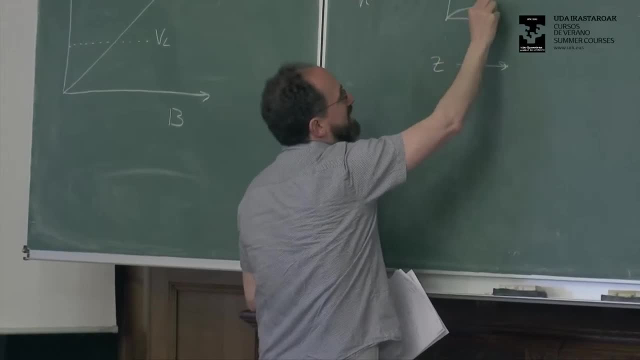 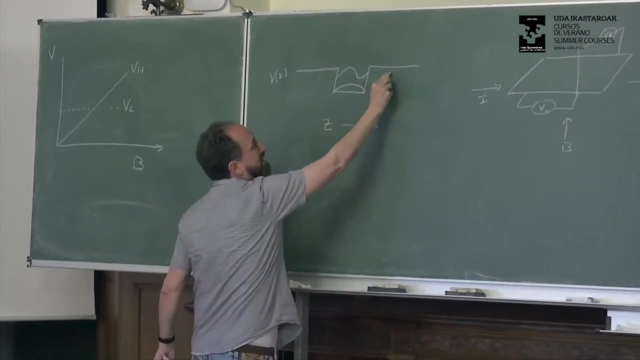 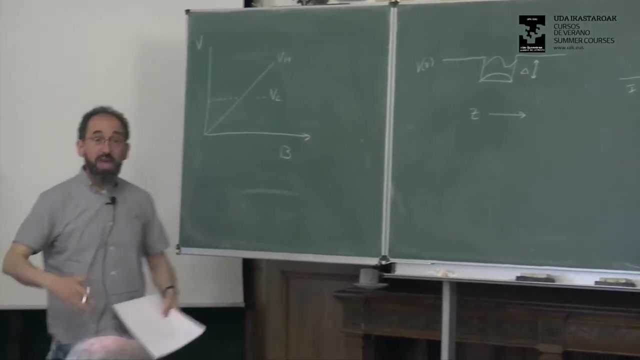 in the particle-in-a-box looks like this And maybe a first excited state that looks like this and maybe some higher excited states, And there's some energy gap between the lowest state particle-in-a-box state and the next lowest particle in a box state with some energy between those two. 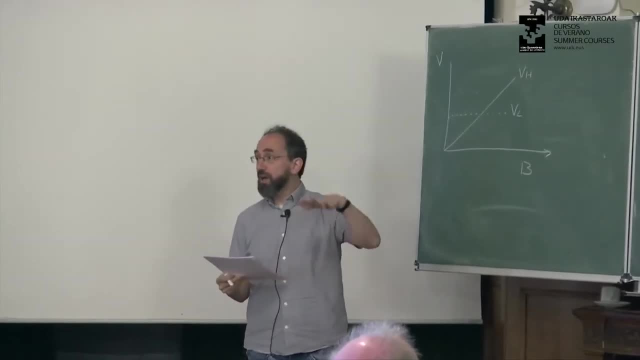 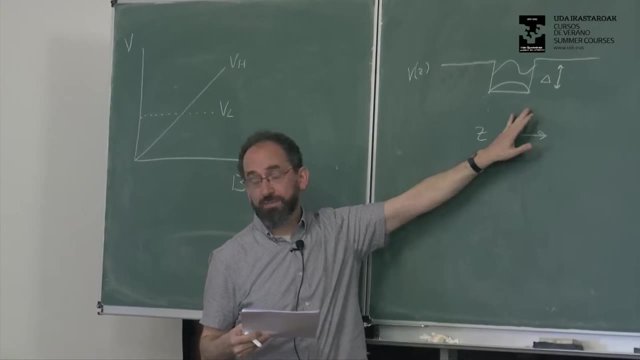 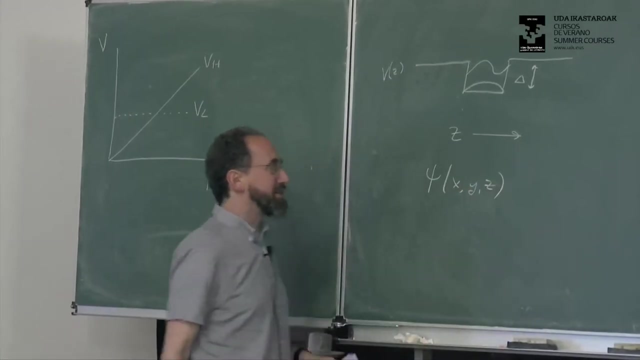 And the idea of two-dimensional electron physics is: you keep the temperature of the system sufficiently low that electrons are completely trapped in the lowest particle in a box state. So wave functions will generally be written psi of x, y, z for our electron wave function. 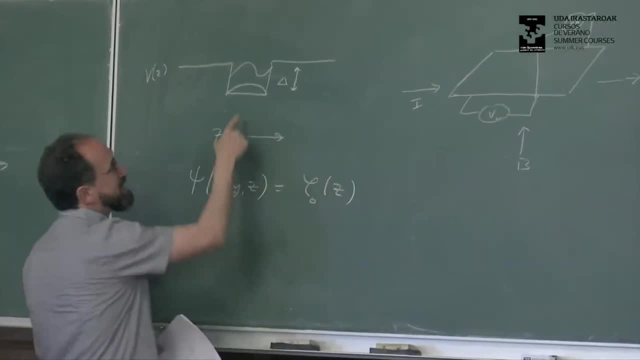 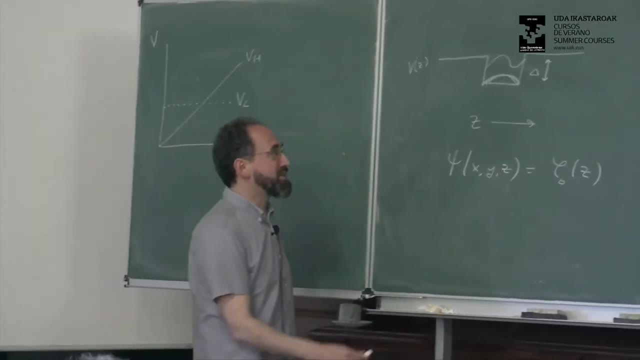 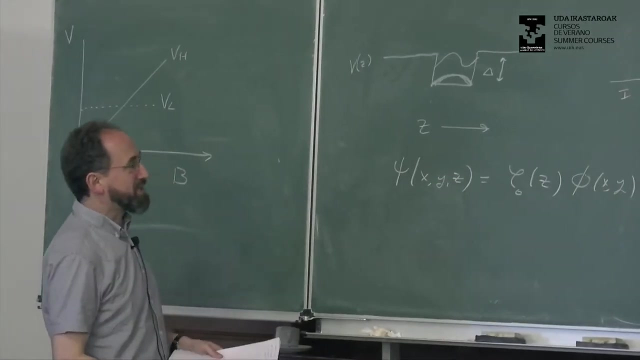 They'll be written as some wave function in the z direction, which is completely frozen in this shape of the lowest single particle in a box state, And then there's some wave function in the other two directions, which still have freedom, So the electrons can run around in the two dimensions freely- x and y- but their degree. 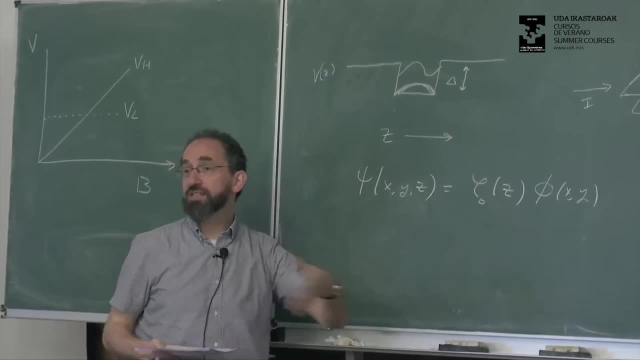 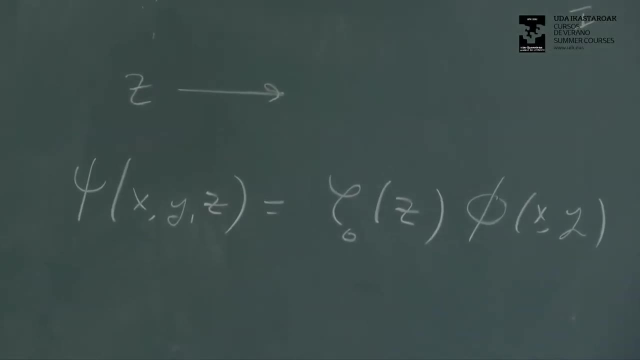 of freedom in the z direction is completely frozen. So that's how you get something that is strictly a two-dimensional, strictly two-dimensional physics. There's no freedom to change its wave function in the z direction. Is everyone good with that? Yes, 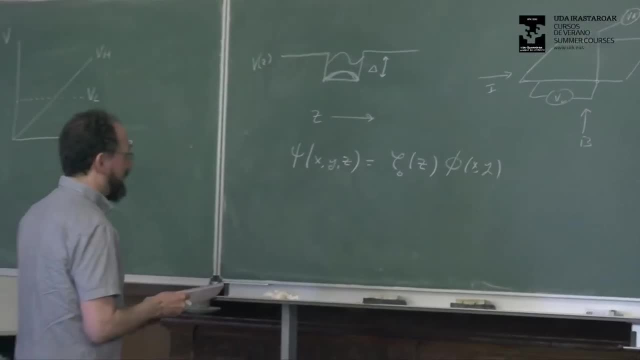 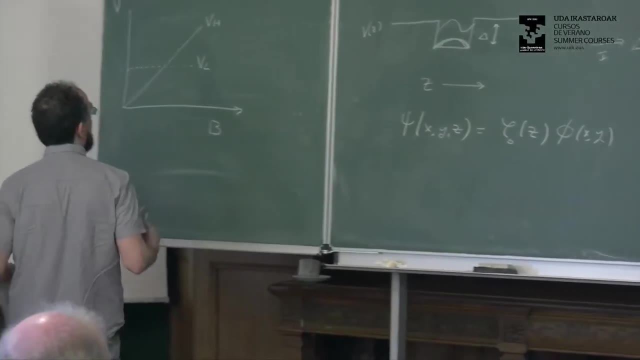 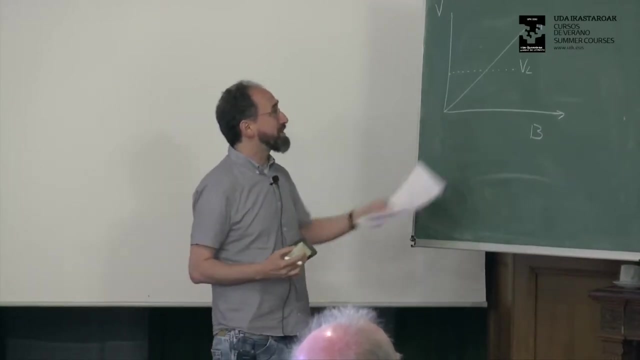 Nod: OK, good, All right. So Klaus von Klitzing, in 1980, went to the high magnetic field lab in Grenoble and took his two-dimensional electron sample and cooled it down to a degree Kelvin or so and measured. 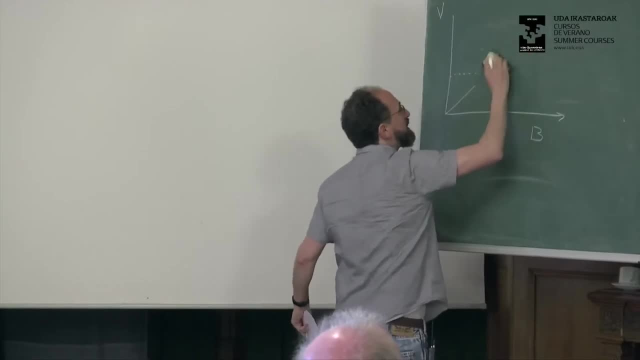 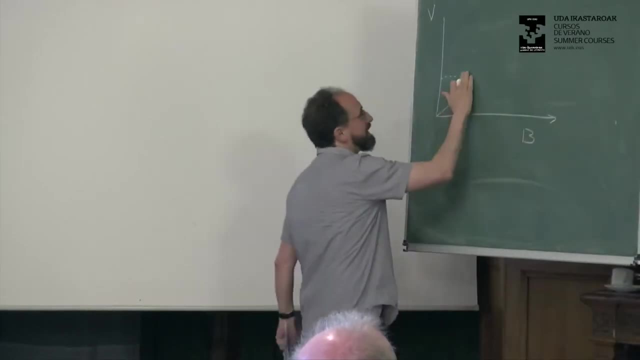 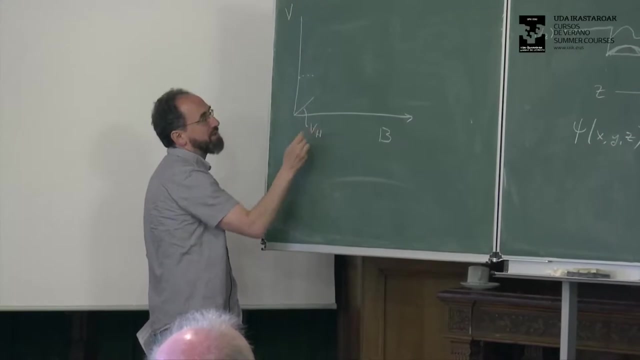 the various voltages And what he found. while at low magnetic field, what he found looked an awful lot like what Edwin Hall found 100 years earlier. He found at low magnetic field. the Hall voltage, The H, is linear in magnetic field and the longitudinal voltage, VL, is roughly constant. 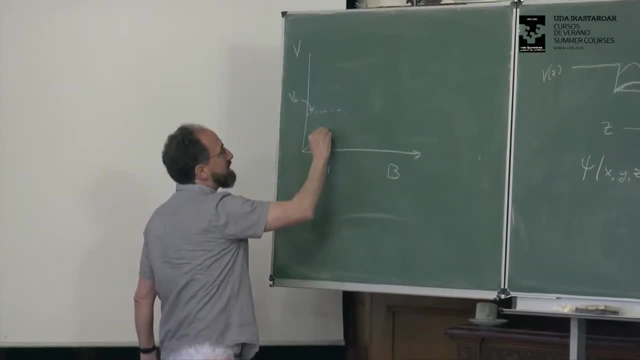 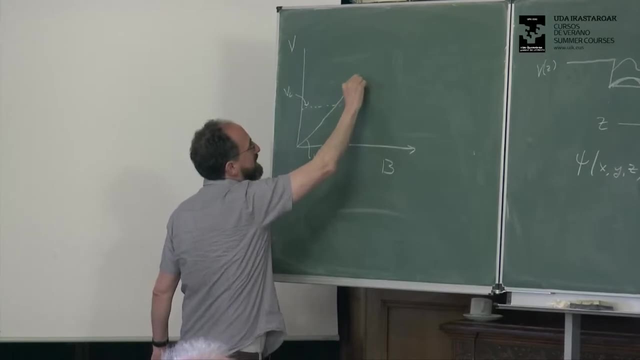 And then things got interesting. He went up to higher magnetic field and the longitudinal voltage starts to oscillate. And then at some point the longitudinal voltage comes down to zero. And when the longitudinal voltage comes to zero, the Hall voltage forms a plateau. 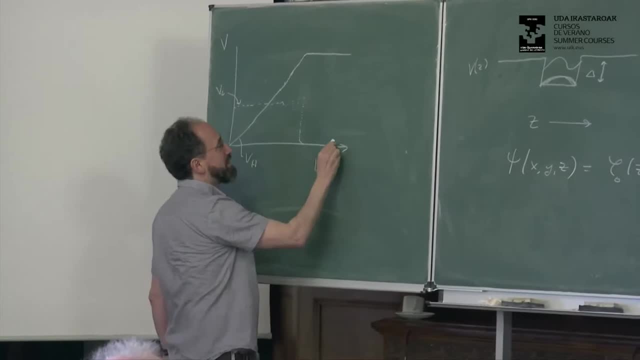 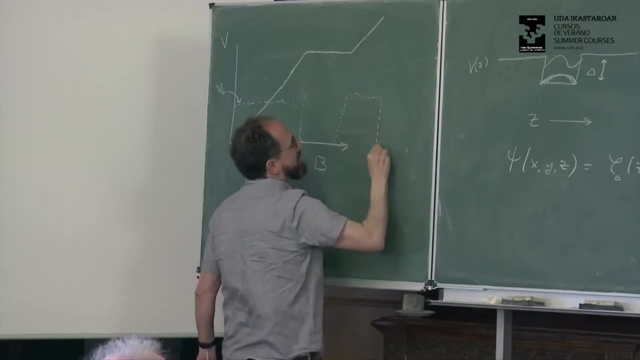 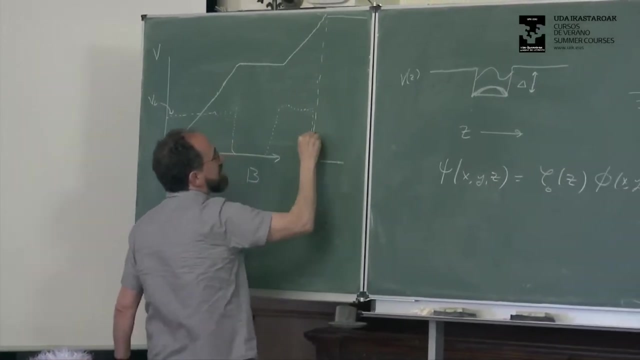 So it becomes completely flat And then after some amount of time it comes back up. This goes back up, And then maybe there will be another plateau where this comes back to zero again. This is badly drawn. This plateau is supposed to line up with the place where this is zero. 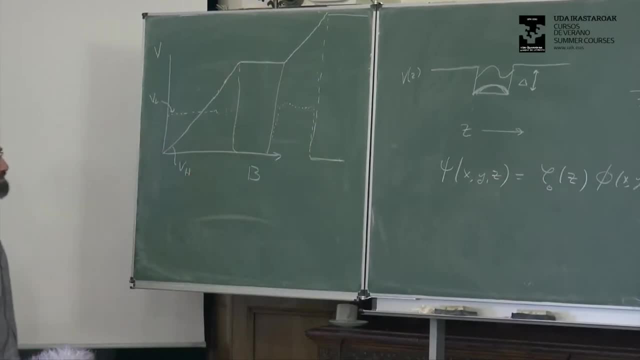 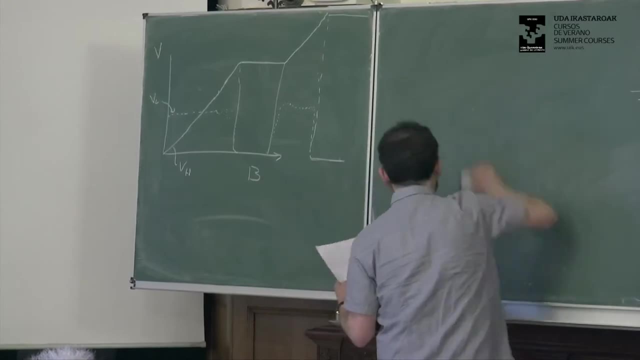 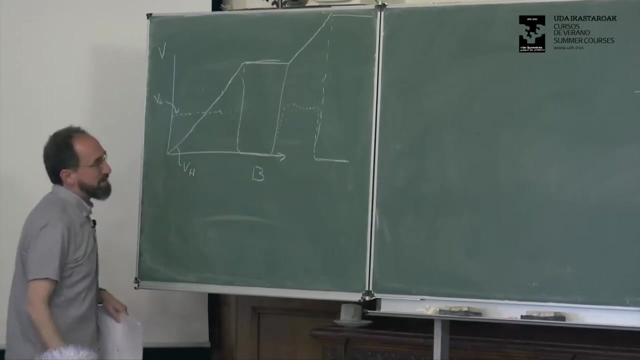 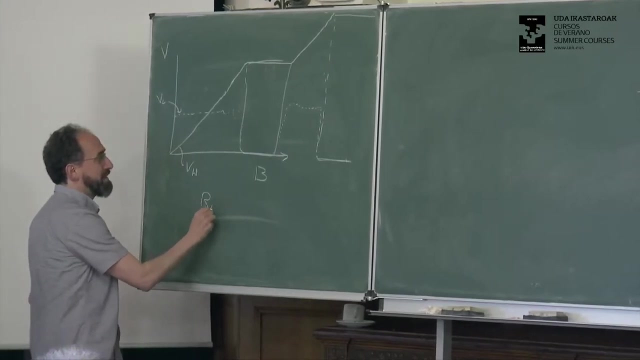 This is supposed to line up with this. Good, OK. So what do we know? These are the quantum Hall plateaus. And what do we know about these quantum Hall plateaus? Well, the first thing is that the longitudinal resistance is zero. RL equals zero meaning. 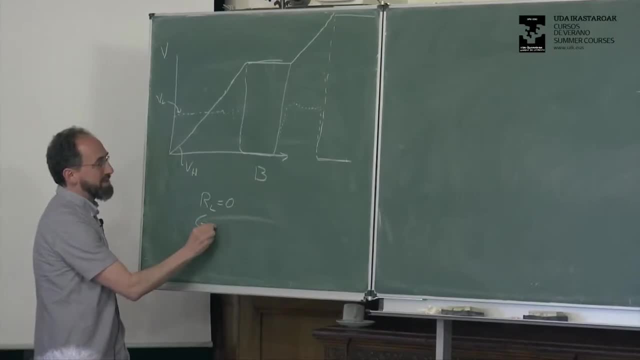 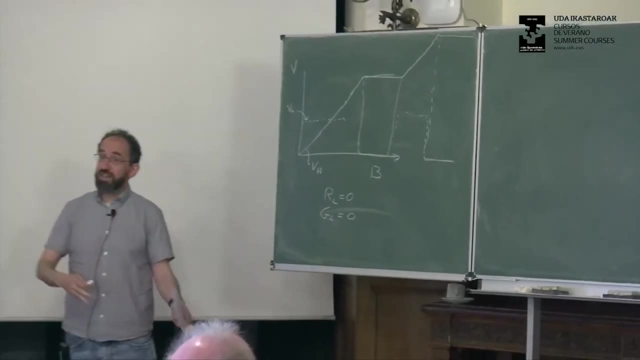 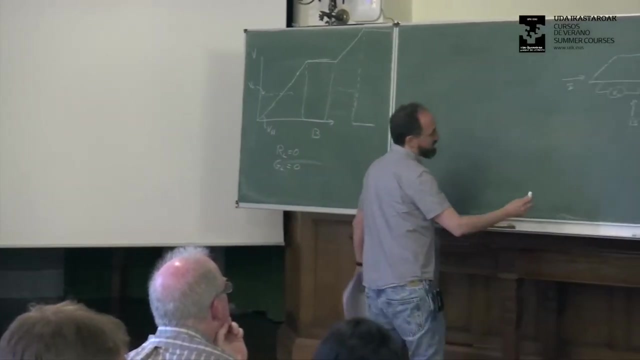 zero voltage here, But we can also say that the longitudinal conductance is zero, And this seems to be a little bit confusing, that you have both conductance and resistance being zero at the same time. But if you think about it for a second, it's actually not so confusing. 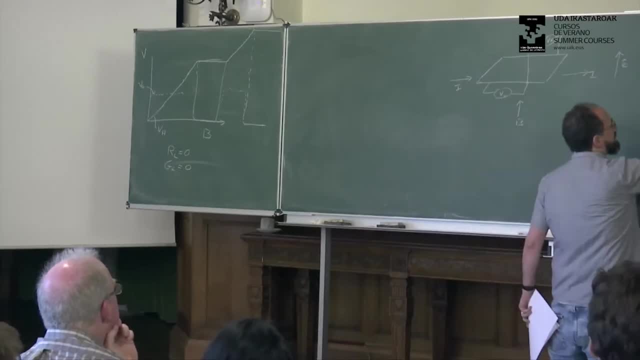 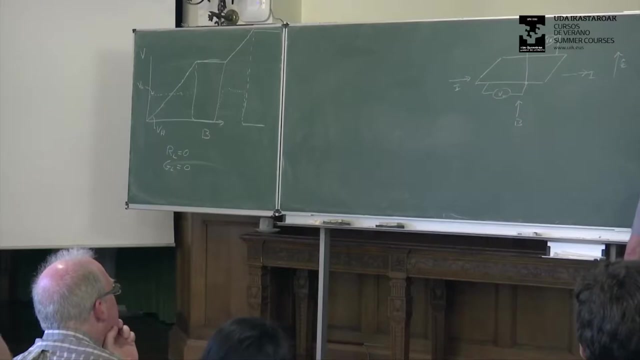 What we actually have is that there's some current density, which is a two by two matrix sigma times the electric field, And what we're saying is that this matrix sigma is off diagonal, completely off diagonal, zero on the diagonals, And it's some constant S on the off diagonal. 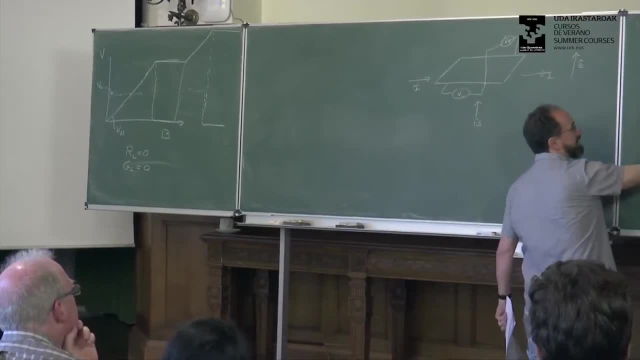 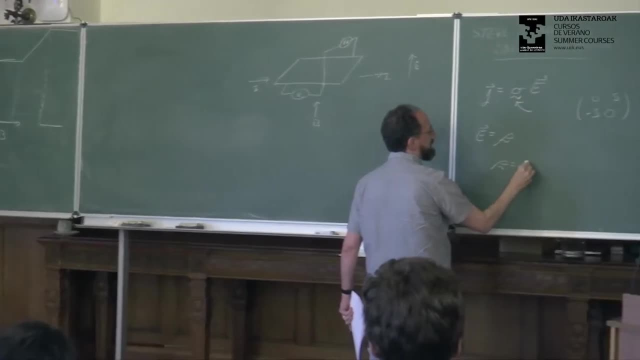 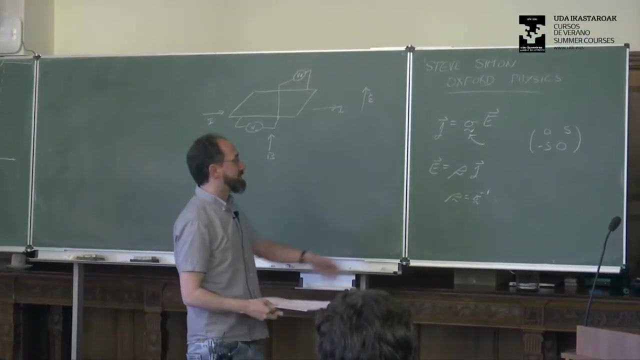 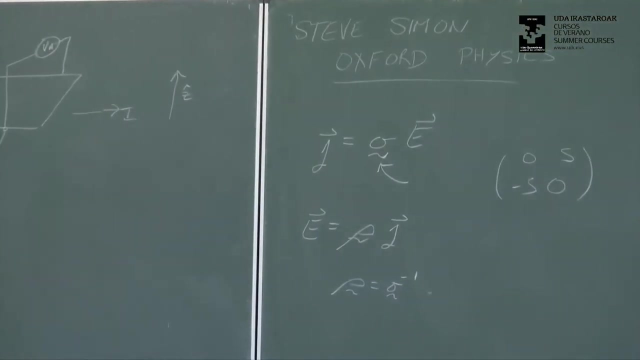 And then if you take this, This matrix, and you invert it, so E is rho, with rho being equal to sigma inverse, sigma inverse times j, The resistance resistivity matrix. this resistivity matrix is also completely off diagonal, So the diagonal parts of both the conductivity tensor and the resistivity tensor. they're 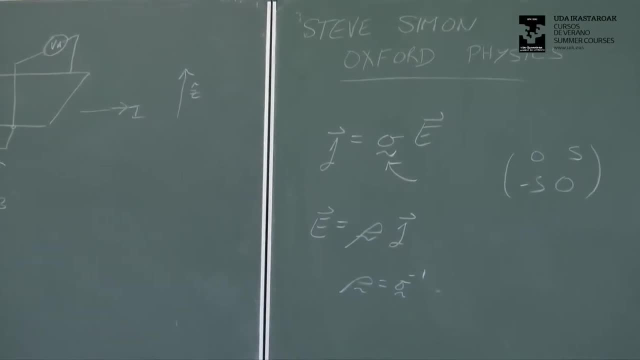 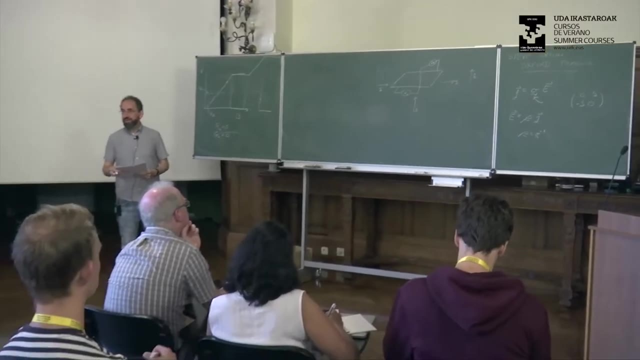 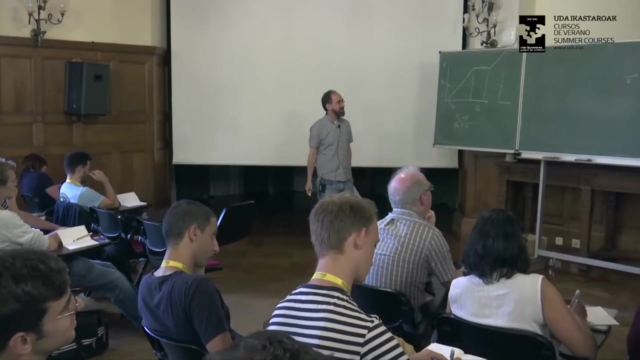 both zero, just meaning that the current is flowing exactly perpendicular to the voltage. OK, To the electric field. OK, Is everyone good with that? OK, Good, Thank you for nodding. Good, All right. So this actually brings me to one of the first exercises that I want to assign for 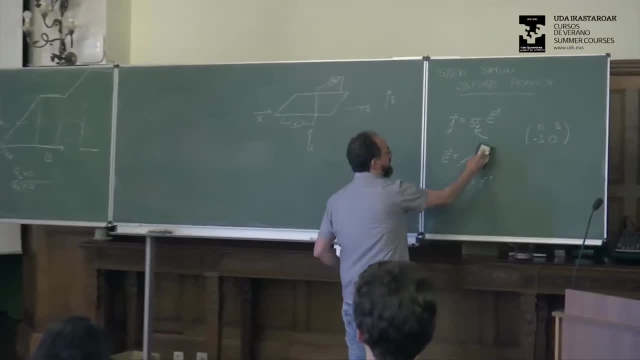 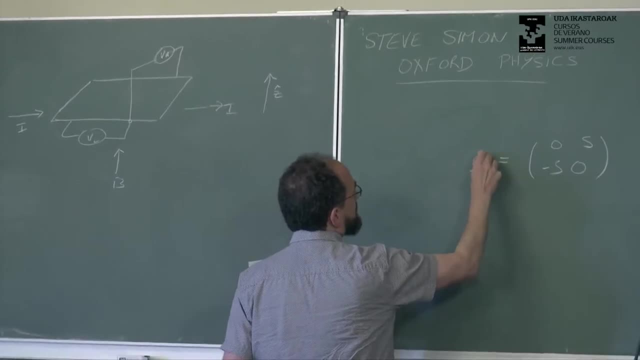 homework And the exercise goes like this: Suppose you have a conductivity tensor of this form where everywhere in the system the current and voltage- Oops, I just erased what we need- Current equals sigma times E, And then you have this: 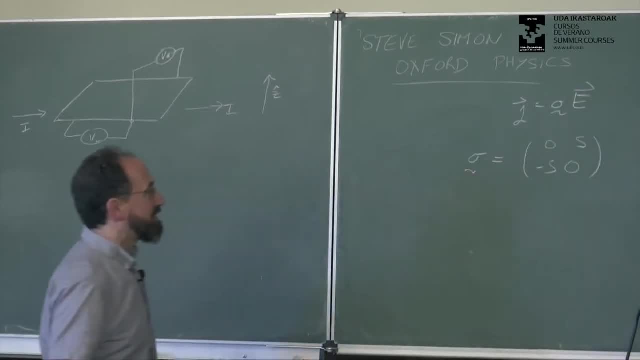 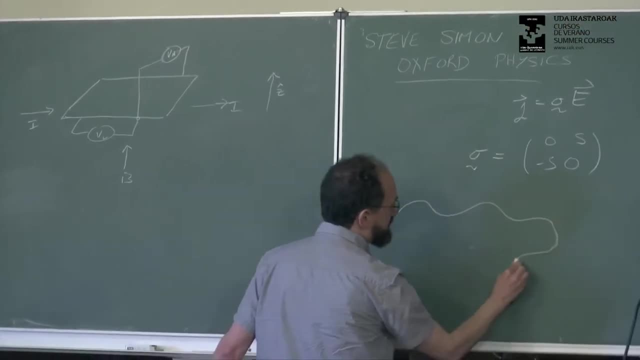 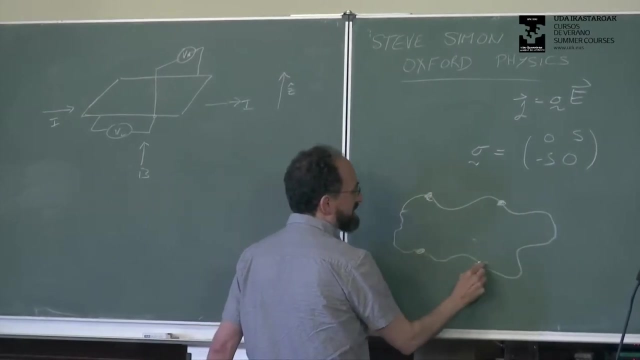 OK, So the current and the electric field are related by this equation, with S being some arbitrary constant, And you have a sample in two dimensions with an arbitrary shape. You don't know what the shape is And you put contacts on the edges of the sample, like this: 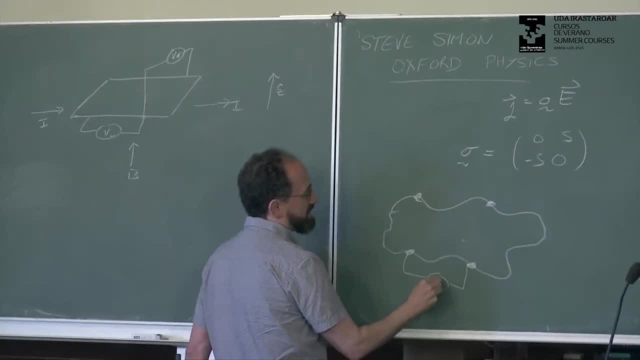 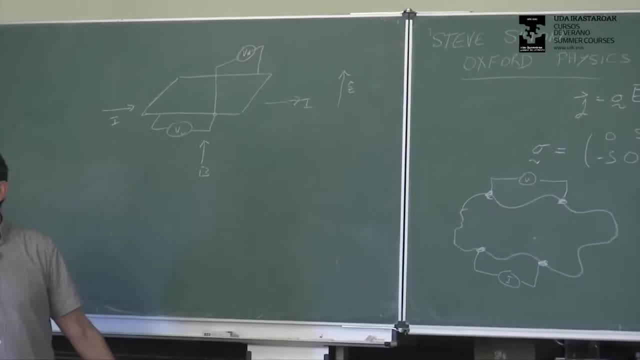 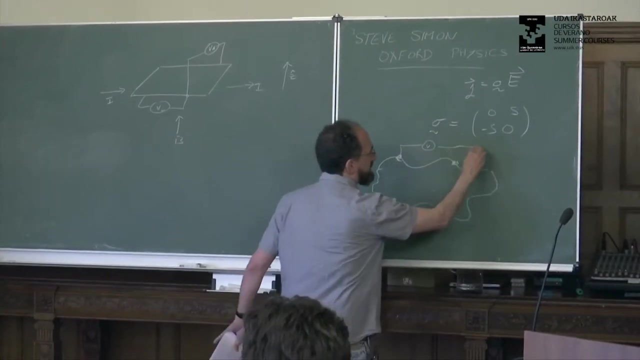 If you run current between two contacts which are adjacent to each other and you measure voltage between the other contacts, show that the voltage always comes out zero in this case. And if you cross the wires such that you're measuring a Hall voltage, so this contact 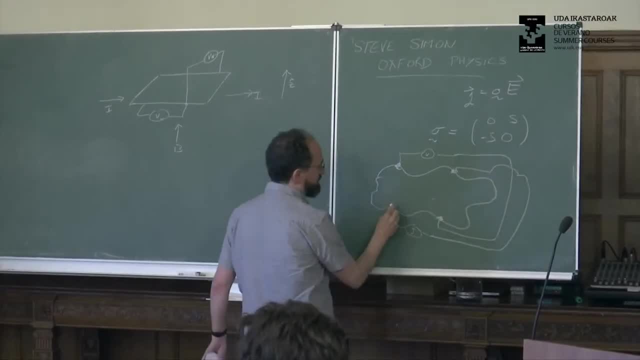 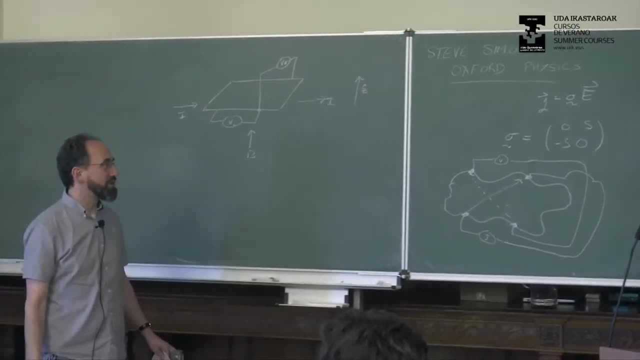 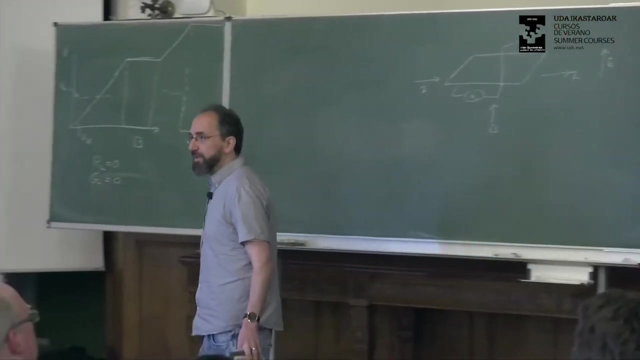 goes here and this contact now goes here, so you're running current from here to here and measuring voltage from here to here show that the voltage you measure is independent of the position of the contacts and the shape of the sample. OK, So that's an exercise. 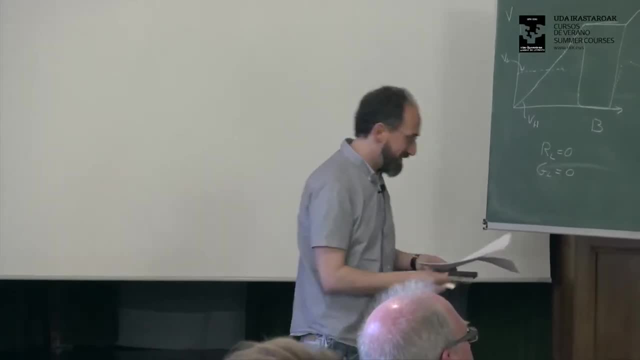 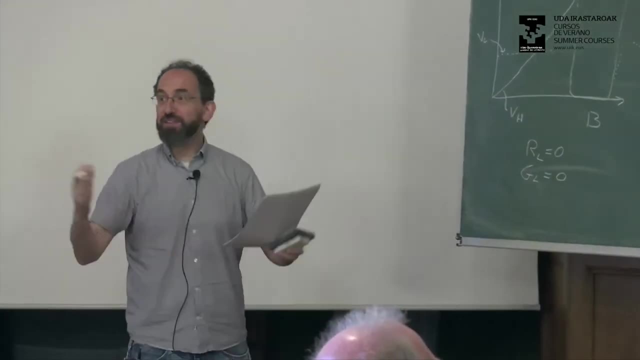 It's written up much nicer If you can see it, If you go to my website so you can try that out. OK, Everyone happy with that? This statement? OK, Yell, if you're not or have any questions, OK. 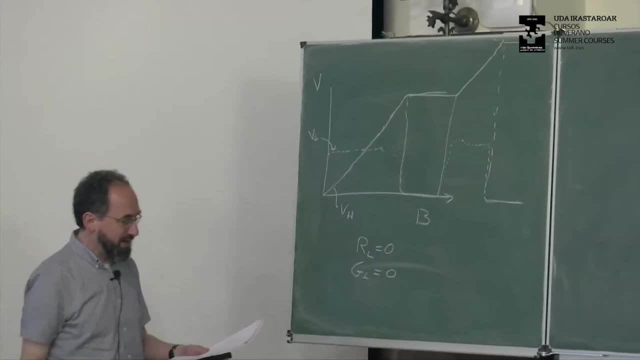 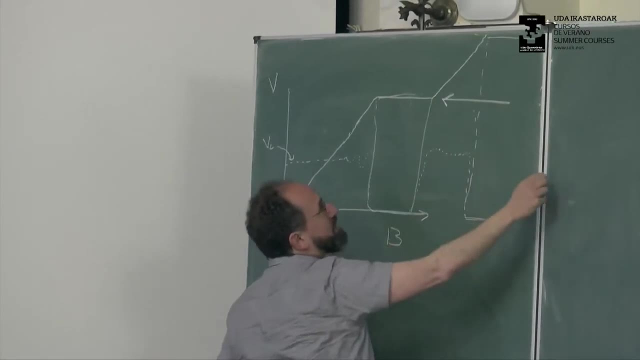 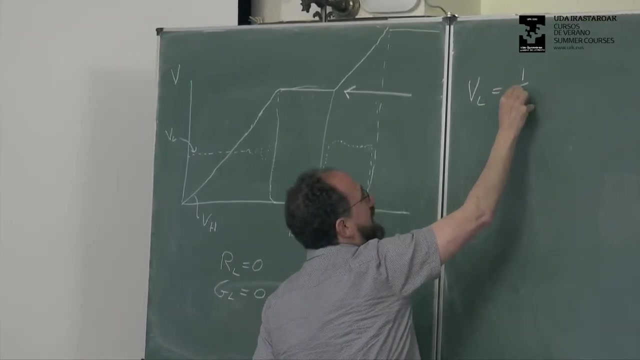 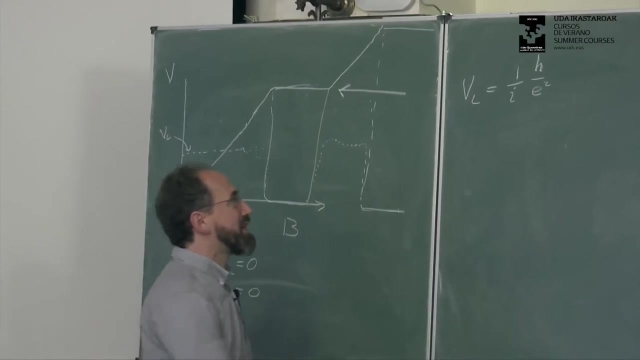 So what else did we? did Von Klitzing measure here. The main thing he measured, or I pointed out, was the value of this plateau, that the voltage on this plateau is 1 over an integer called the integer i, h over e, squared where h is Planck's constant, e is the charge of the electron times, the current. 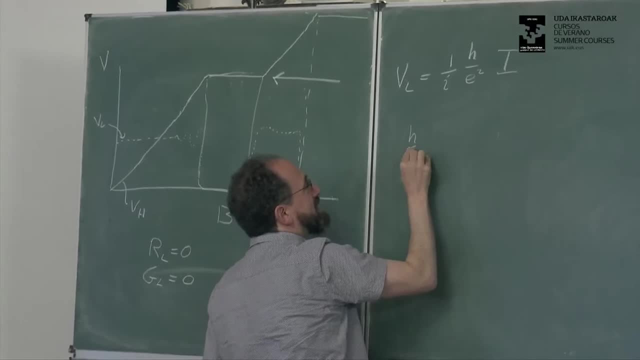 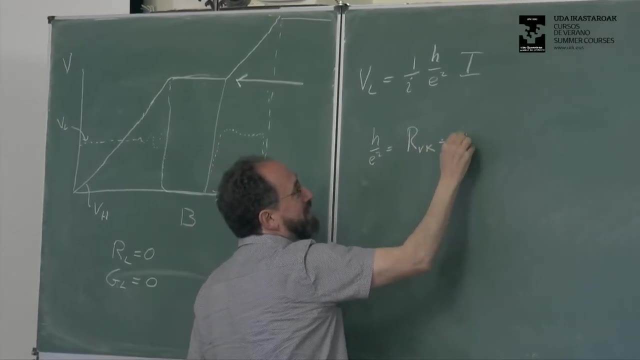 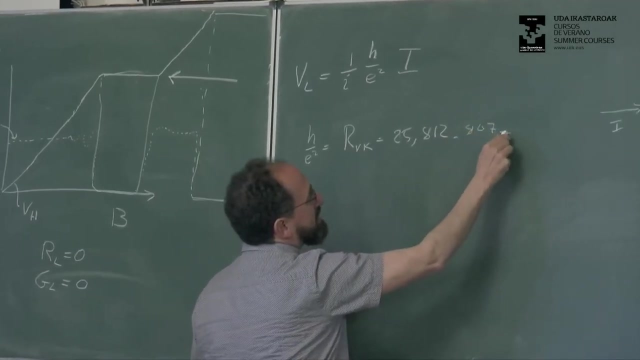 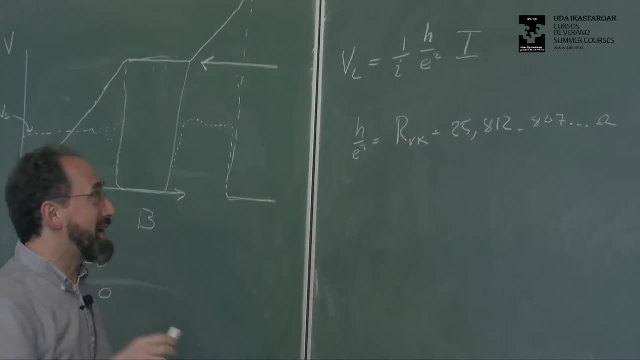 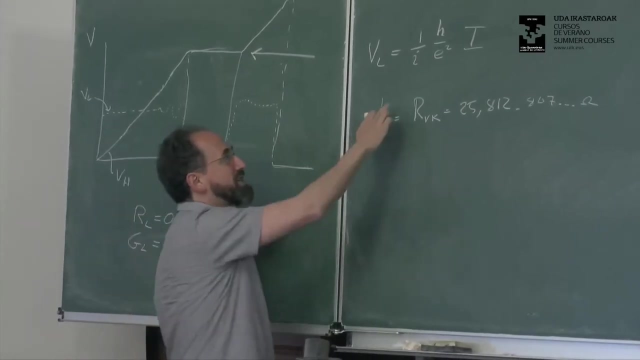 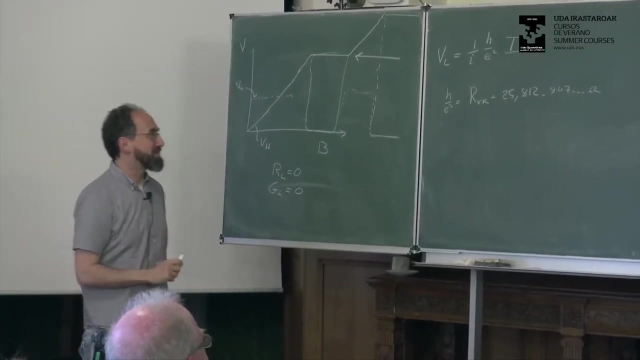 Yes, this is the h over e squared is now exact, is now in the new system, international of metrology It is h and e are both numbers that are precisely defined, that those are exact statements. So the Von Klitzing constant is exactly defined, some number which has 14 digits and that. 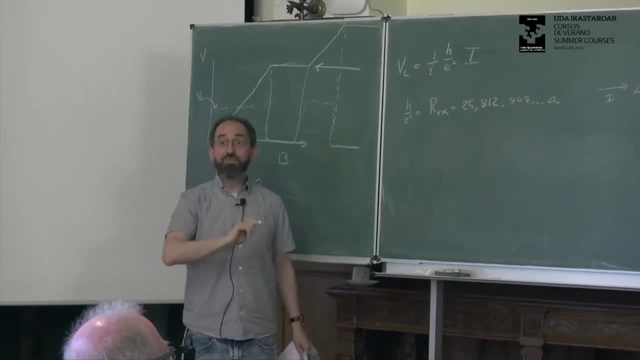 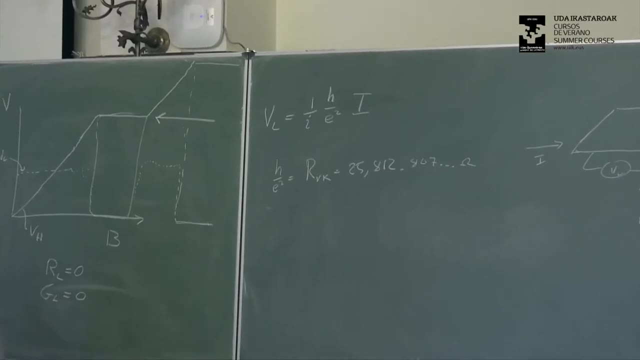 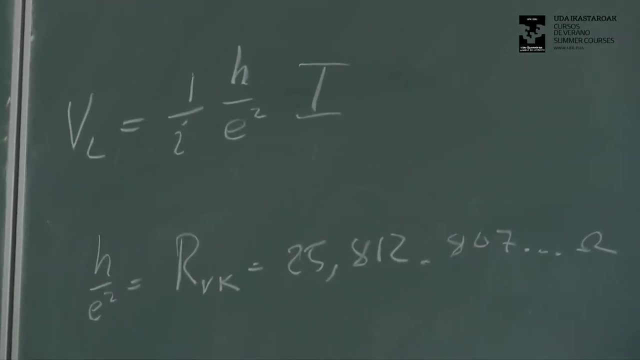 is exactly what h over e squared is. The statement which is non-trivial is that when you do this experiment, You measure exactly this number, and the precision with which this experiment has been done is about to 10 decimal points of accuracy. 10 or 11 decimal points of accuracy. 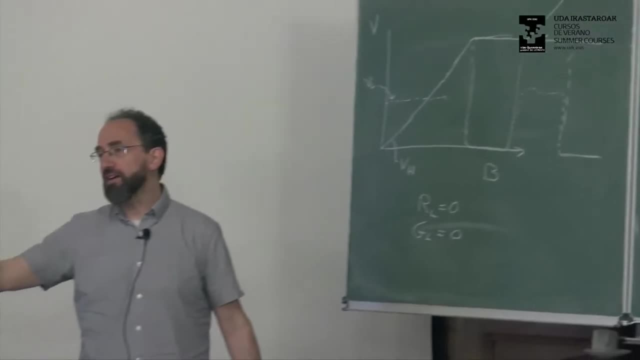 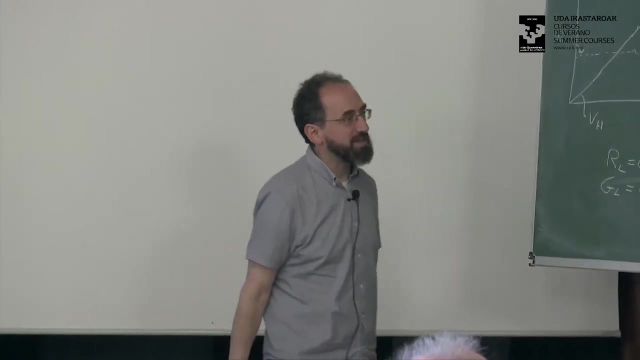 That's like measuring the distance from here to California to less than a millimeter. Okay, so it's a rather remarkable level of accuracy for an experiment where there's disorder in the experiment When you attach if you've. is anyone in the room an experimentalist? 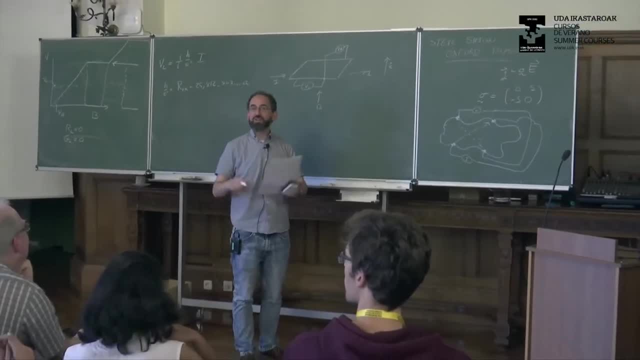 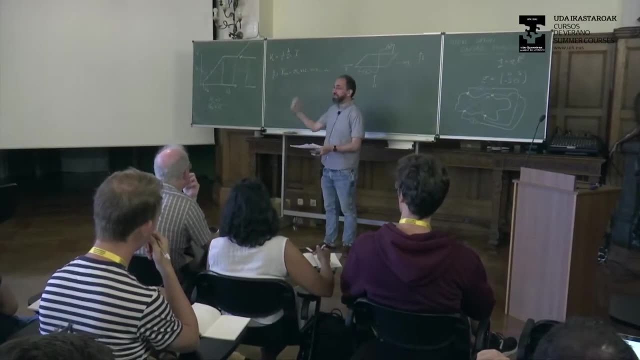 Oh, quite a few, okay, good. So you know how you attach contacts to your sample. you take a big blob of solder and you whack a contact onto it. So nonetheless, you attached a big blob of solder to your sample. there's disorder in. 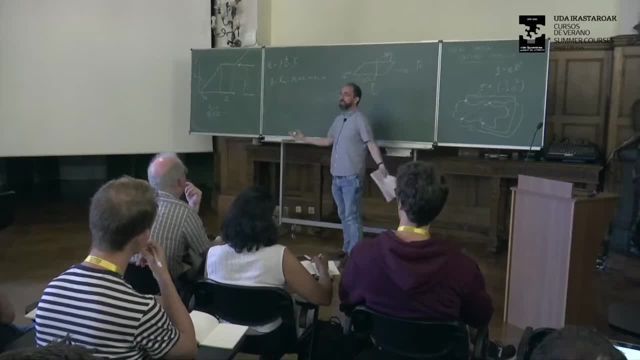 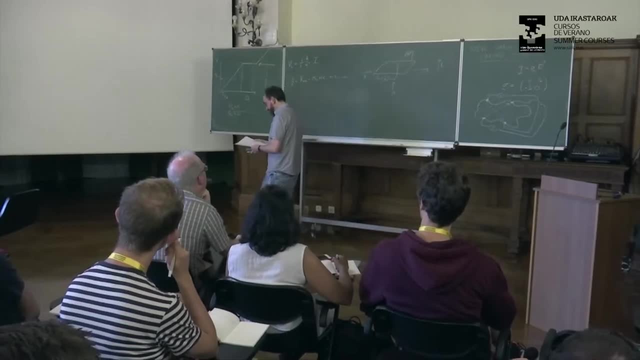 your sample. you don't know exactly where the magnetic field is. there's all sorts of effects that you might not have paid attention to, and nonetheless the experiment is reproducible to one part in 10 to the 10, or maybe even better. 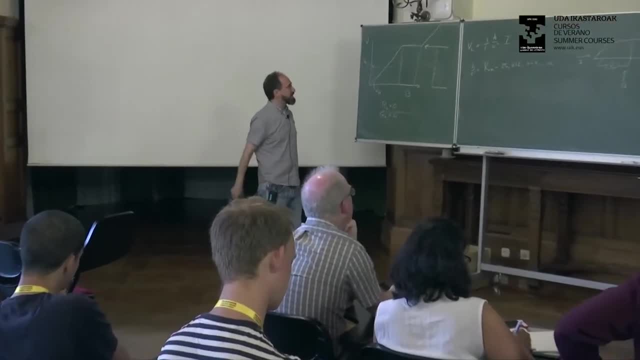 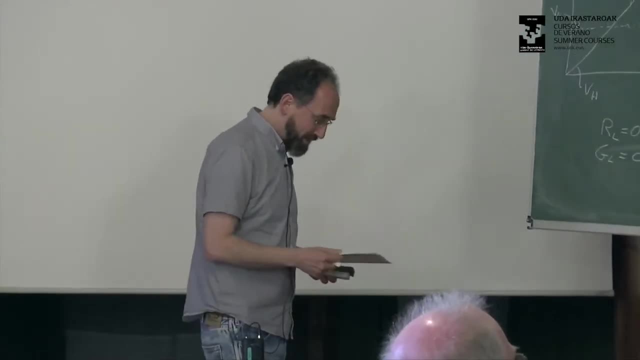 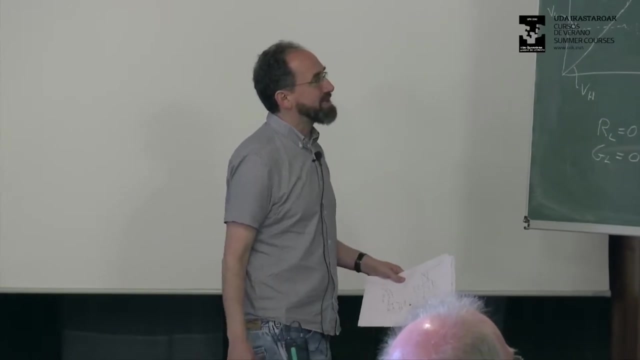 Okay, So we're going to want to explain this in some amount of detail. Von Klitzing won a Nobel Prize for discovery of this in 1985, about five years after he first made this measurement. One more comment about the basics of this experiment here that we might want to ask. 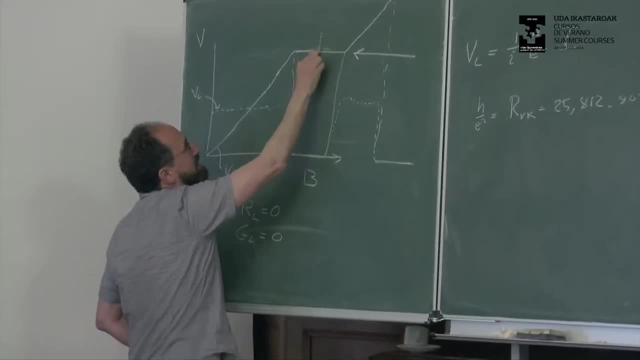 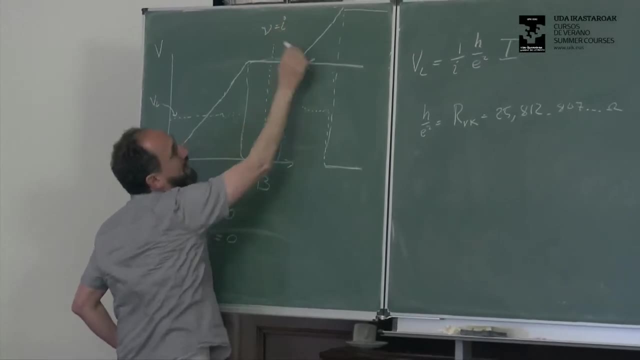 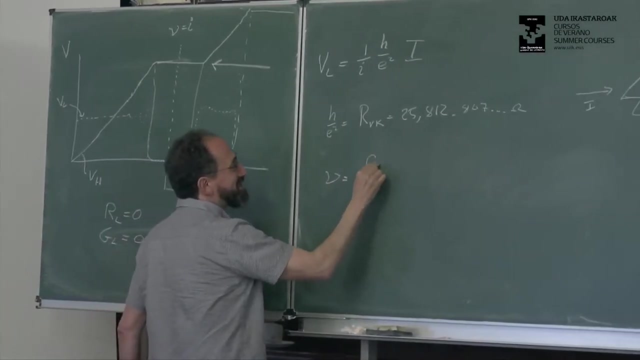 at what magnetic field does this plateau form? So at here We'll label this as nu. Nu equals I, this integer. I is the same integer that shows up over here, and this nu is known as what's nu, What's nu. 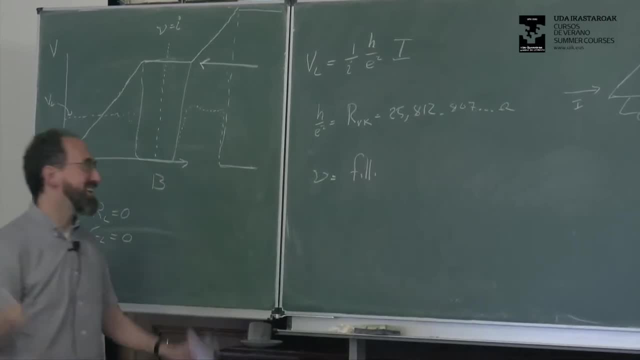 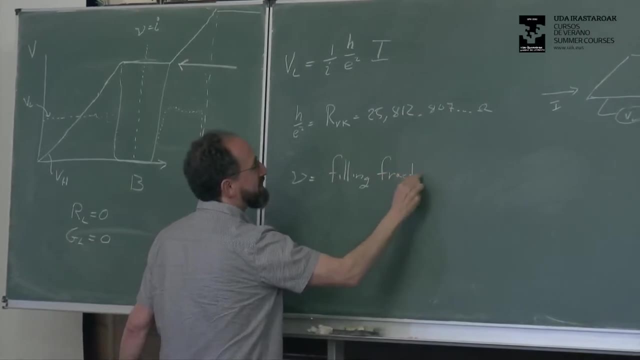 This is what's nu. Nu is, that was a joke. Did no one get that? God, I should not. I just give up on making jokes. right Is known as the filling fraction or the filling factor, which is well, we'll just define. 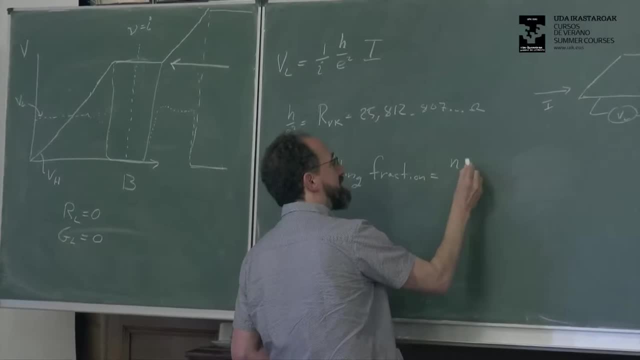 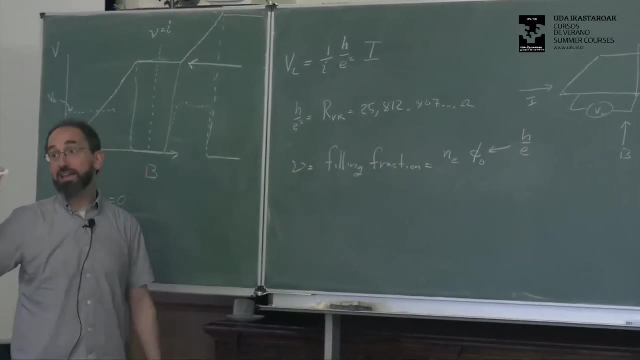 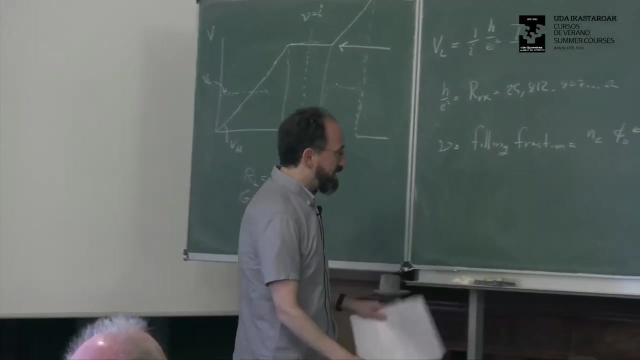 it this way now: It's the electron density times the flux quantum. The flux quantum is H over E. It's some again exactly defined fundamental constant. It's four point, something, something, something times 10 to the minus 15 Webers of magnetic. 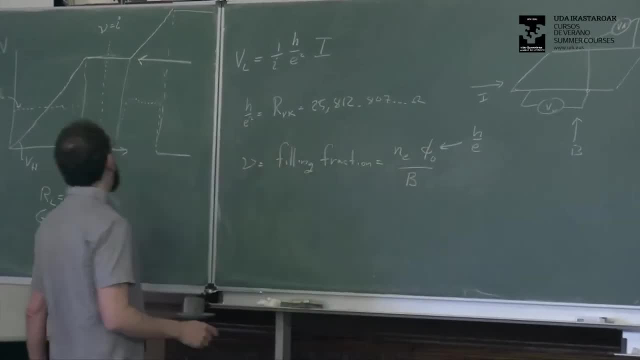 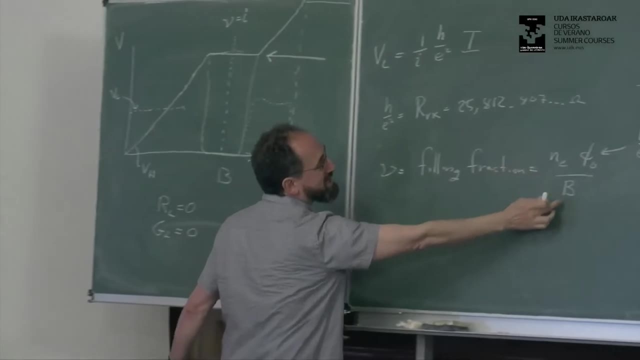 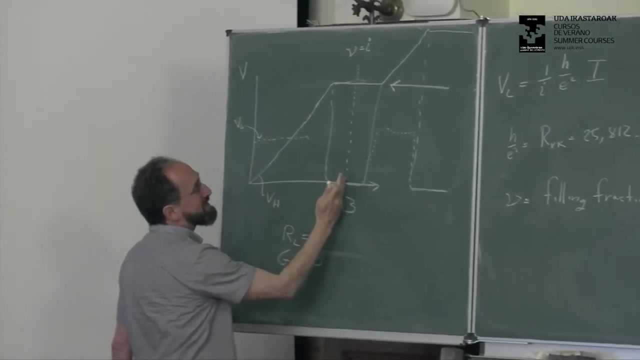 flux divided by the magnetic field, And the center of this plateau is roughly at the filling fraction at electron densities divided by magnetic fields. These are the things you can actually change in your experiment: the electron density and the magnetic field. So Who lines up with the center of the of the plateau? 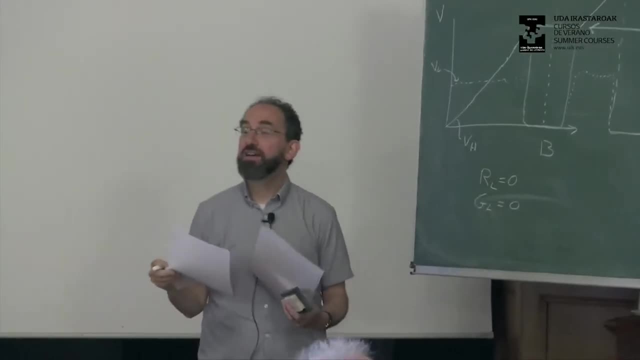 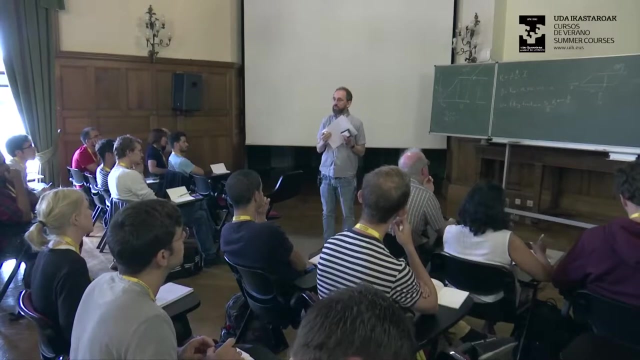 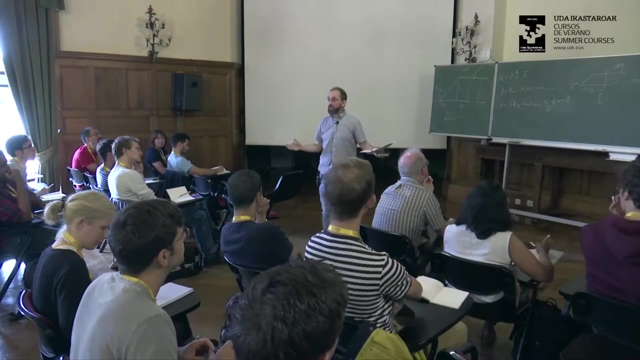 Everyone's still happy. Yes, Yes, So the width of the plateau is non-universal, It depends on the particular experiment. So it's actually it's a rather surprising result that in very dirty samples you have no plateau at all. 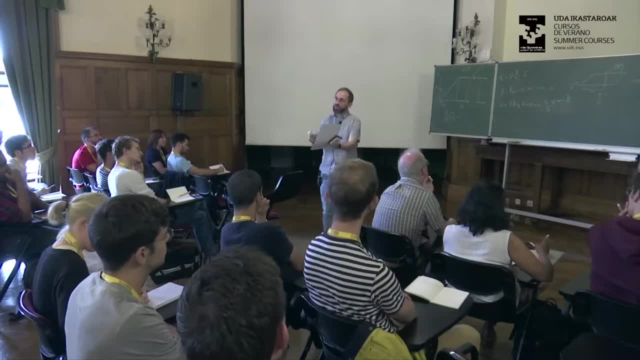 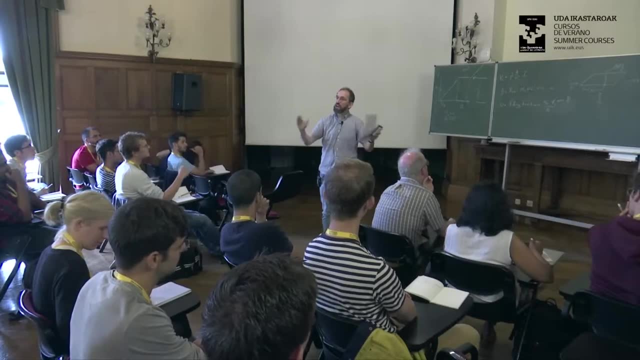 In sort of medium samples you have a medium plateau, and in sort of really good samples the plateau is still there, but it's very thin, So it's so. the width of the plateau is a complicated story, It's, and it depends a lot on the details of the sample. 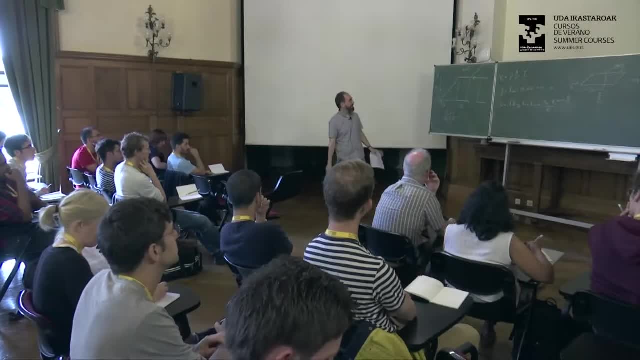 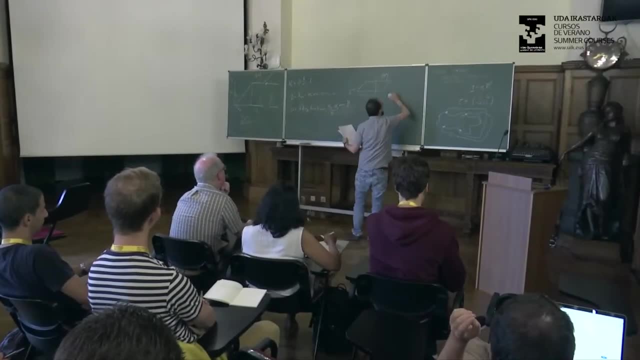 Okay, All right, So we're going to try to explain some of this, some of this physics, in some amount of detail And to begin, we will. um, I wish I had a bigger chalkboard here, but you know, we'll. 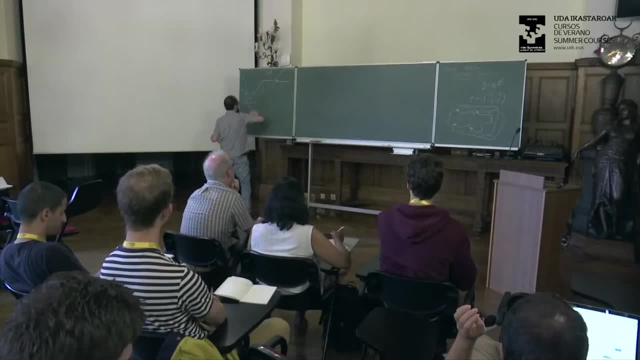 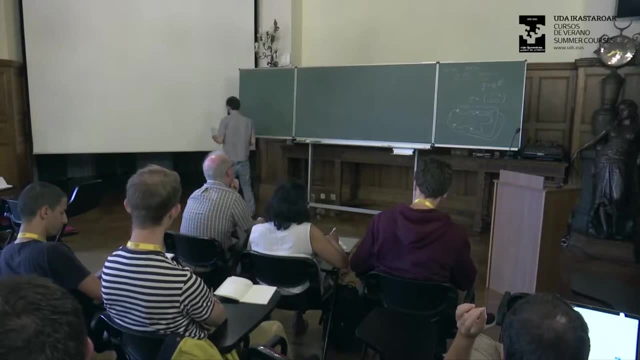 have to make do We're going to start with the single electron problem Of a single electron in a magnetic field, sometimes known as the Landau problem, um, because it was solved by Lev Landau in the early 1930s. 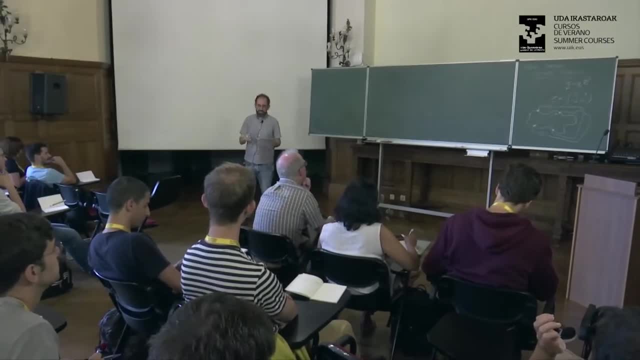 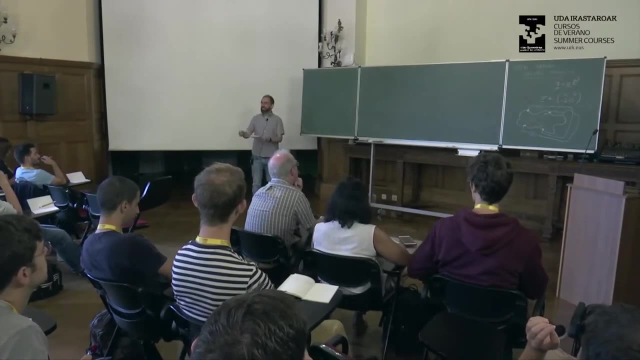 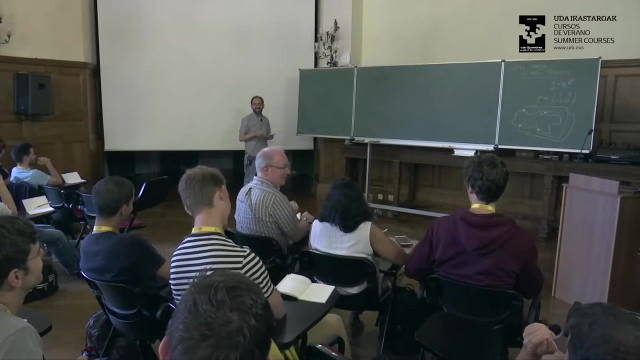 Uh, this was before Landau was sent to jail for criticizing Stalin. Um so just a important moral of this story is: if you live in a totalitarian dictatorship, do not criticize the person in charge. Um so, Landau, Landau, learned this really the hard way. 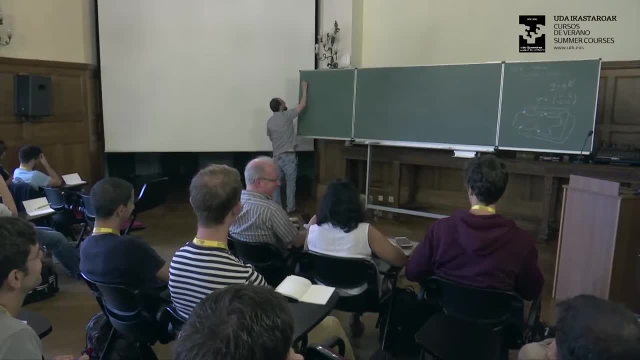 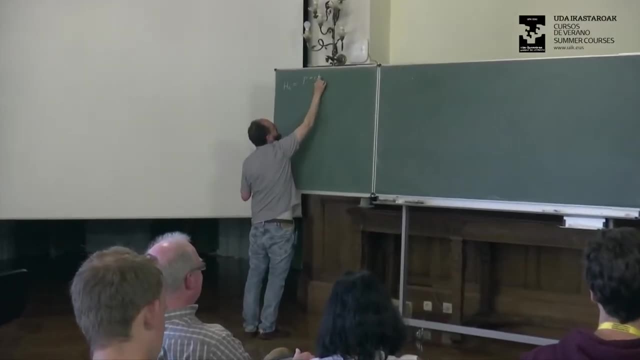 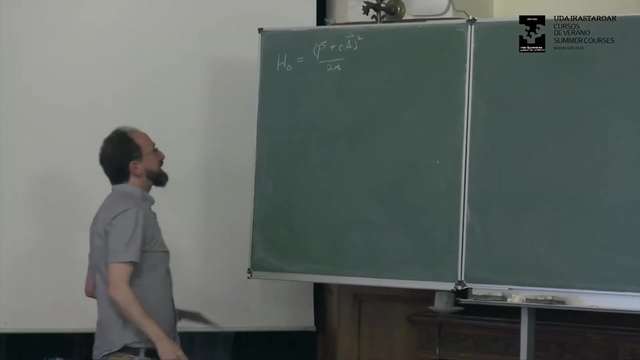 Um, okay, So an electron in a magnetic field, the Hamiltonian uh, P plus EA uh, squared over two M? Um. and we're going to ignore a lot of things in uh to make our life simple. 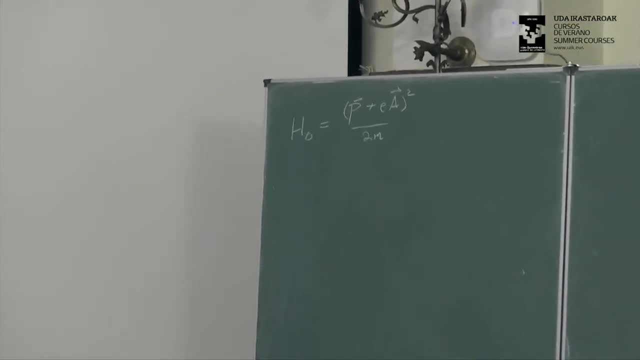 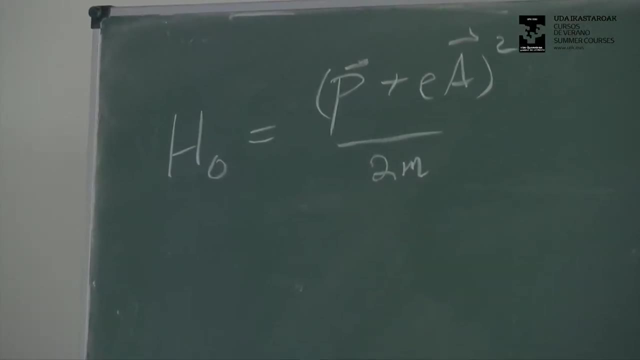 We're going to ignore the spin of the electron. We're going to ignore disorder. We're going to ignore spin orbit coupling, We're going to ignore phonons. Lots of things Just throwing out just to make our life simple at this point. 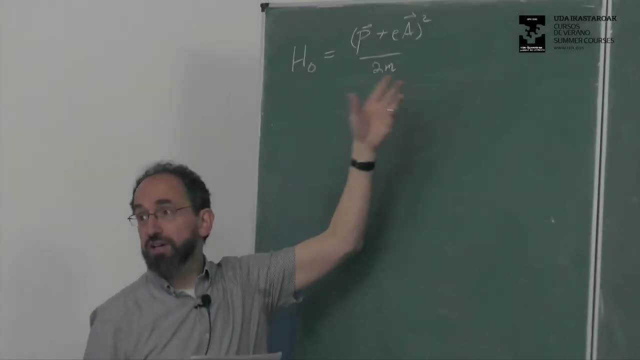 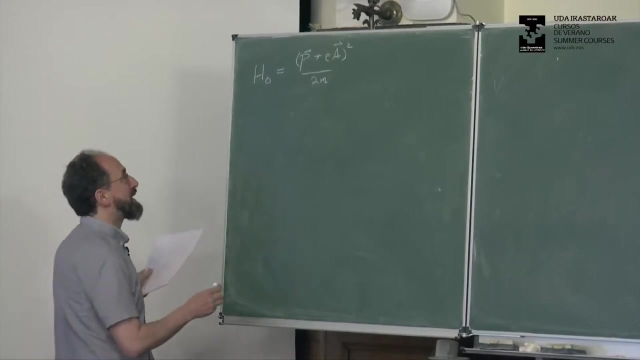 In order to describe an electron in a magnetic field, we have to choose a gauge for our vector potential, A Um. there's many different gauges we can work with Um. the simplest is probably so-called Landau gauge, where the vector potential is um. 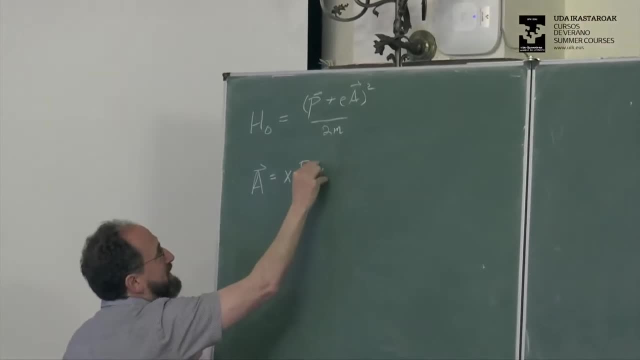 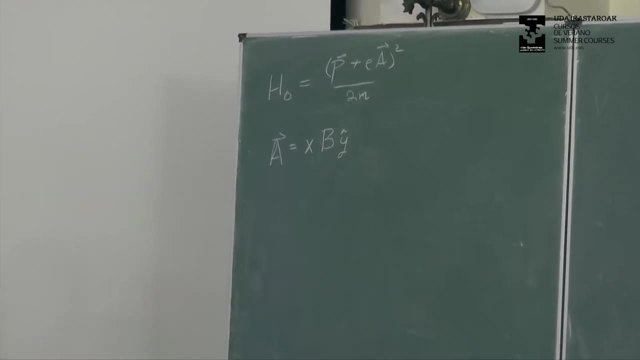 X times the magnetic field, B in the Y direction. So our plane is in the XY, the XY plane. So it has a value X times B. It has a value Y in the Y direction And this is convenient because it's translation invariant in one direction, in in the Y direction. 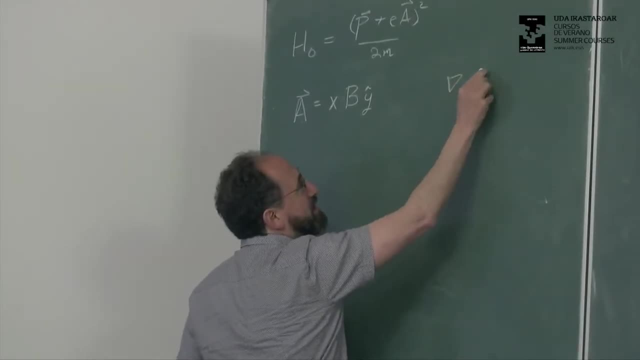 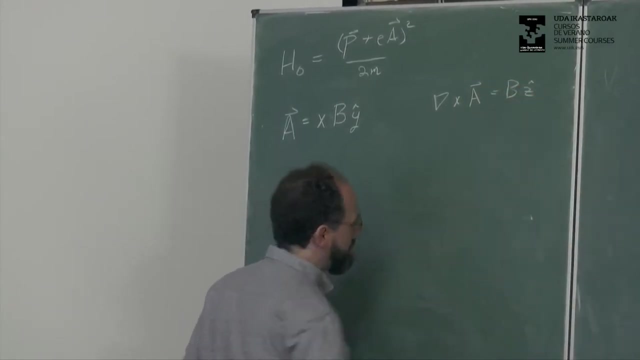 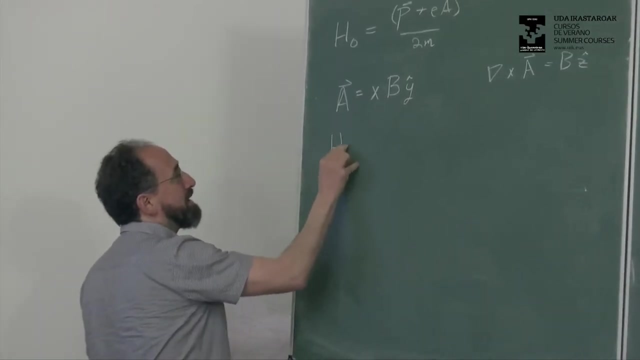 Um, you can check, uh, very easily, that the curl of A gives you the magnetic field B pointing in the Z direction, which is what we want, And we can then plug this into our, our Hamiltonian to get. our Hamiltonian is then one over two. 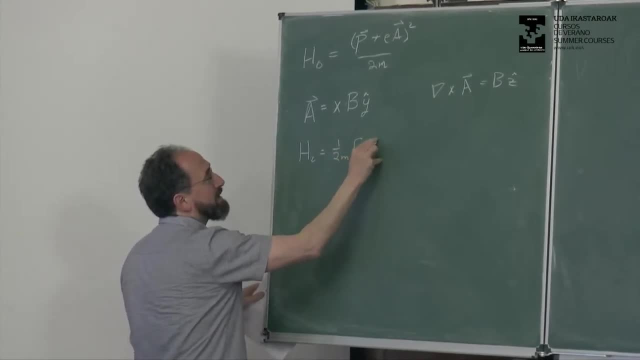 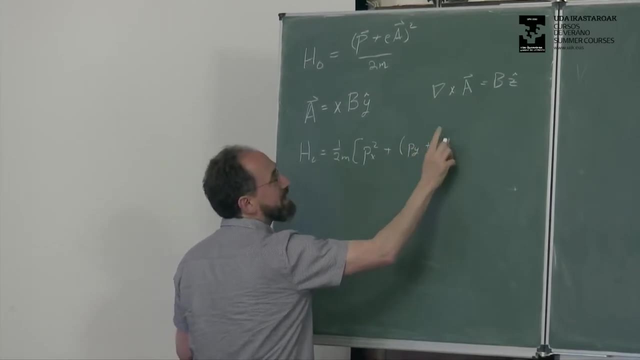 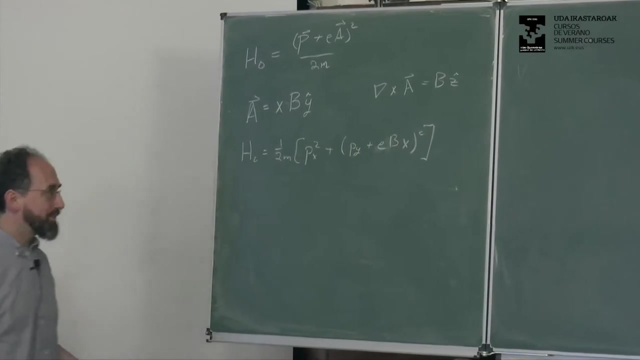 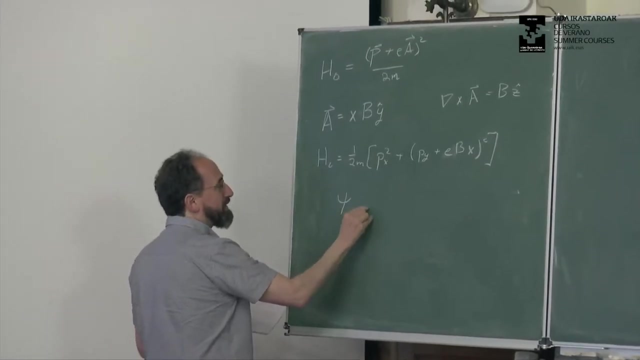 M um, P plus P, P, X squared plus um P, Y plus, I guess E, E, B, X squared like that Um. since the system is now translationally invariant in the Y direction, we can write the wave function has to be some function of X only. 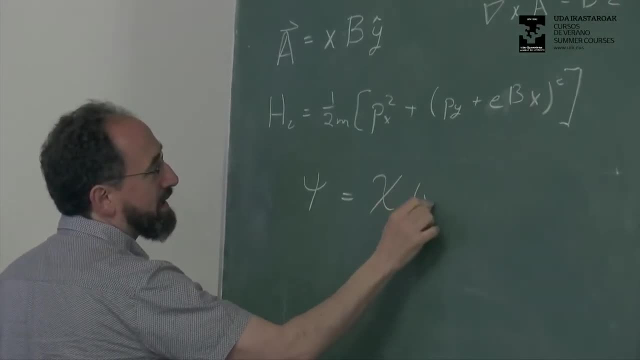 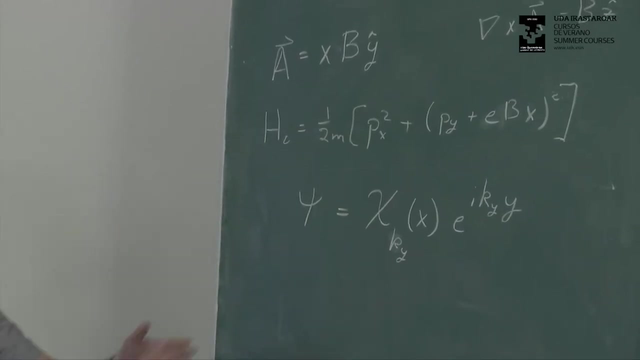 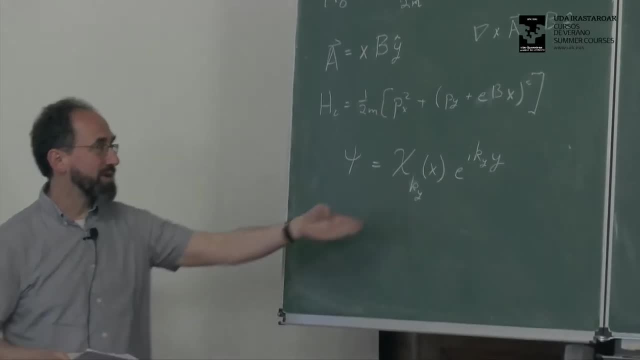 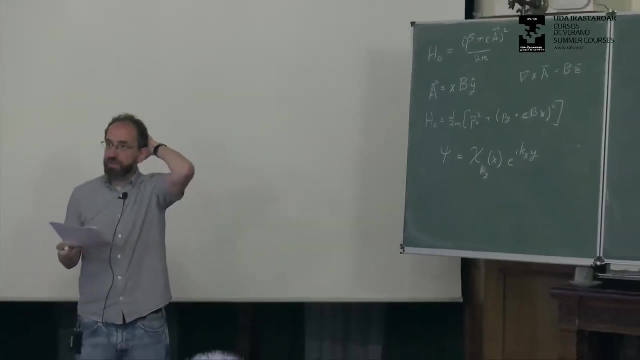 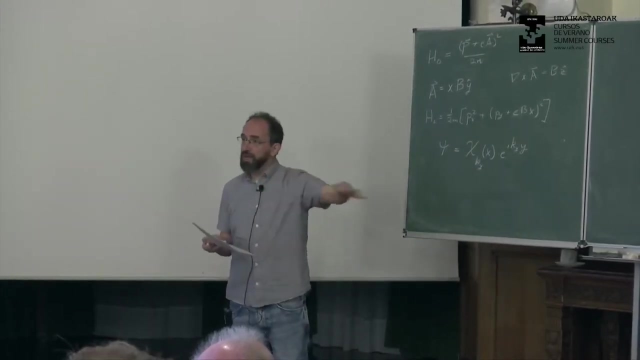 of Hamiltonian series based on a Hamiltonian frame set. Um, so this is just the circle of Hamiltonians. Um. again, there's instantly a function discussion. So we got to consider buying people adds up a little bit of the excோtion. weğin the distance between Hamiltonian space bars and Hamiltonian importance here. 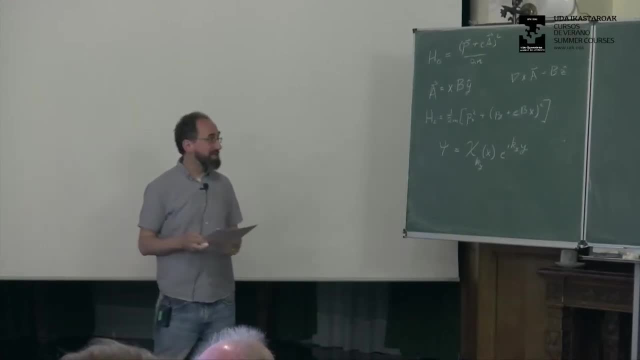 But that makes sense, I'm gonna, I'm gonna- and here's aplayin the function. I want to make sure I've got some of these oct ye potential and you have some function of the position in the unit cell times. a plane wave. 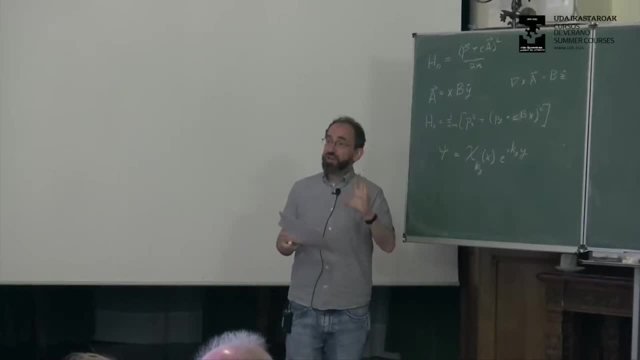 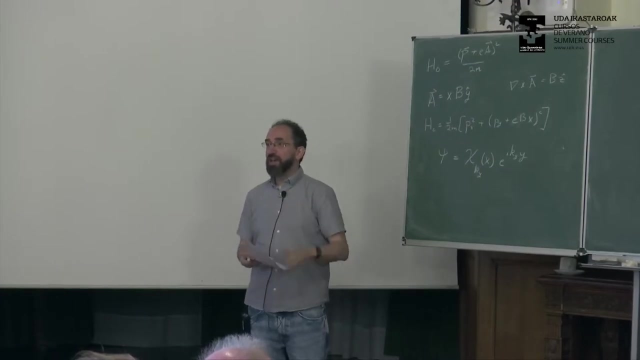 in both directions. you actually can translate the quantum Hall problem to exactly what Charlie was talking about. You make a unit cell with an integer number of flux quanta in it and work in a gauge which is periodic in that unit cell. This can be done but it's a lot more complicated and 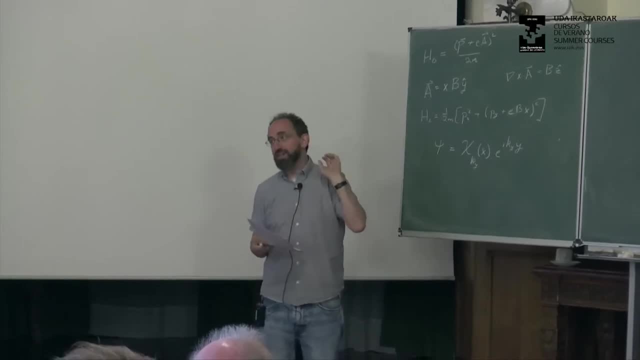 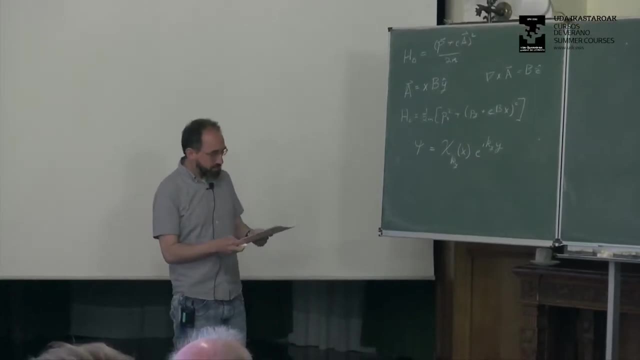 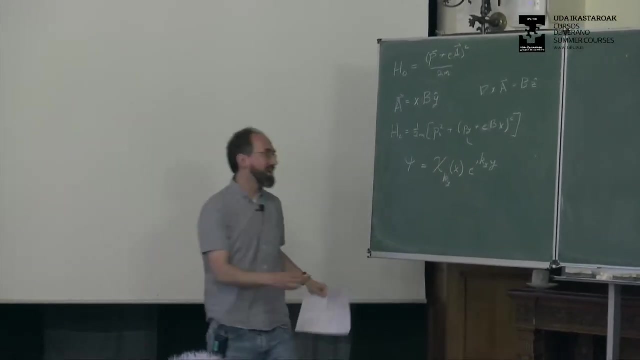 our life is going to be a lot easier if we do it this way. But if we did it that way it would look a lot more like what Charlie was talking about. but we're not going to do that, Okay, All right. So any questions on where we are so far? Good, Okay, So p? y here is minus i h. 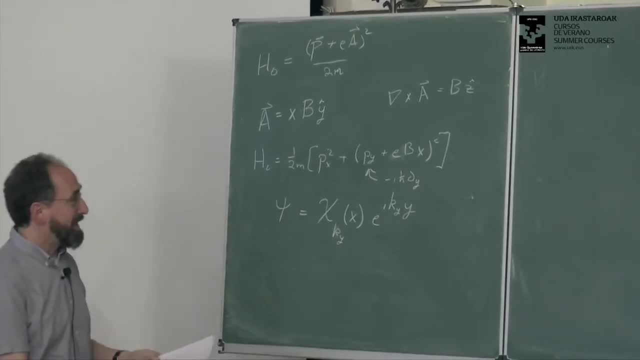 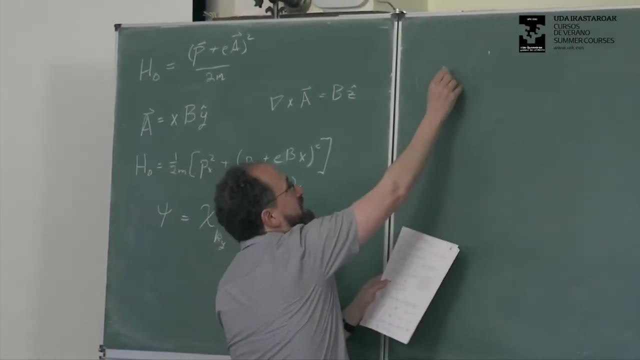 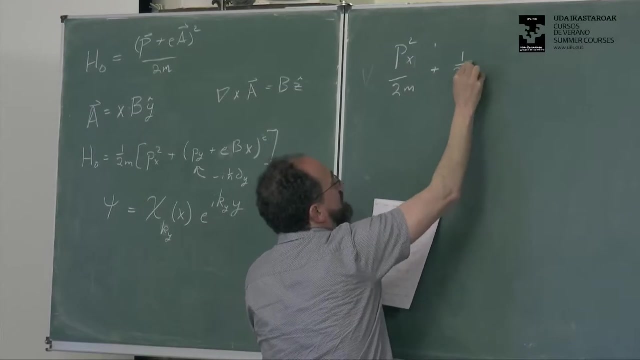 bar derivative in the y direction. and then we plug this wave function into this Hamiltonian and we rewrite our Schrodinger equation in the following form: So it then becomes p x squared over 2 m plus. I'm going to define a couple of constants here which are sort of 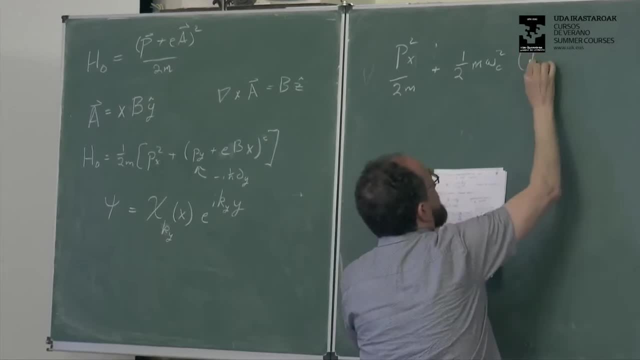 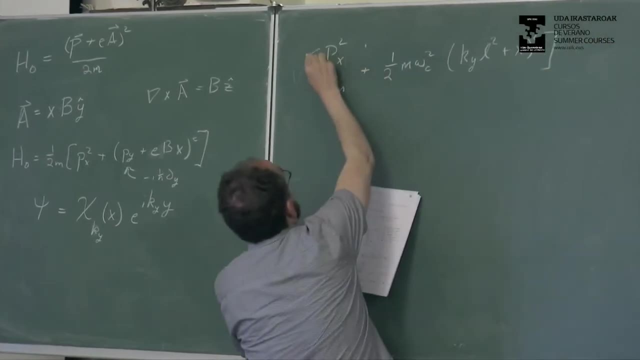 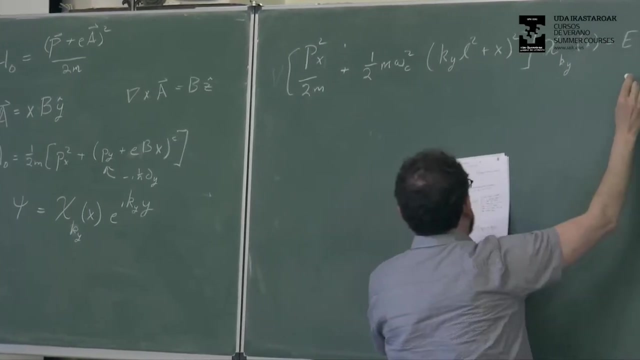 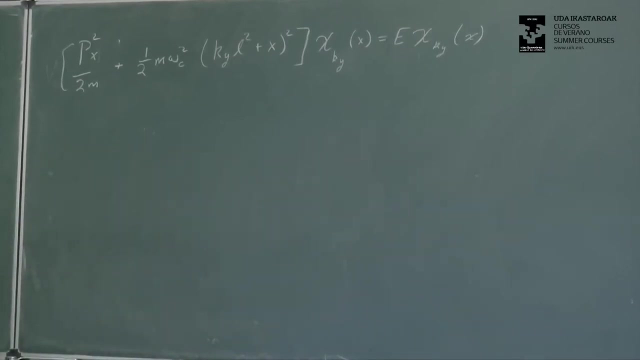 useful constants to know about. k y, l squared plus x squared, this on the function k chi sub k y in the x direction equals e times chi sub k y in the x direction. So for each value of k? y we choose we get a different one-dimensional Schrodinger equation. So we reduced our 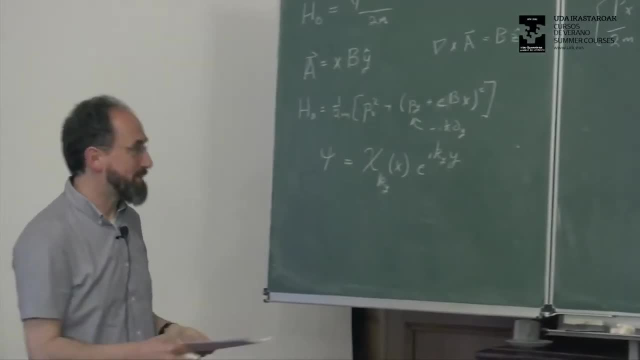 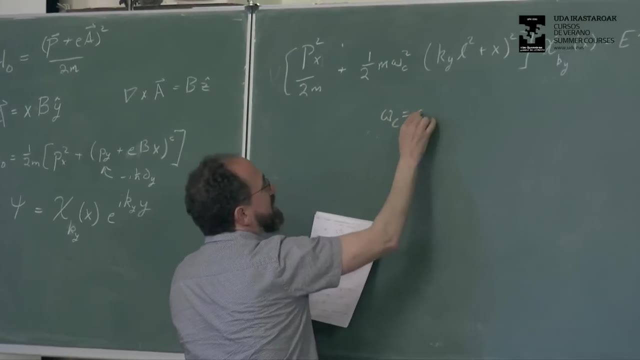 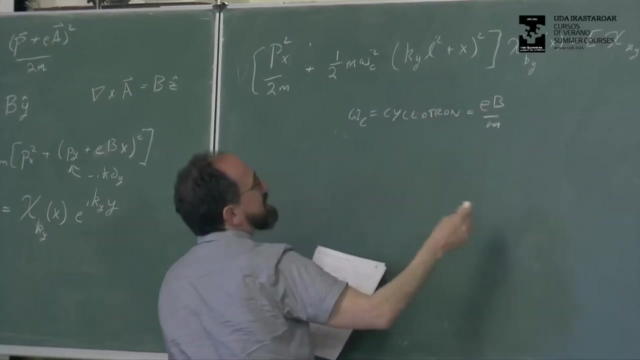 two-dimensional problem to a one-dimensional Schrodinger equation. Okay, And if you look at it a little bit harder, oh, I didn't give you what these, what these constants were. So omega c is known as the cyclotron frequency cyclotron, which is just e, b over m, And the other constant I. 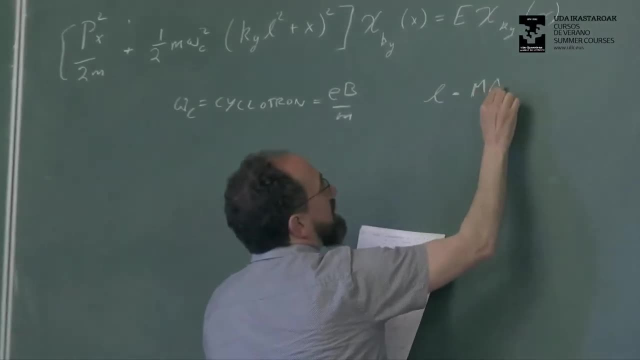 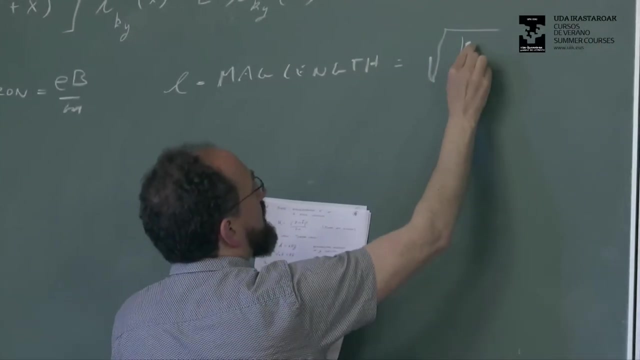 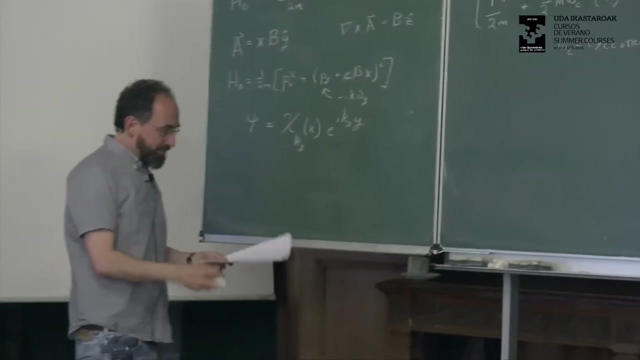 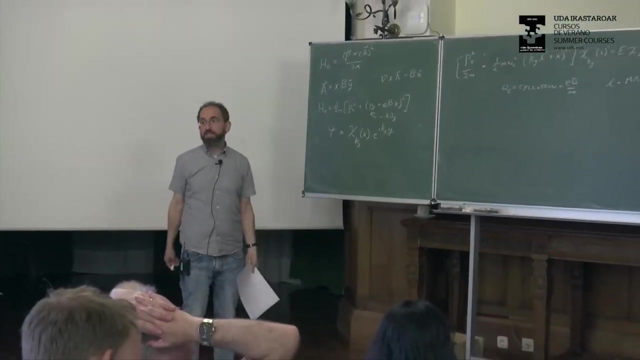 defined is l, the so-called magnetic length, mag length, Um, which is square root of um, h, bar over e, b, Okay, Um, all right, And we can look at this equation a little bit more carefully And what we realize is that it's just a harmonic oscillator. 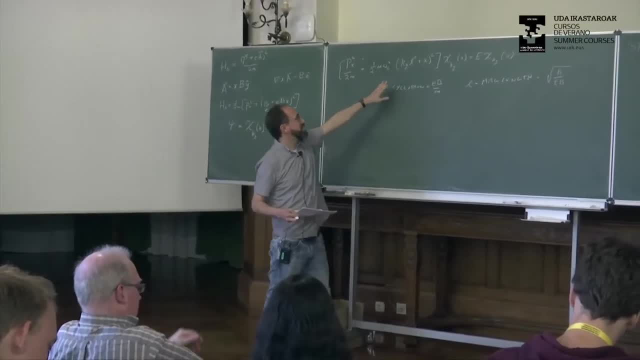 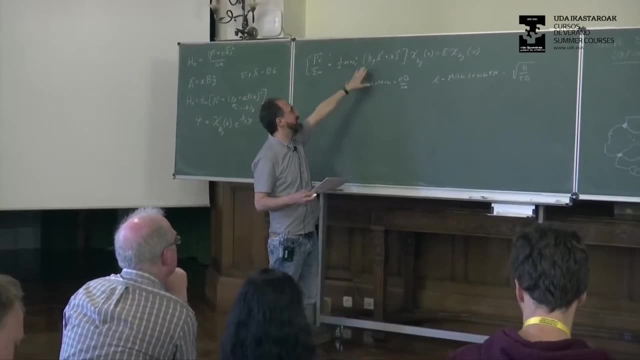 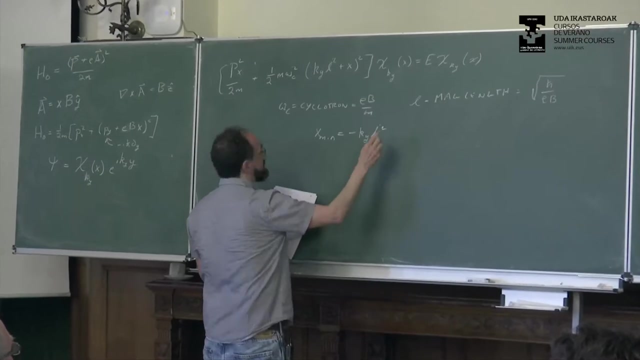 So it's. this is the kinetic term, This is a quadratic term. It's just that x has been shifted by a constant, So it's a harmonic oscillator where the minimum of the harmonic potential is at position uh, x min is minus k, y, l squared, l squared like this. Okay, So we know what the 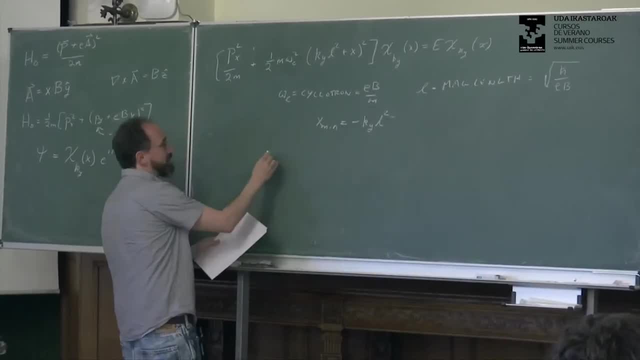 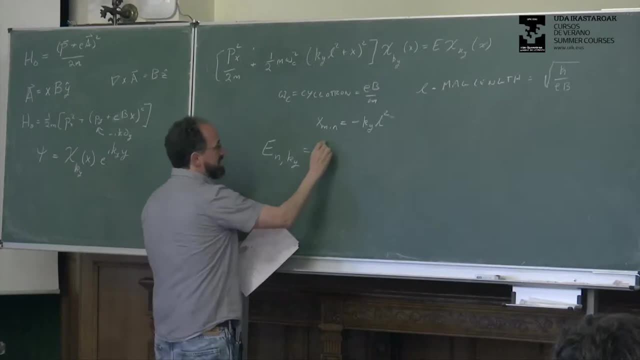 solutions of this uh harmonic oscillator equation will be The energy, the nth energy at um given k y is h bar cyclotron frequency, n plus one half. Okay, So we have a discrete energy uh set of energy levels which are independent of the momentum in the k y direction, um and. 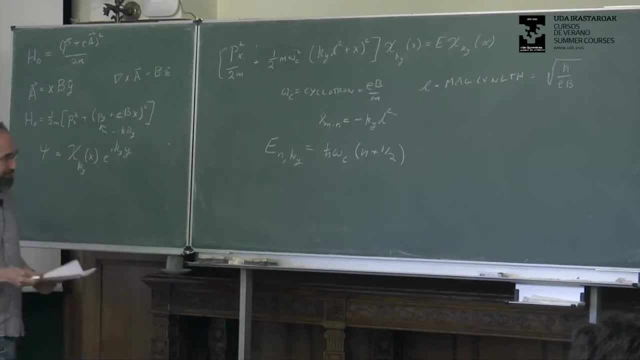 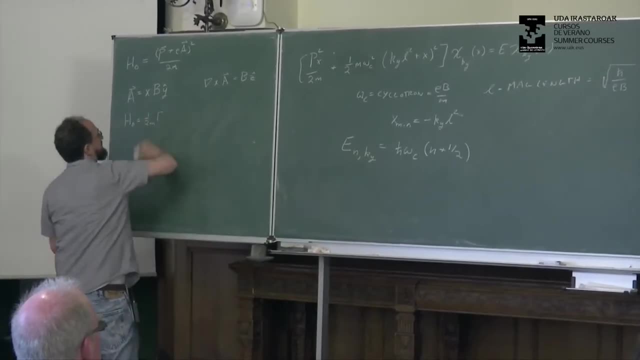 depend only on this index, on this index n. So what do these eigenstates look like? Let's erase this here. Um, the eigenstates, um, let's try to draw it in in two dimensions here. So we have: 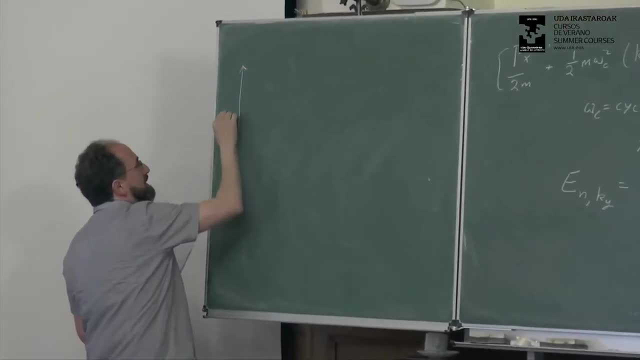 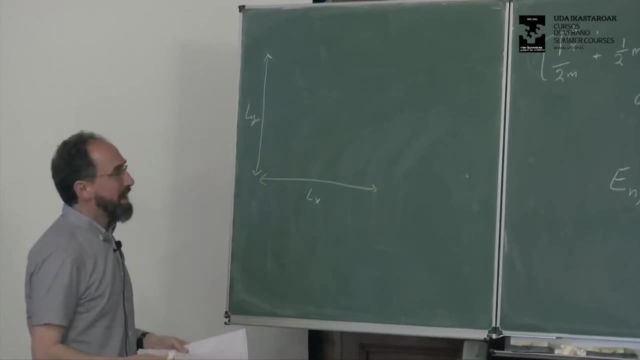 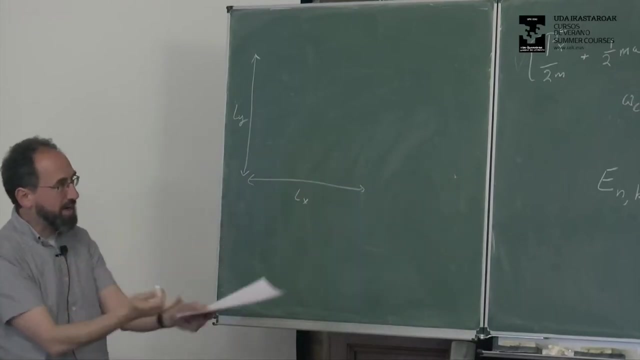 uh, some system, uh, with size l y in the y direction and size l x in the x direction, And the um position in the x direction will be. you know, we should think of it as being a harmonic, well positioned around the position, you know, centered around the. 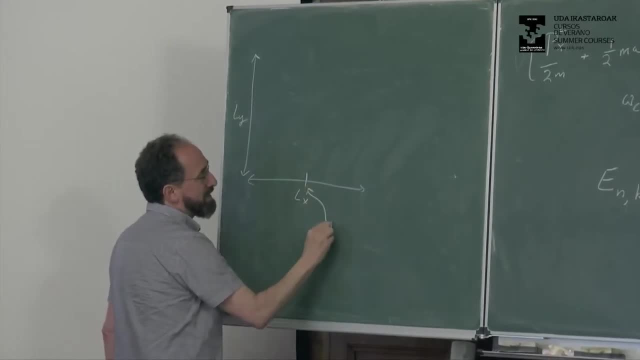 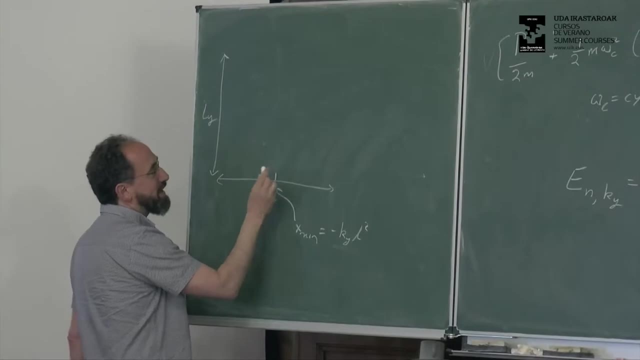 position of here, which is the minimum of that potential. well, is at minus k y l squared. And so if we take the lowest harmonic oscillator state, that's a Gaussian like this, and then it propagates in this direction. it goes as: 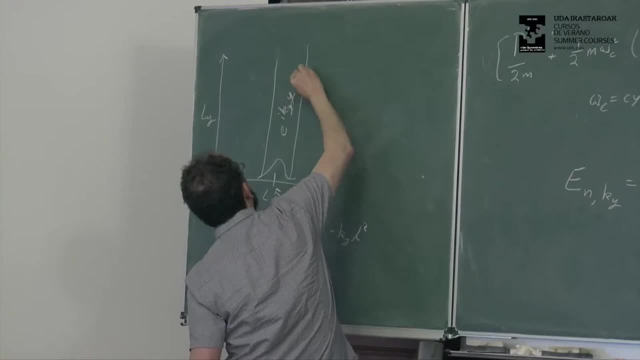 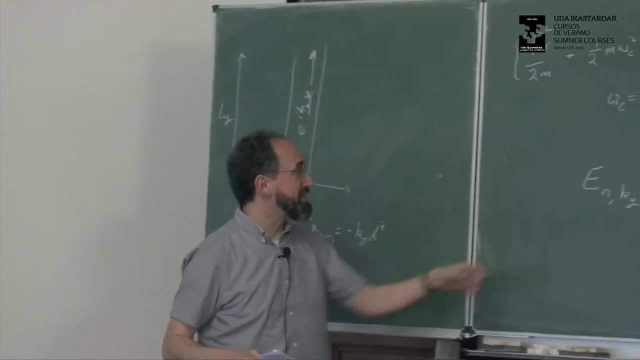 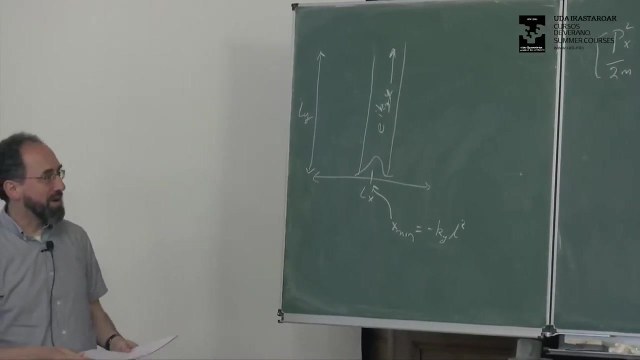 uh e to the i k y, y is a plane wave in that direction And then it's a harmonic state in this direction And the higher um higher eigenstates look like not Gaussians but but more weakly Gaussians, like the higher harmonic oscillator particle in a um harmonic well state. Okay. 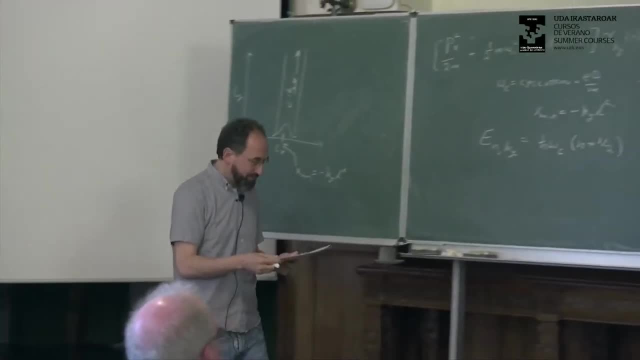 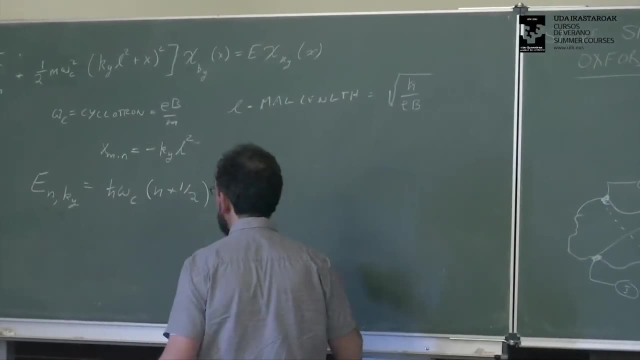 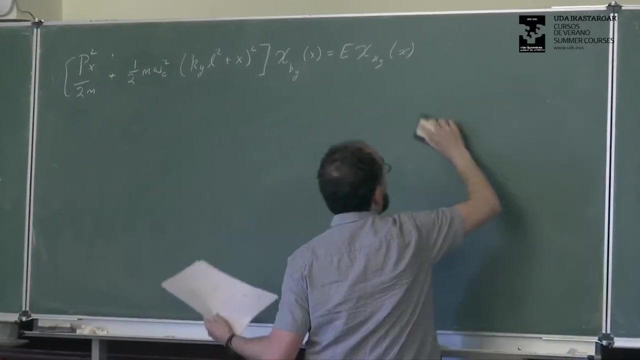 Everyone's still happy with this. Okay, good. Um so our- uh, I keep having to erase what I just wrote, but to live with it. Um so, we, we can write our. okay, we can write our. 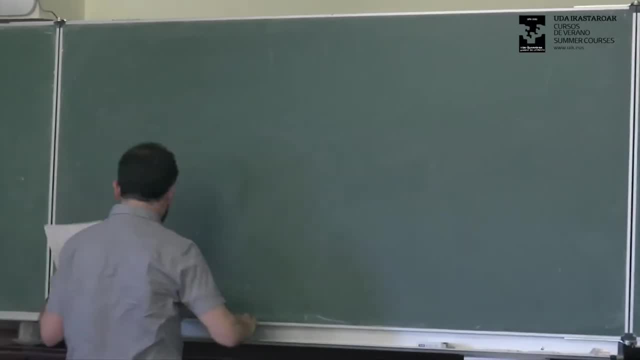 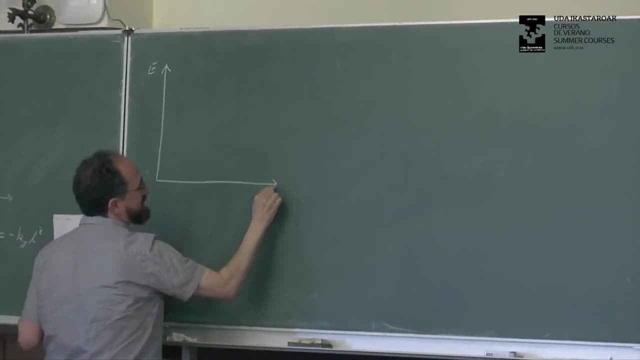 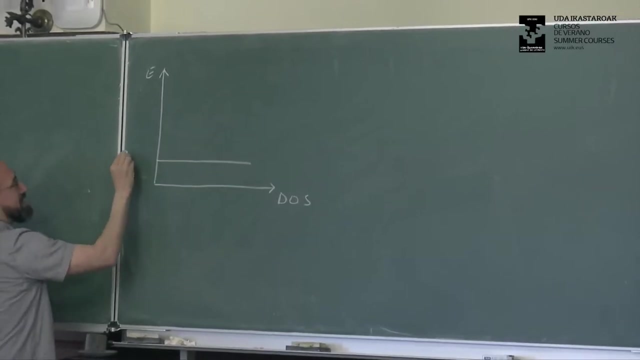 um, density of states as a function of energy. Uh, uh, sorry, Yep. So here's energy over here, energy going up, and then we have density of states, like this density of states, and then there's a big spike, a whole bunch of of states at energy, half h bar omega c. 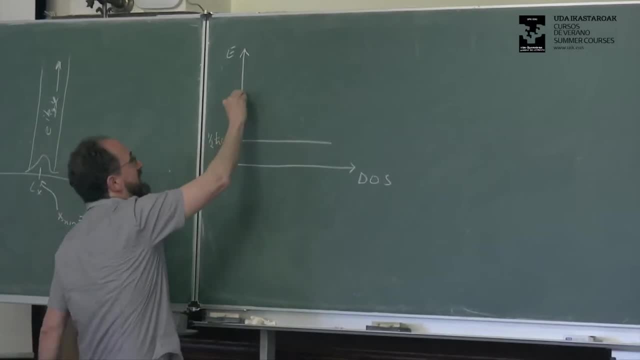 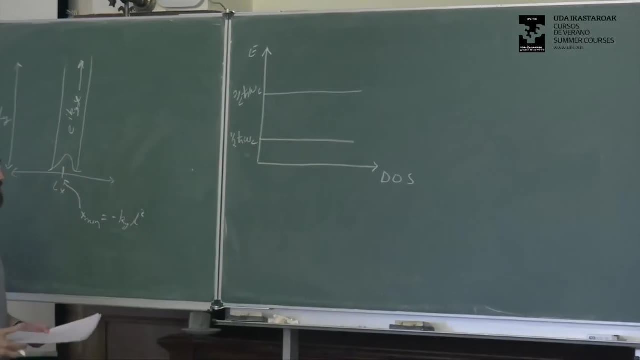 it's the lowest harmonic oscillator state, And then the next lowest harmonic oscillator state is at three halves h bar omega c, And at each um. at each harmonic oscillator uh energy level. you have a whole bunch of states corresponding to the different. 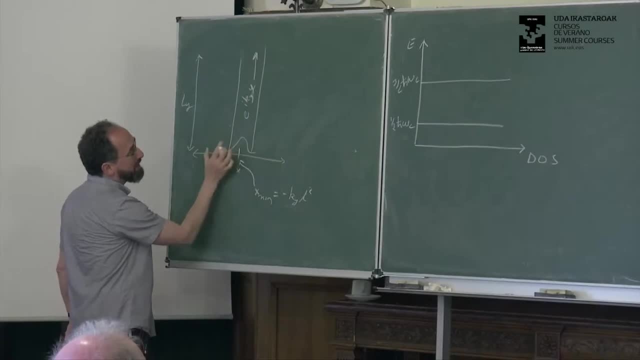 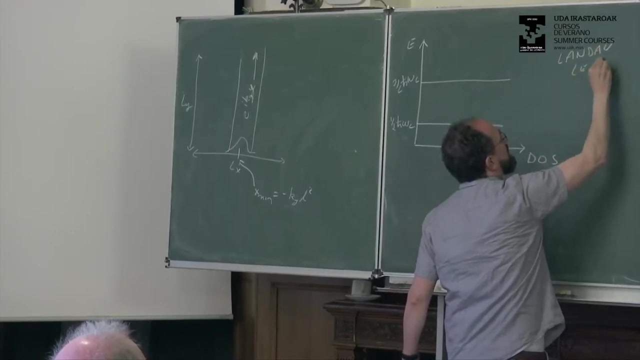 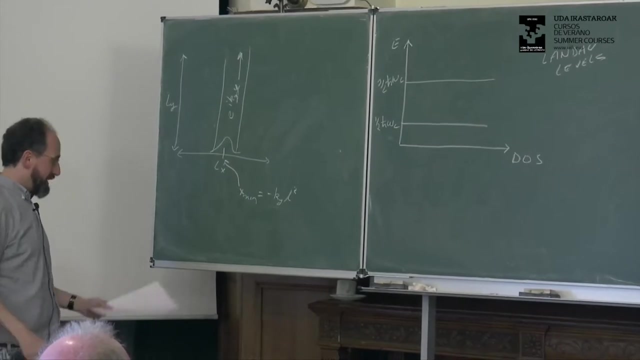 possible values of k, y, which move the minimum of the well uh to a different position in in x. Okay, So these levels are known as Landau levels, after I love Landau, Landau levels, Um, and it's important to try to try to figure out how many states are there in a a given Landau level. 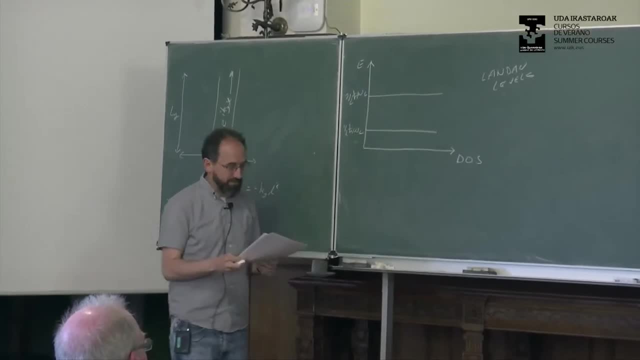 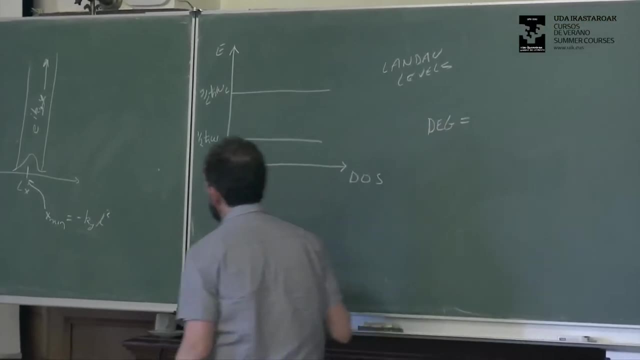 What's the degeneracy of one of these sets of of eigenstates? So let's try to figure that out. So the degeneracy is equal to, um, well, the the length of your system in the x direction. 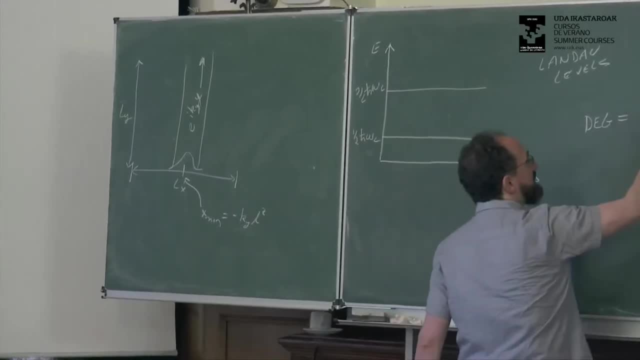 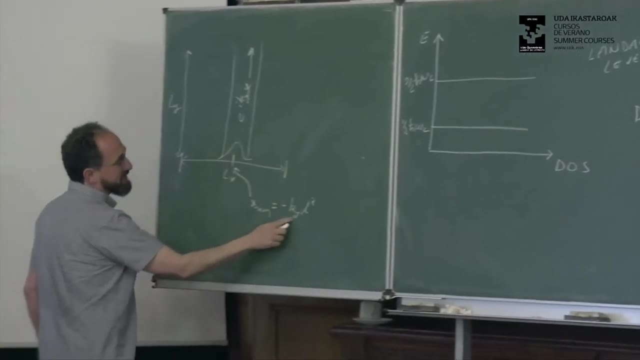 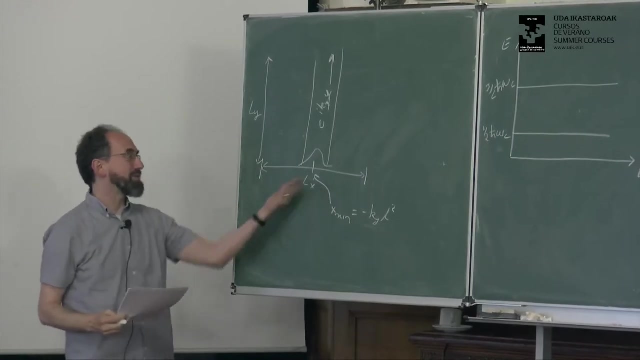 divided by the spacing um in x between adjacent eigenstates. Because as we change, uh, as we change k? y, this moves over a little bit. change k? y some more, it moves over a little bit, and so forth. And so all we need to to count up all the states. 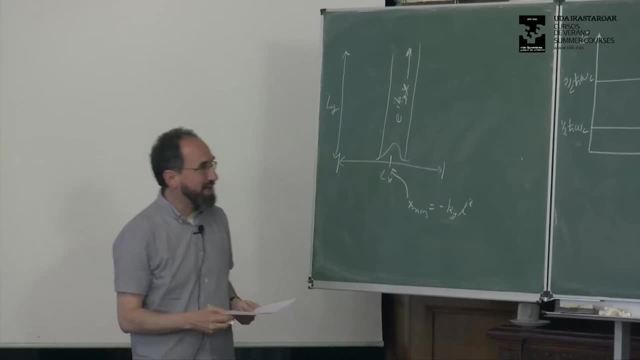 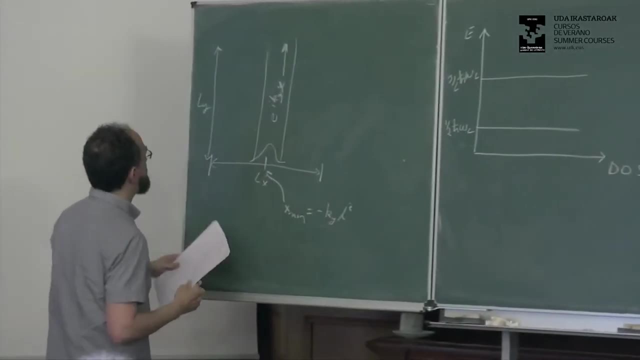 we just have the length in the x direction divided by the spacing. So what is the spacing? Well, as we usually have in uh, quantum mechanics, we're going to well in solid state. what we usually do is we take. 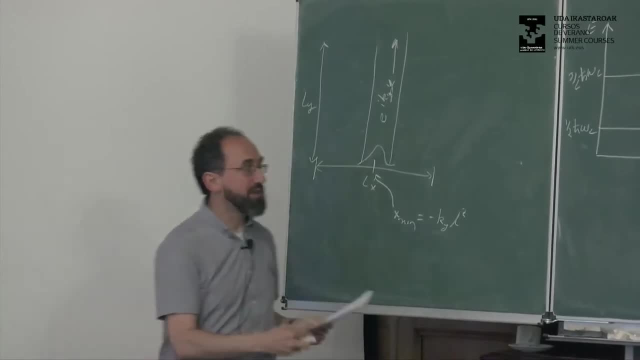 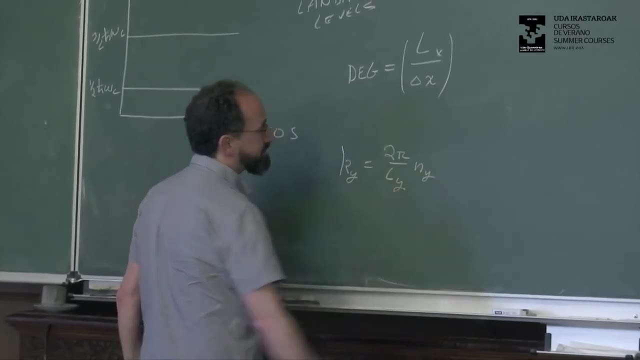 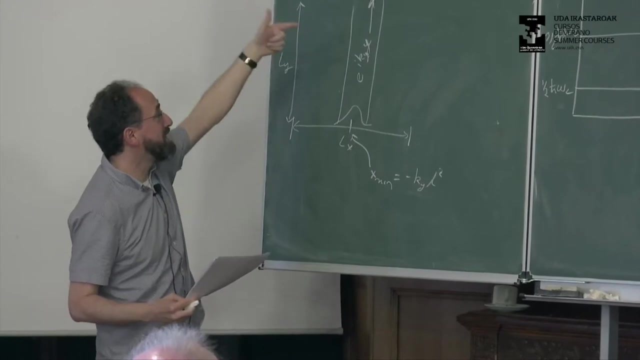 the distance in the y direction to be periodic, so that k? y becomes quantized as 2 pi over ly times an integer. That's so that the plane wave going this direction has to bite its own tail when it comes back to itself. So we're really thinking about something that's a cylinder that wraps around in in this direction. 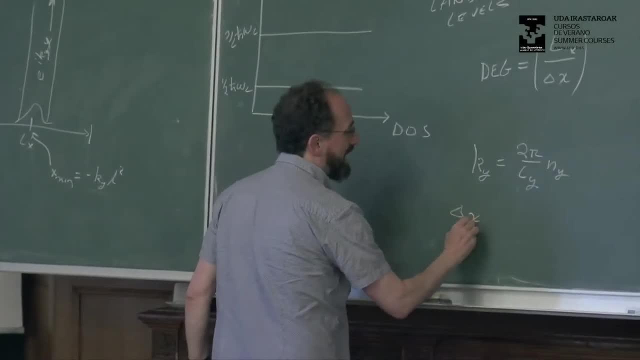 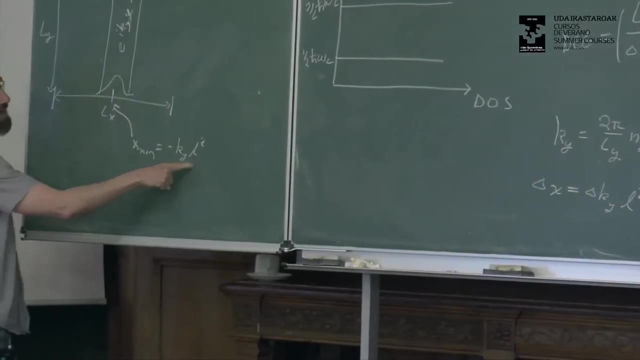 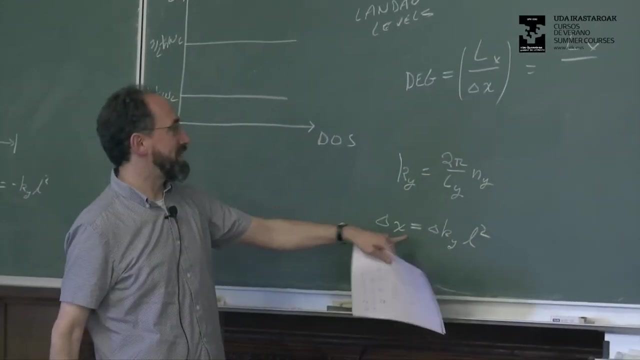 So the spacing delta x is delta k, y times l squared, because x is related to ky by a factor of l squared, So the degeneracy is then lx over the spacing of x. delta ky is 2 pi over ly, then times l squared. 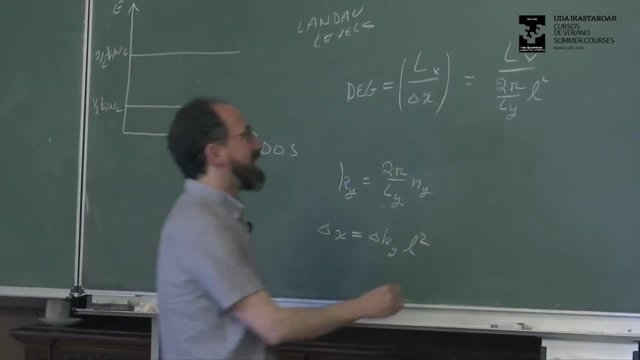 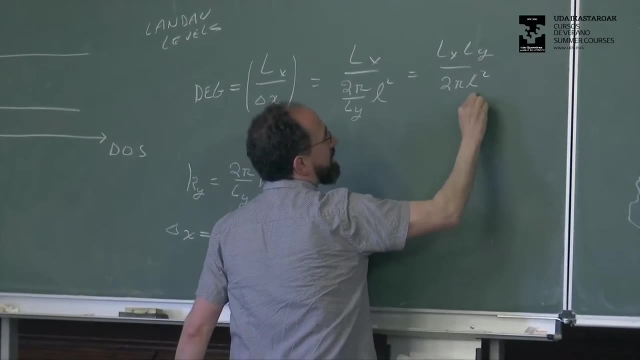 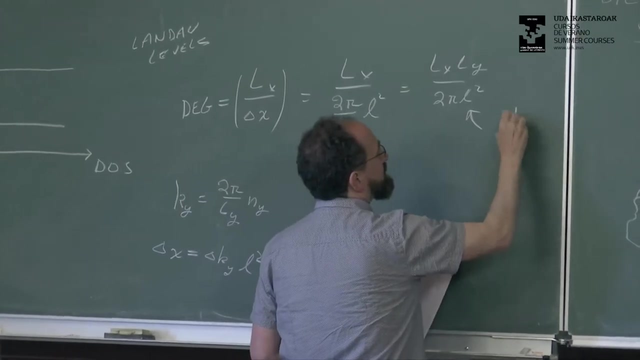 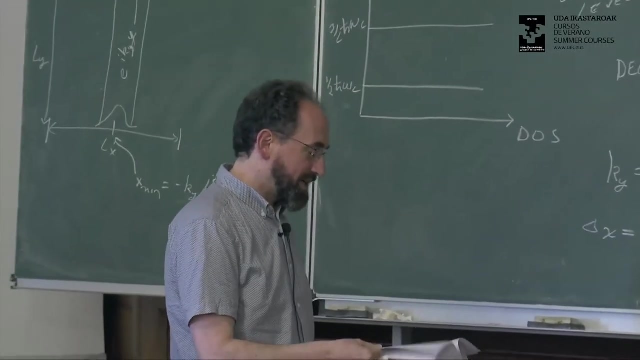 I didn't mess that up. And then we can simplify this to lx times: ly over 2 pi l squared. l squared was l squared. is h bar over ev or was it h? Problem with erasing what you just wrote? No, it's h bar is correct like it is. 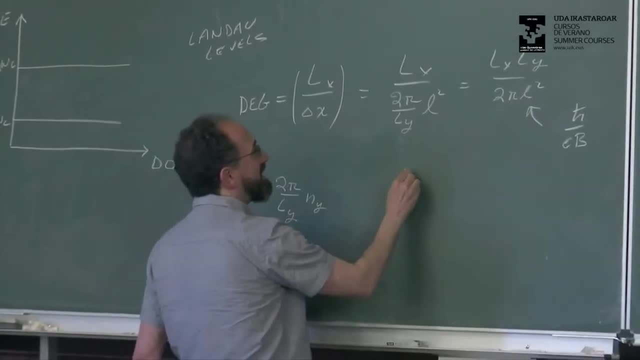 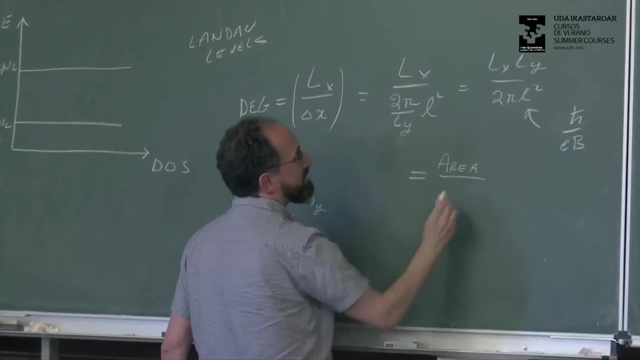 Oh, because there's 2 pi right, So that makes it h, Thank you. So the degeneracy is in the area of the system and divided by magnetic field, and then there's a factor oops area in the system times magnetic field. sorry, 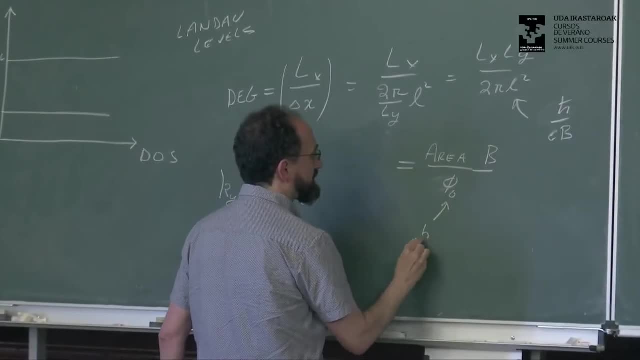 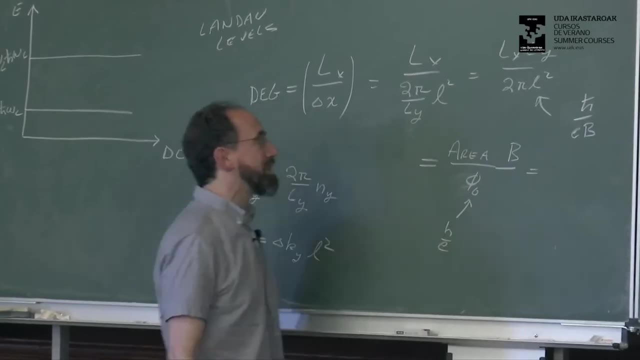 divided by a factor of phi naught, and phi naught is the h over e factor and we recognize this as the area of the system times. the magnetic field is the total magnetic flux penetrating through the system divided by the flux quantum. So this is flux. 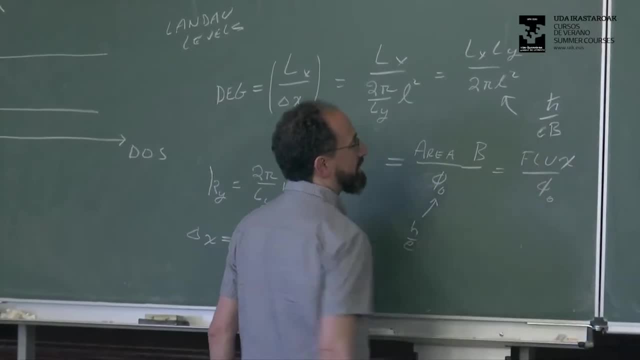 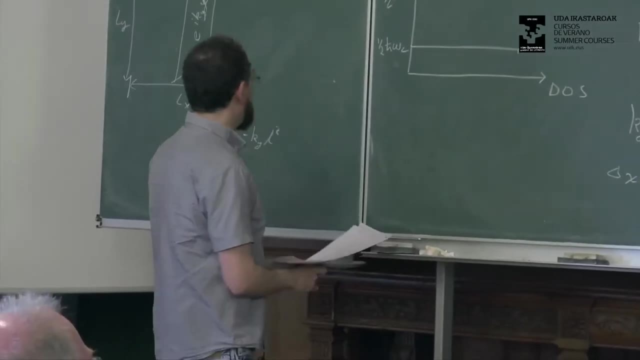 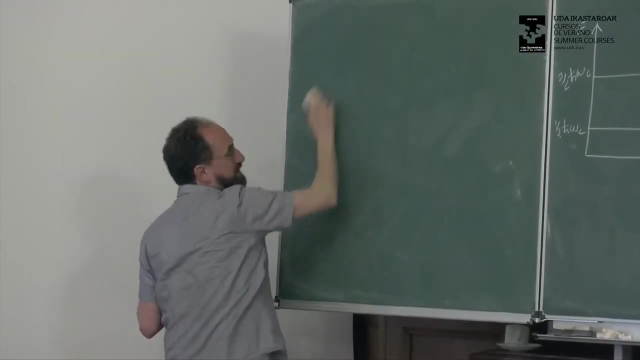 total flux divided by the flux quantum. Okay, that gives you the total degeneracy. Okay, that gives you the total degeneracy of each of these of these Landau levels. So this brings us back to one of the things I defined earlier. 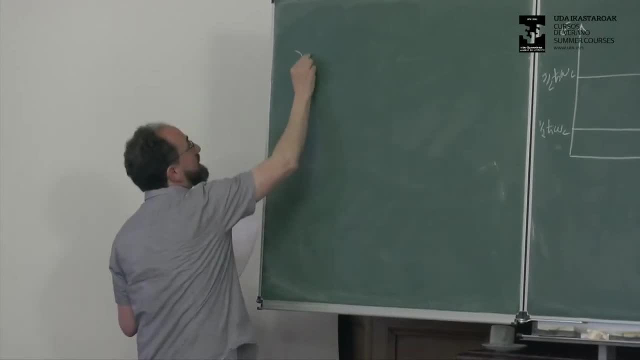 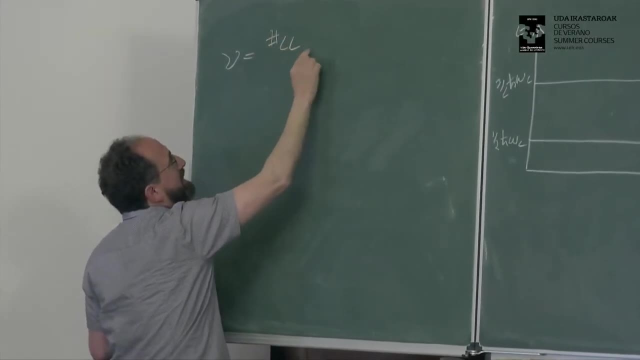 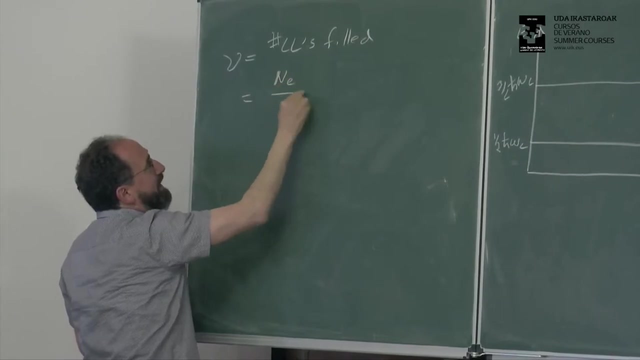 which was this thing we called filling fraction nu, and I claim that this thing, filling fraction nu, is the number of Landau levels filled. Landau levels filled- Why is that? Okay, so it's the number of electrons divided by the degeneracy of a Landau level. 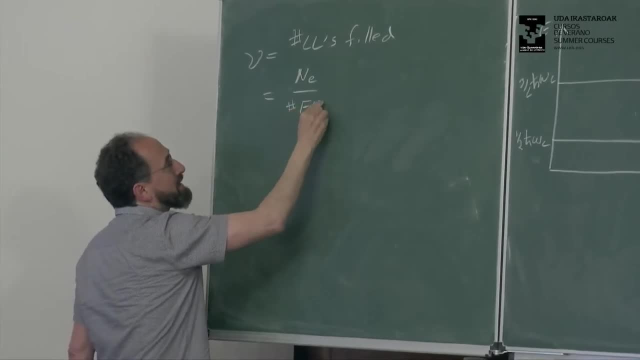 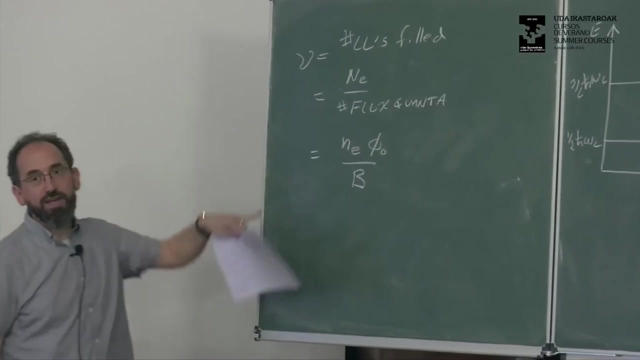 which is the number of flux quanta, and we can rewrite that, if we want, as the density of electrons times the flux quantum divided by the flux density which is the magnetic field. and this is how I define the filling fraction earlier. Everyone still with me. 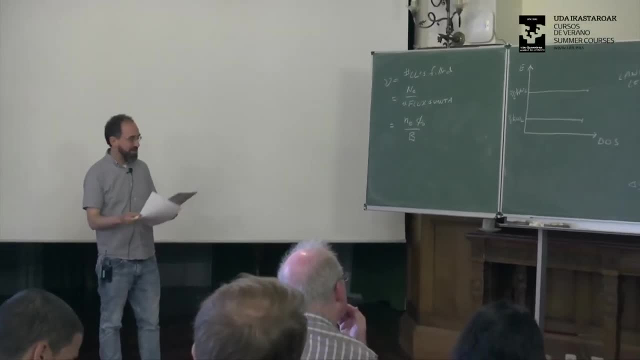 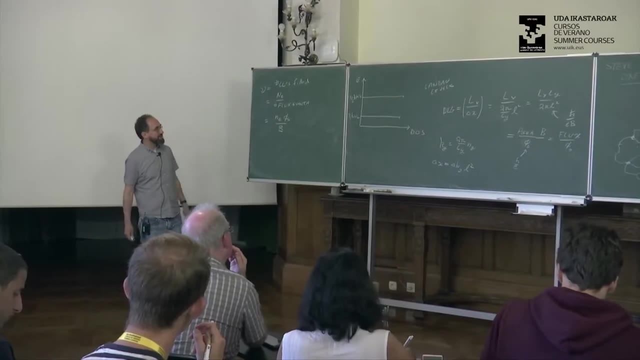 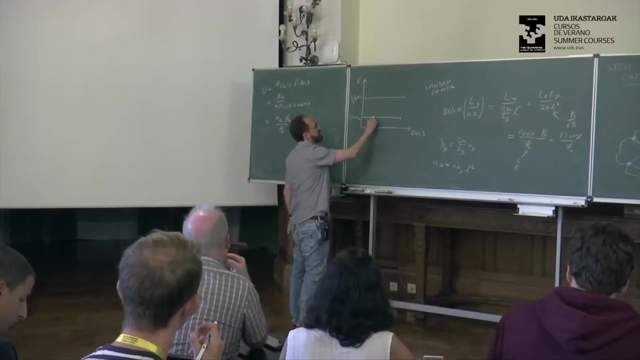 Good, Alright, Alright. so we've made it this far And we see immediately that there's something interesting about this spectrum. If nu is exactly equal to an integer, then we will fill up. we have enough electrons to fill up exactly one of these Landau levels. 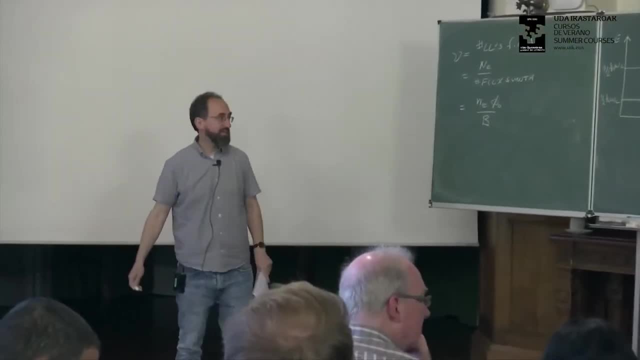 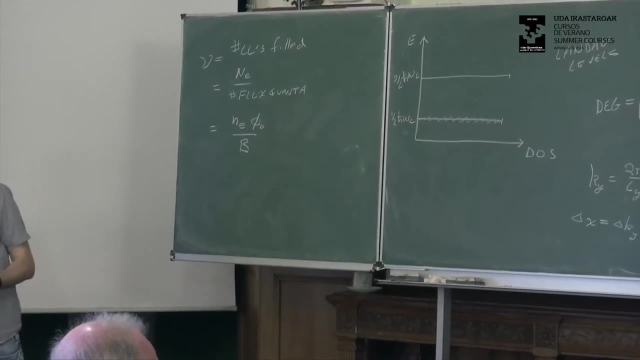 and then there's a gap to making any excitations. The electrons are completely frozen, filling this band and leaving this band completely empty. And that is the essence of what causes our fractional quantum Hall effect. So it looks like an integer, a filled band. 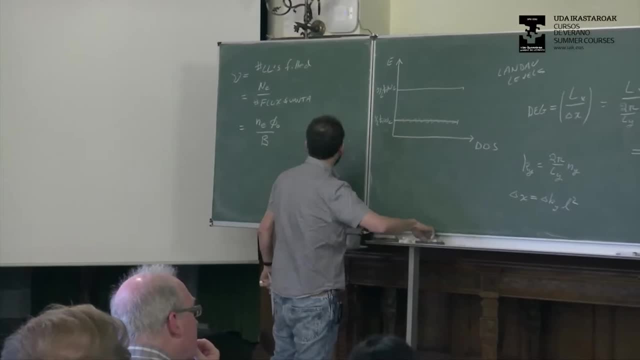 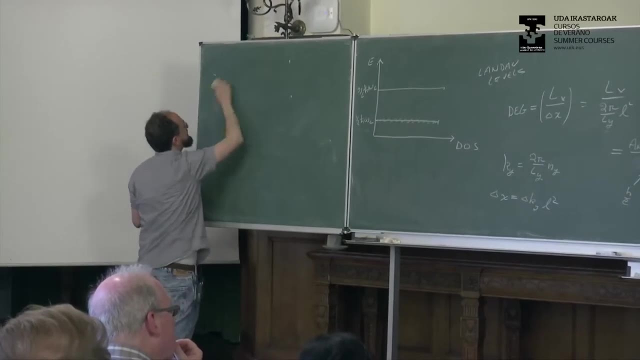 integer with a valence band and an empty filled valence band and an empty conduction band. Now, because Modi is going to talk about edge states, I'm going to switch to talking about edge states and then back up to talking about more physics. 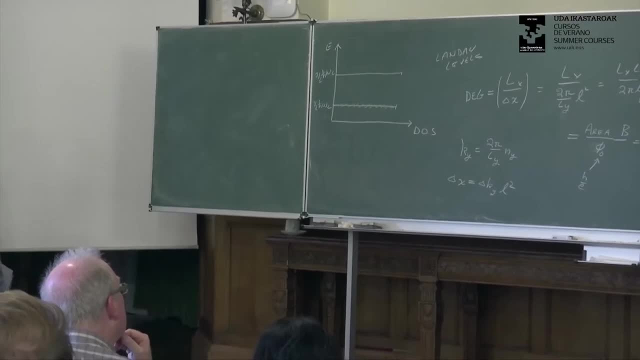 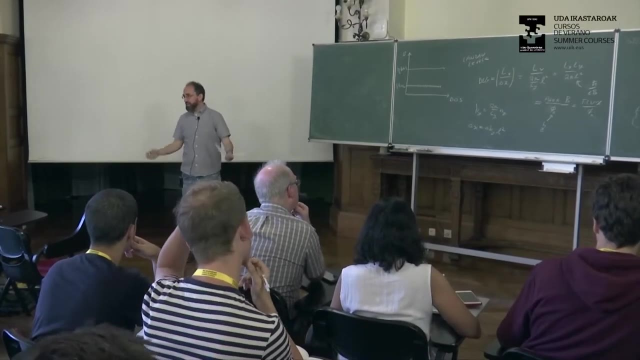 of integer quantum Hall effect. So one thing that I left out in discussing a fractional quantum Hall effect is that in reality, your sample always has edges, no matter what you do, unless you have an infinitely big sample Or you've wrapped your sample up into a 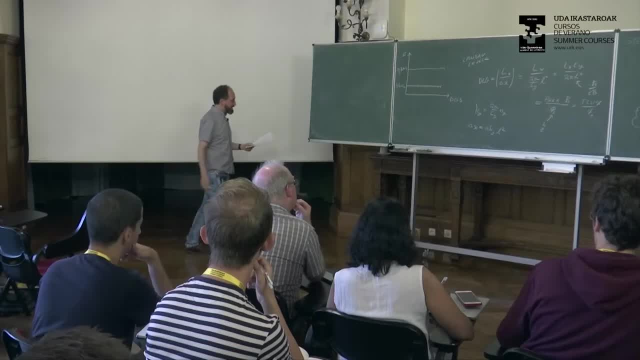 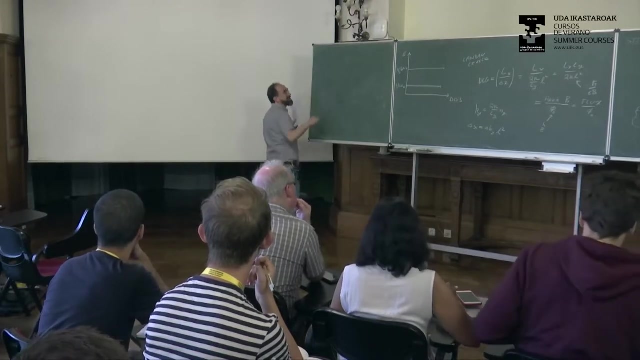 sphere or something like that. your sample is going to have edges and at the edge of the sample there's always some potential holding the electrons inside the sample. otherwise the electrons would spill out of the sample and land on the floor or somewhere Anyway. so there's some sort of 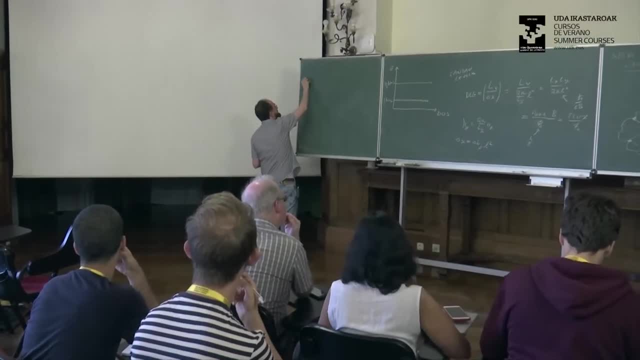 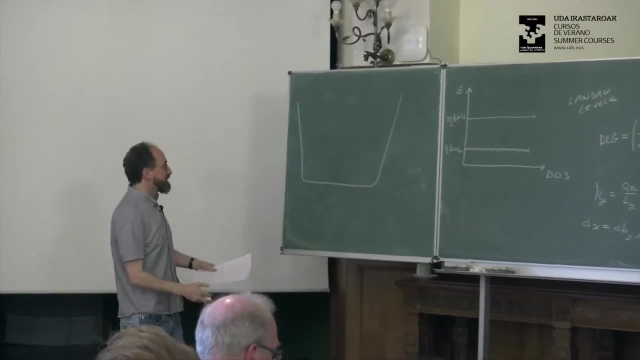 potential that holds the electrons into the sample, and so I'll draw it like this: This is the potential that holds the electrons into the sample. the bulk of the sample, the potential is flat, but then, when you get to the edge, the potential somehow goes up. 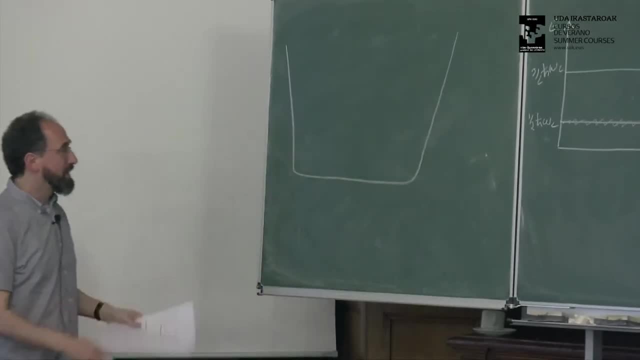 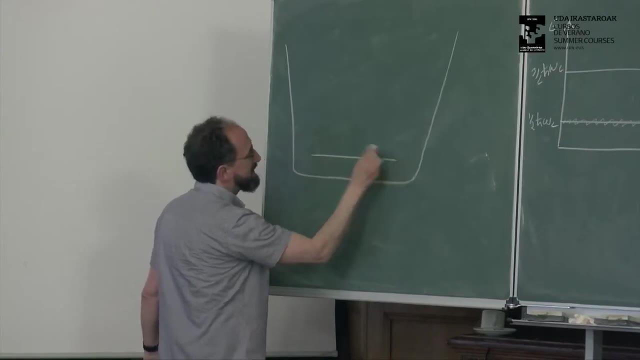 to hold the electrons inward. Now, in the middle of the sample, we're going to have Landau levels. say the lowest Landau level, like this, the next Landau level, like this, and then, when you get to the edge of the sample, 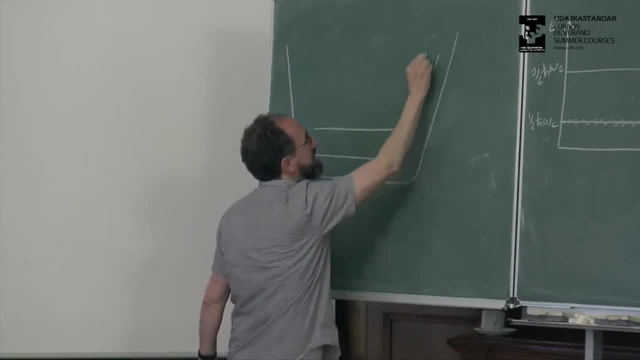 these Landau levels get pushed up in energy. In fact it's not too hard to include the energy in the sample. We're going to include this sort of V of X potential. so this is V of X into our diagonalization of the single body. 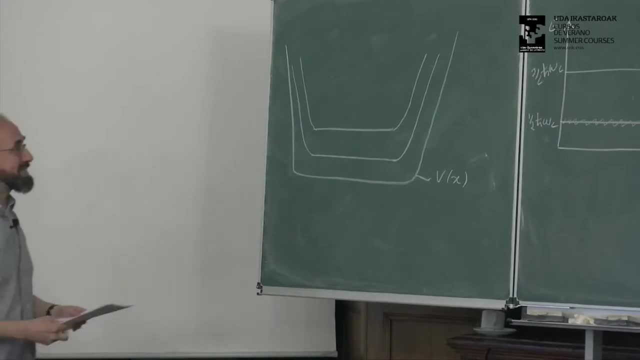 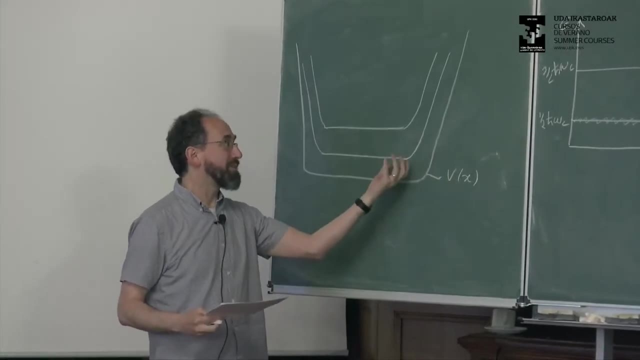 shortener equation that we solved earlier on, which just takes our harmonic oscillator equation, adds this single term to it, but roughly, the eigenstates still look like harmonic oscillator states that just if you're close to the edge, your energy is pushed up. 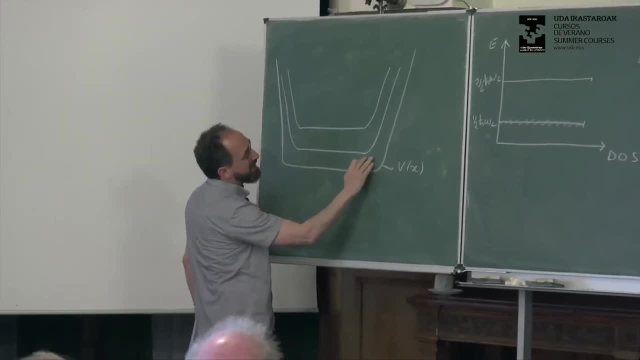 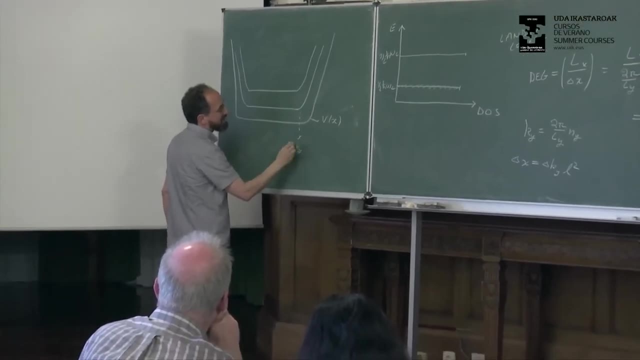 So you still have all these you know eigenstates in these Landau levels, but then as you get close to the edge, so these things here are X near the edge, so it's KY. you know, X is always equal to minus KY times L squared. 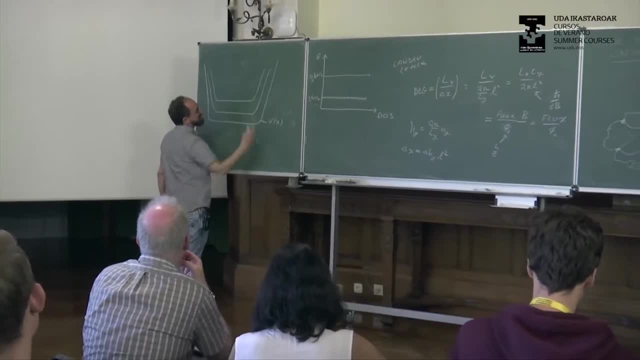 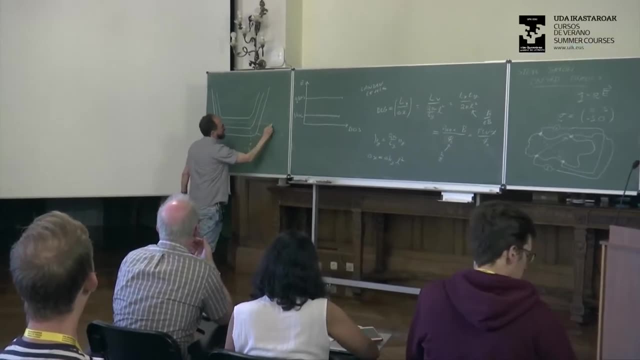 and as KY gets close, you know, pushes you close to the edge, the energy goes up. okay, So now we're going to add a chemical potential, say here, and we're going to fill all the states below the chemical potential and while the bulk 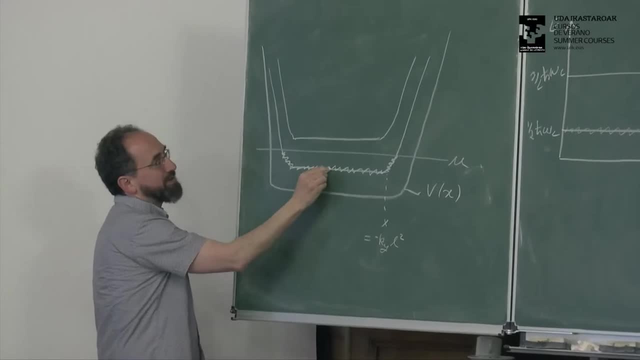 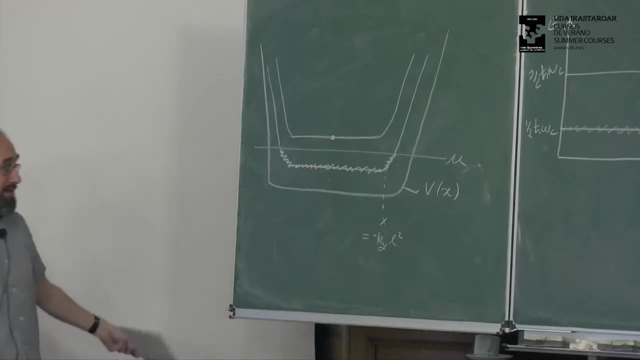 of the system is gapped. you know, if you're sitting here, your lowest energy excitation is to. you know, make a hole here and put an electron up there and that's, you know, very high energy if the cyclotron energy is large, in other words, if you're. 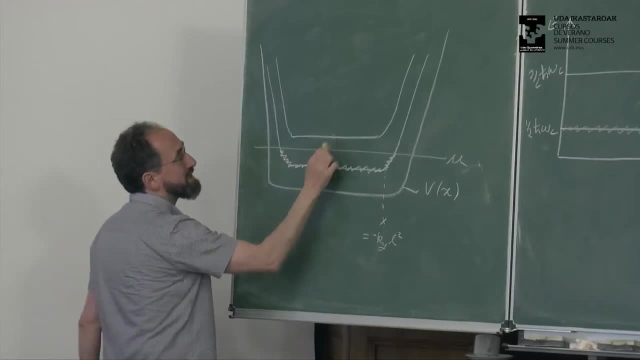 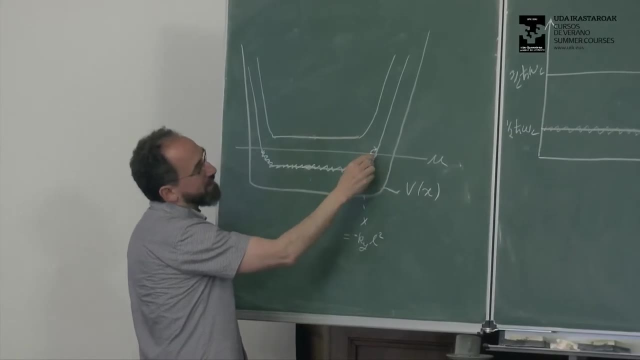 in a large magnetic field. so you're not going to make any of these excitations. but near the edge of the sample there are low energy excitations We can take. you know we have a Fermi surface. if you want to think of it that way, we have a place. 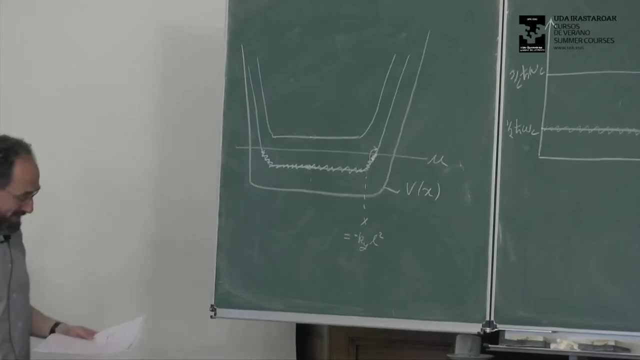 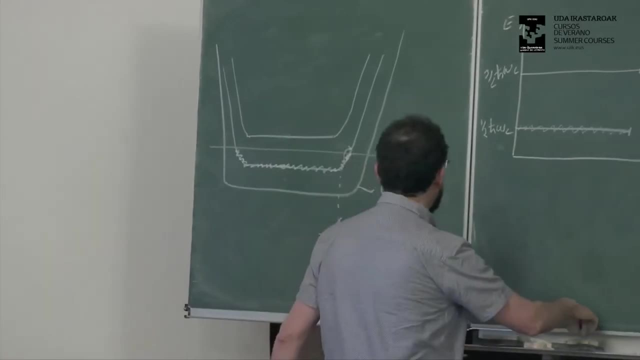 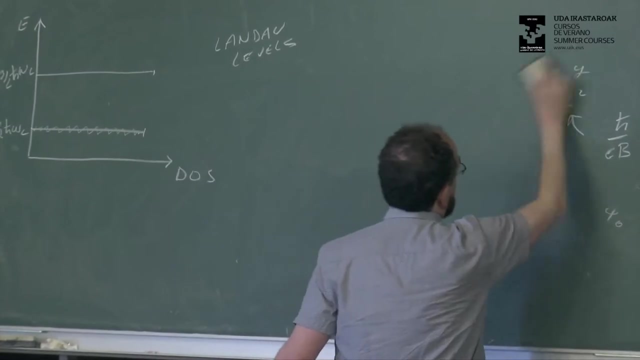 where empty states meet filled states, and this is where you can have low energy edge excitations. and there's another nice way to think about these edge excitations, or these edge modes which make them feel, you know, much more natural, I think. 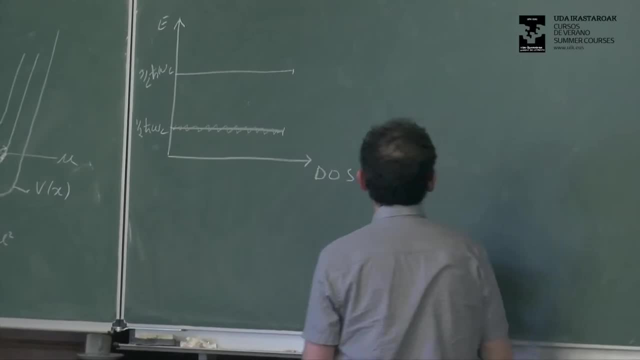 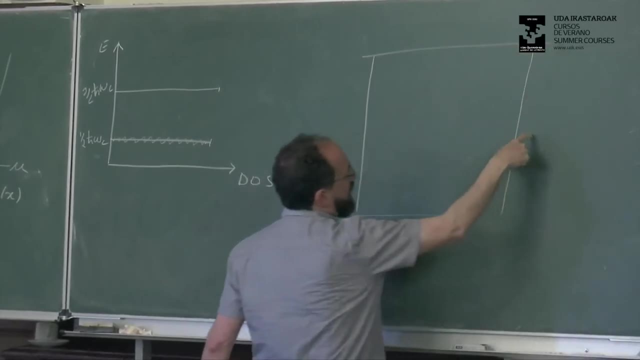 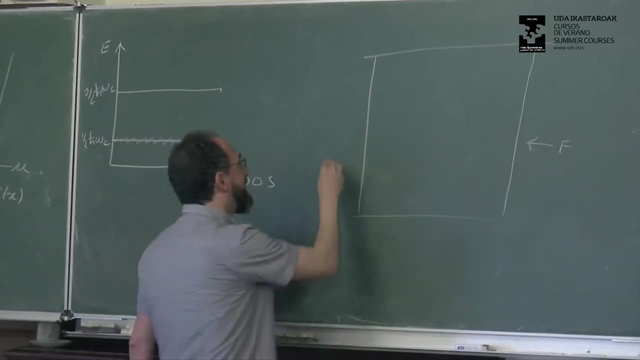 which is to think of. okay, here's my two-dimensional system, with my edges, okay, and on the edge we have some sort of force holding the force, which, incidentally, the force holds the energy. The force is always with you and I just have to get. 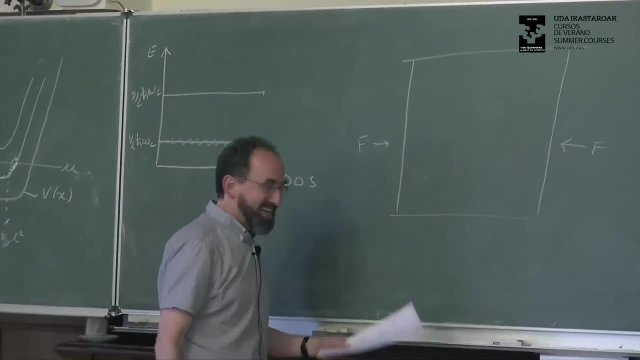 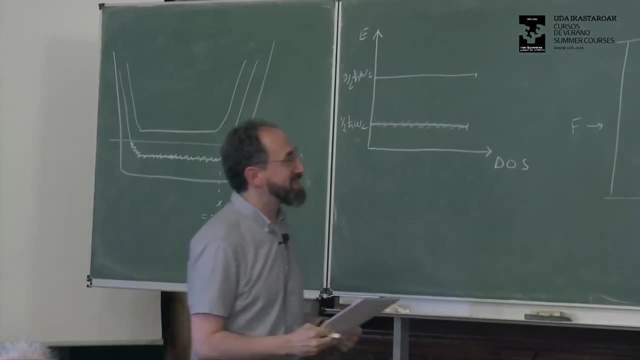 into some Star Wars reference there. The new movie's coming out December 19th, incidentally. So there's some force holding the electrons into the sample, so think of it as an electric field, and there's a magnetic field which is perpendicular to. 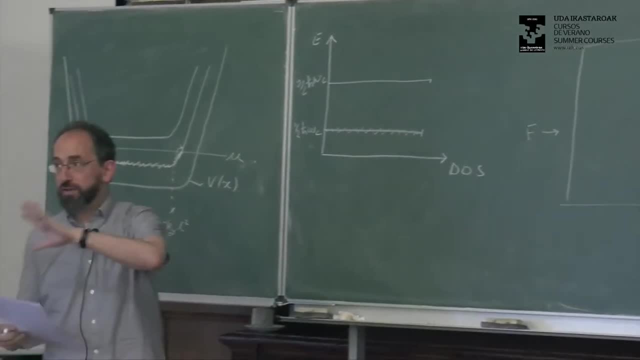 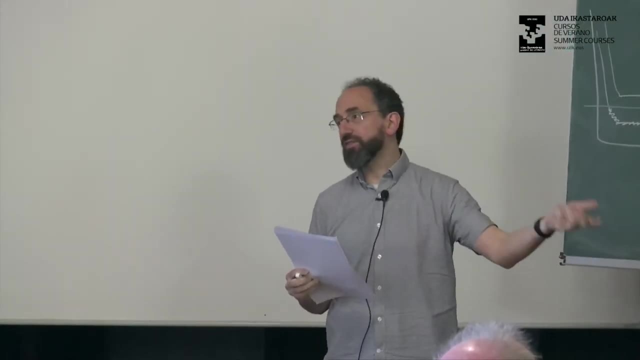 the plane of the sample. and we know just from you, know elementary freshman physics- when you have a crossed electric and magnetic field, charged particles exhibit a drift velocity. So in this region, near the edge, where there's a slope, 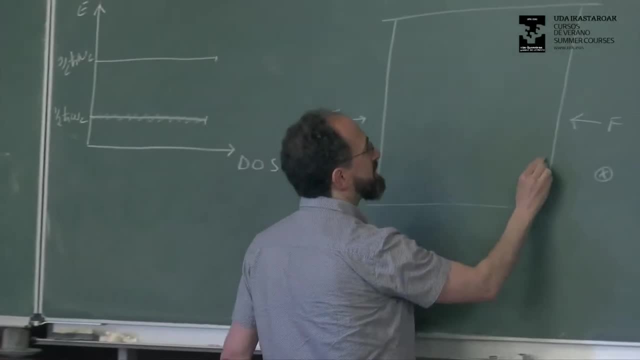 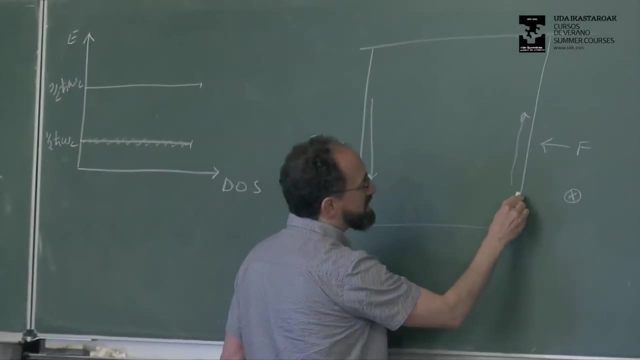 to the potential. there's going to be a drift velocity running along the edge and a drift velocity here running along this edge. So if I make now a little bit of a bump in the shape of the edge, add a little bit of an electric, you know. 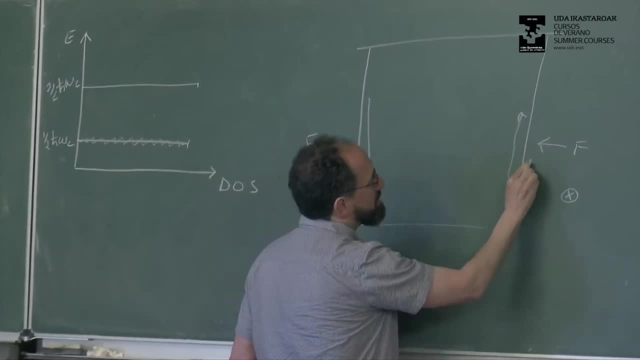 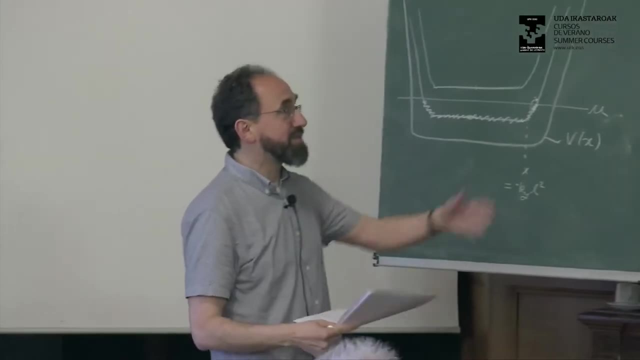 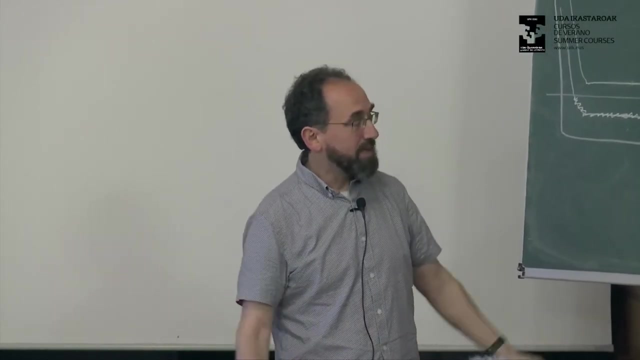 an extra electron on this edge, it's going to drift along the edge in that direction, carrying its charge with them. And this is very typical, as we heard from Charlie, this is very typical of topological insulators, that there will be some sort of edge modes. and because these 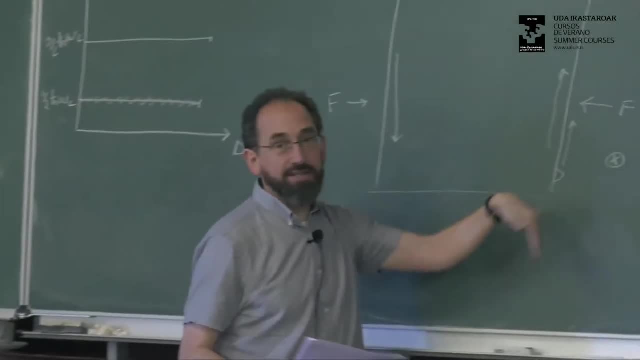 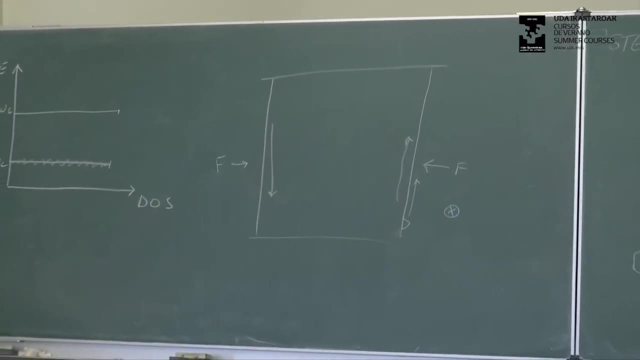 are chiral edge modes. they can only move in one direction. they can't come back and move in the other direction. so they're protected from disorder. Now we can do. is everyone still happy? Okay, good, So we can do a little bit better. 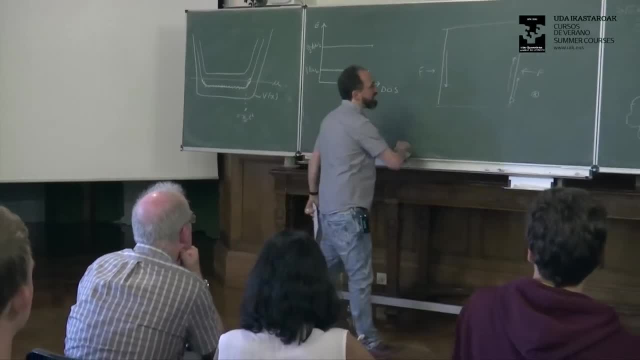 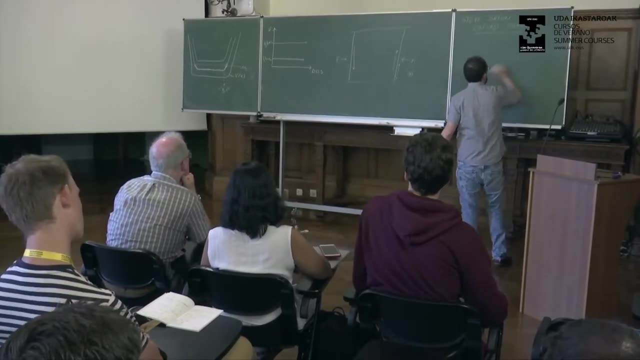 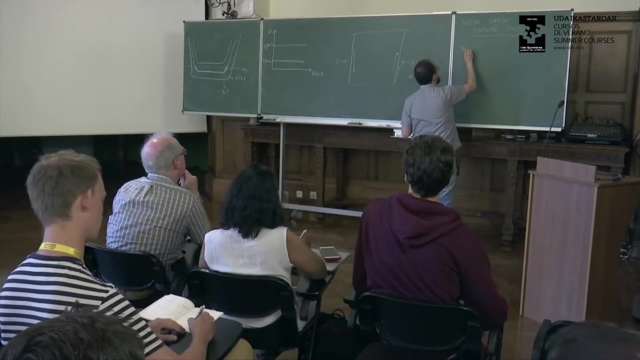 We can actually calculate how much current these edge modes carry, And to do that we want to know something about the velocity of these edges. and the velocity is pretty easy to calculate. Charlie did it briefly. Well, okay, the group velocity is always d, omega, d, k. 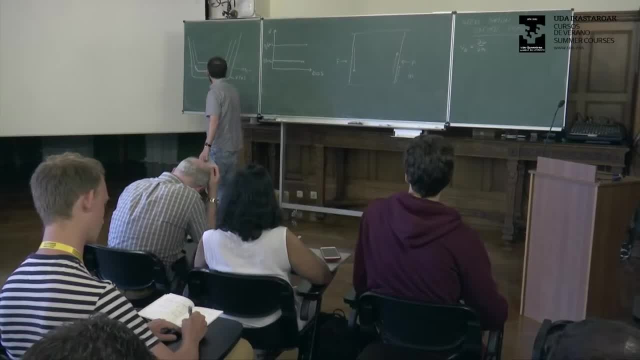 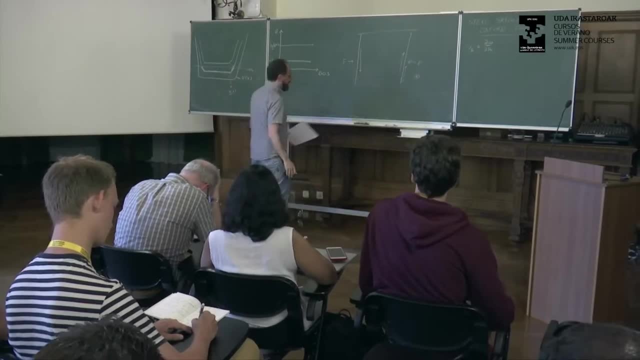 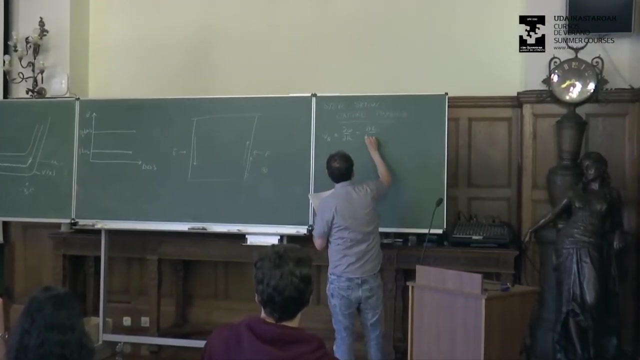 So remember that the k here is really equivalent to position. so we're asking: what's the change in energy with position? basically? So we can write it as d energy d k if we want. So it's d e divided by h bar d k, like this. and if we want to, 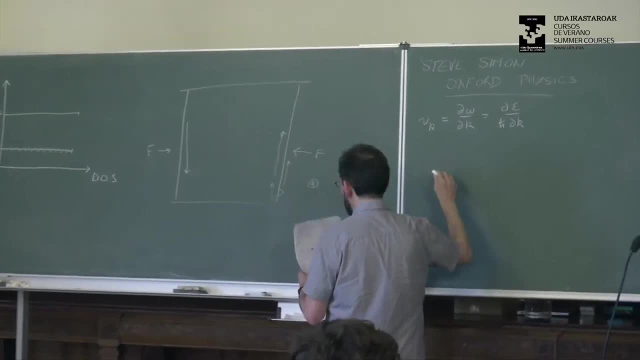 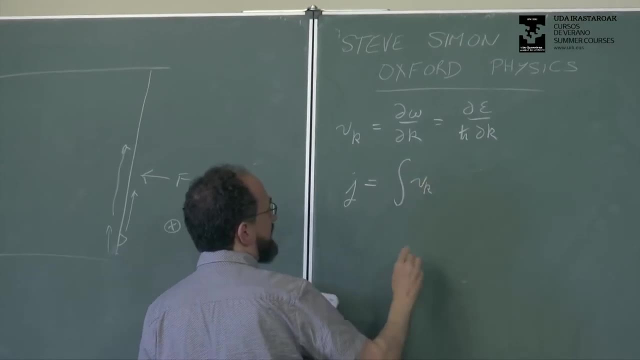 add up all of the current that's flowing this direction near the edge. we then just write: the current equals the integral of v k, d k, like this: I guess d k always comes with a divided by 2 pi, and then, if we want the charged current instead of the particle current, 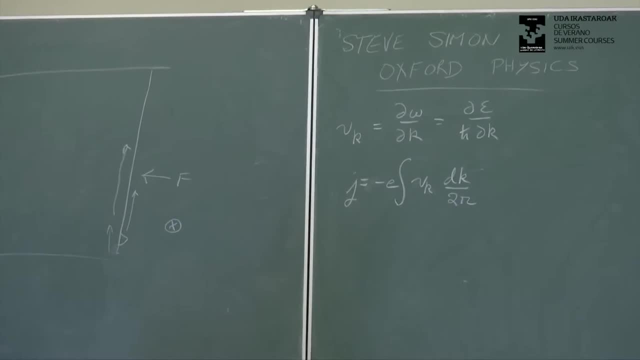 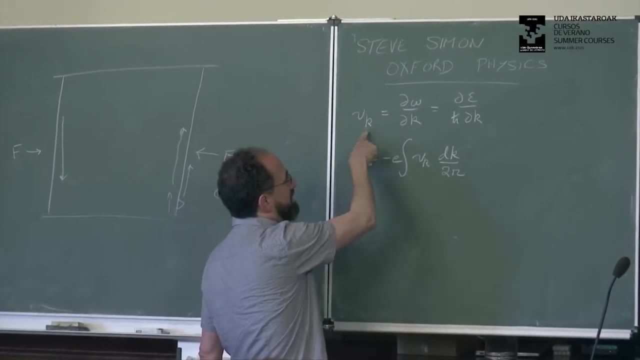 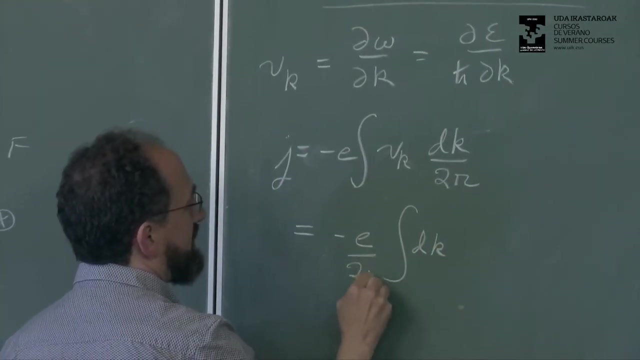 we add a minus e out front and this gives us the total current flowing along the edge. Now, if we take this expression and insert the expression for v here, we get minus e, integral d k. I'll pull out the 2 pi here and then we have d e d k. 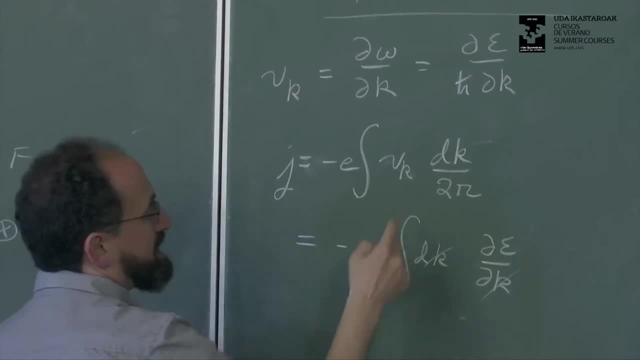 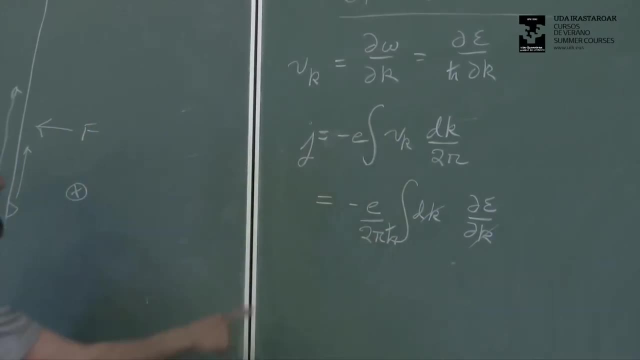 We can cancel the two d ks with each other and just have an integral d e. There's an h bar I missed, so 2 pi h bar There. so the 2 pi h bar becomes an e over h. There's a minus e over h and we're left with integral d e. 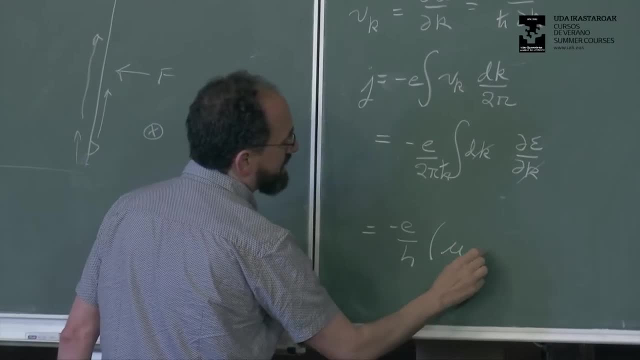 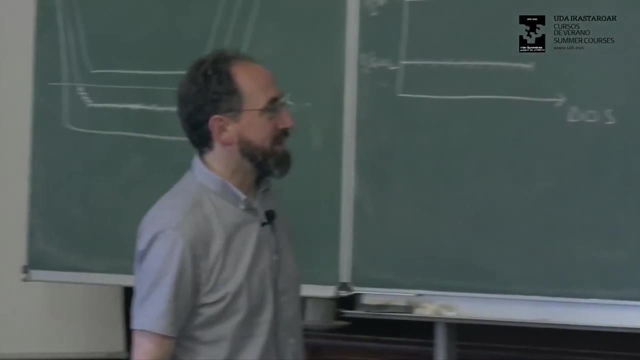 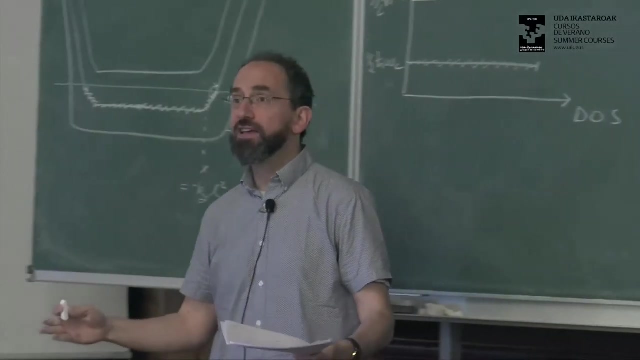 and this will be the chemical potential of the edge minus the chemical potential of the bulk. It will be the total current carried by the edge. Now, all we have to do then is: so now we're going to do a simplified quantum hall experiment here. 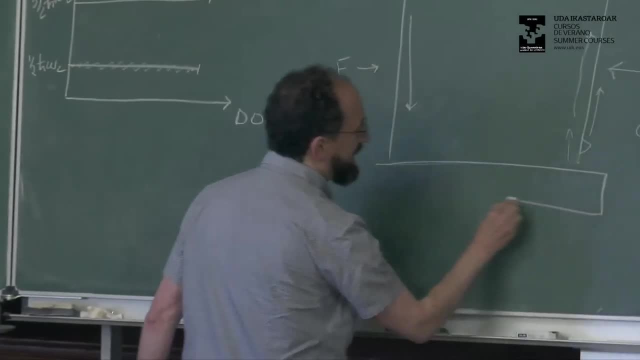 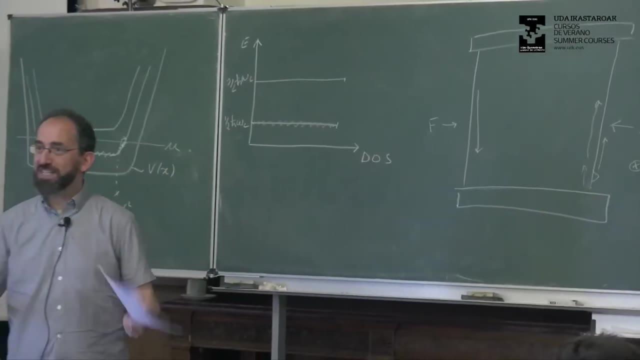 The simplified experiment. The idea is to put one contact way down here and another contact way up here, and experimentalists will know why it is. you don't do two contact experiments, but let's imagine an ideal two contact experiment where you have perfect contacts and things like that. 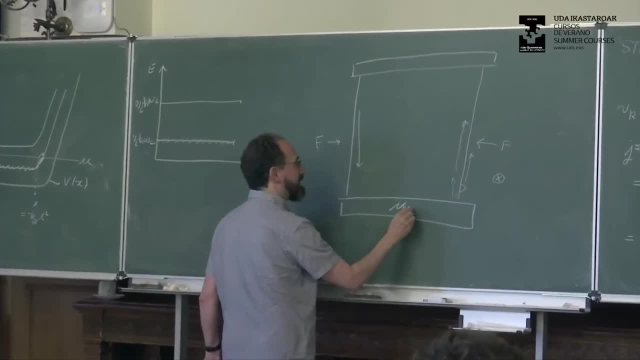 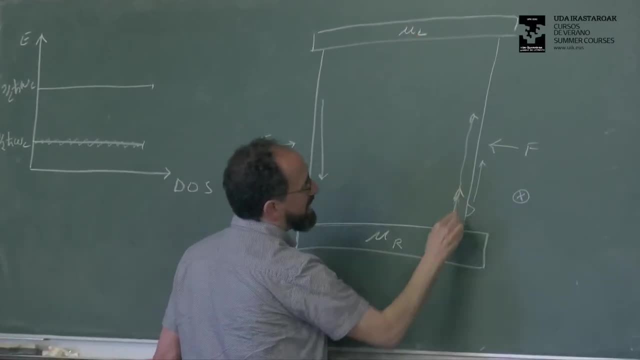 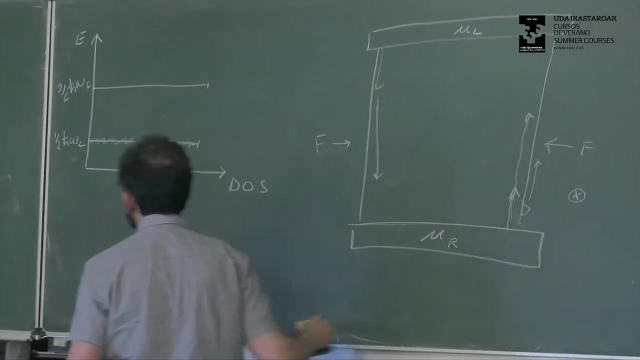 We can put one chemical potential here, call it mu right, and another chemical potential up here, we'll call it mu left. This edge will get mu right. This edge, going this way, will have mu left, And then the total current. oh boy, where am I going to put this? 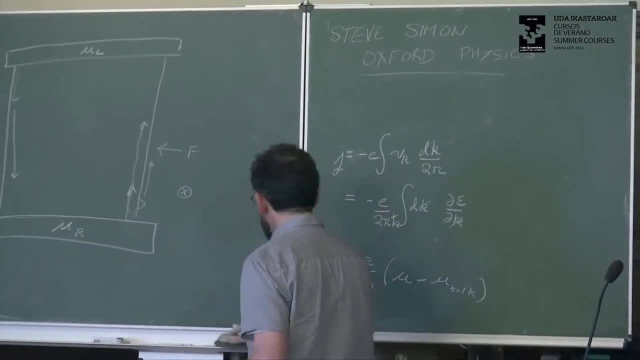 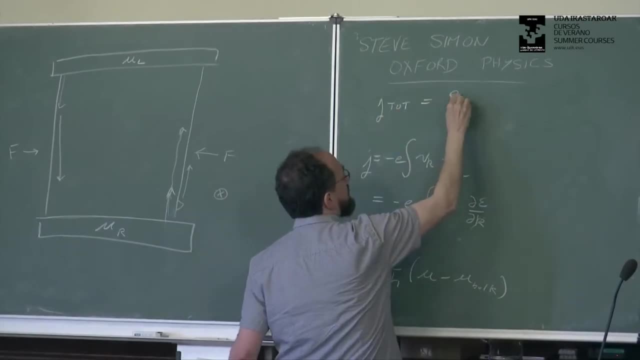 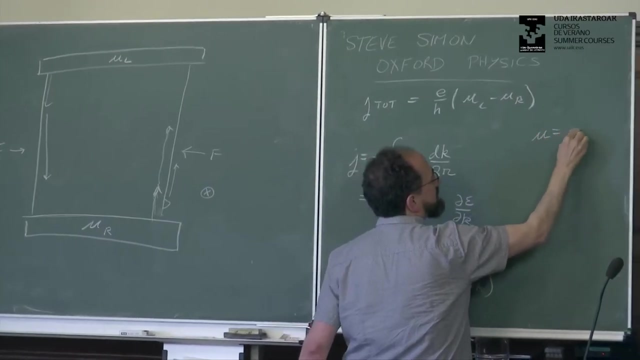 Put it over here, I guess The total current will then be j. total running along the sample is then e over h, mu left minus mu right, and using the chemical potential is just e times v. This then gives us the two terminal g, two terminal. 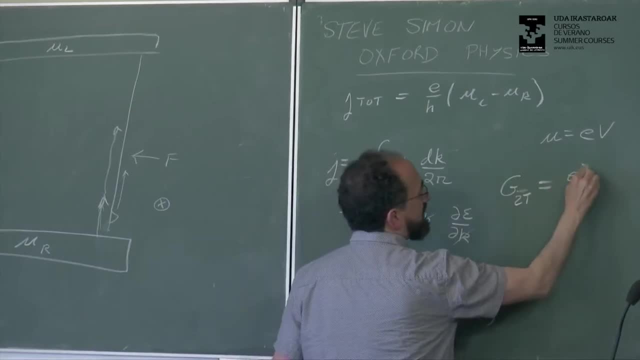 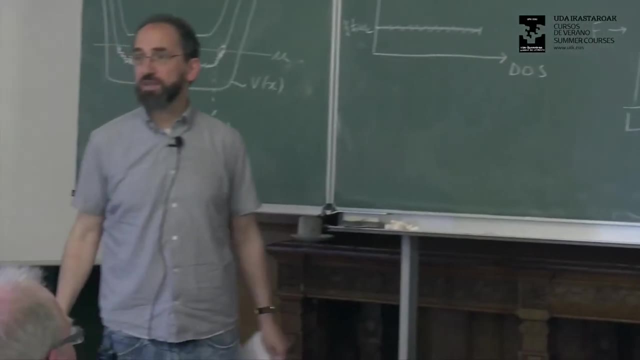 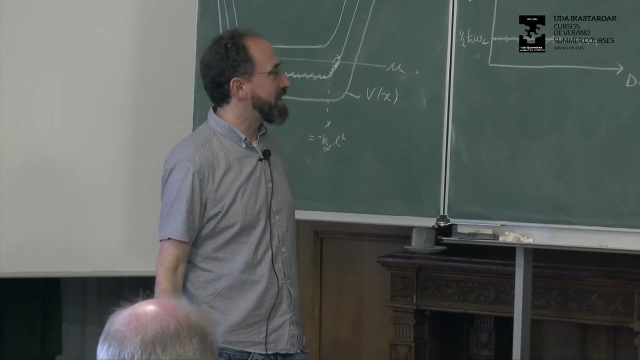 The two terminal conductance between these two things is e squared over h, So we re-derived the quantum hall conductance in a two terminal experiment. this way Now, as Charlie mentioned, and I think Modi will mention quite a bit, we can actually do the same thing, but with thermal currents rather. 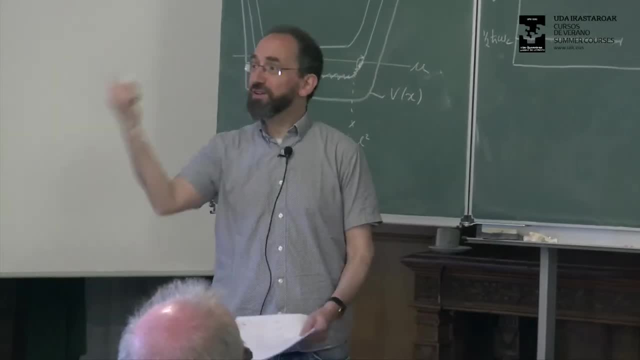 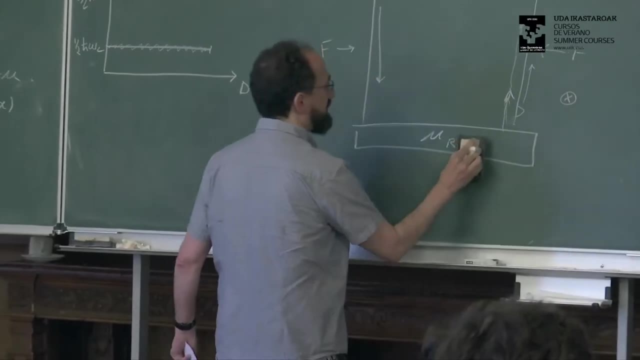 than electrical currents. This is a homework problem, so you can go to the website and get hints for how you do this. but in the thermal experiment, what we're going to do is we're going to fix both chemical potentials to be the same. 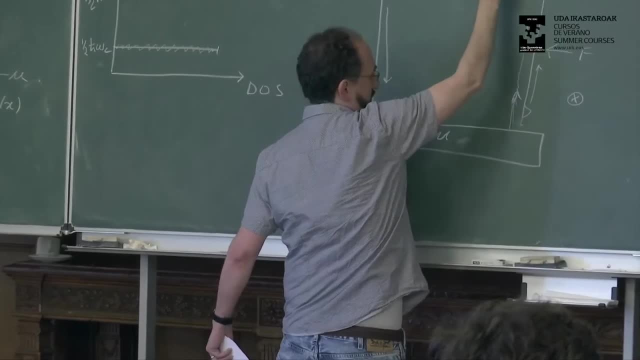 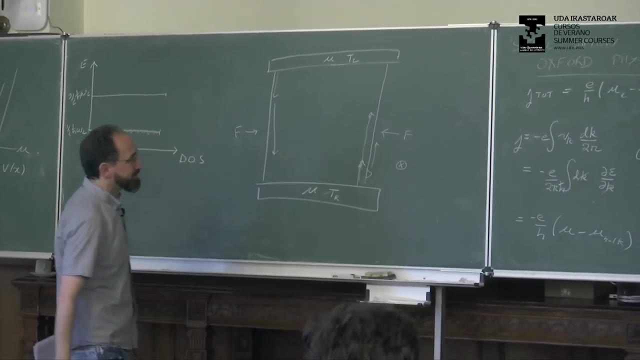 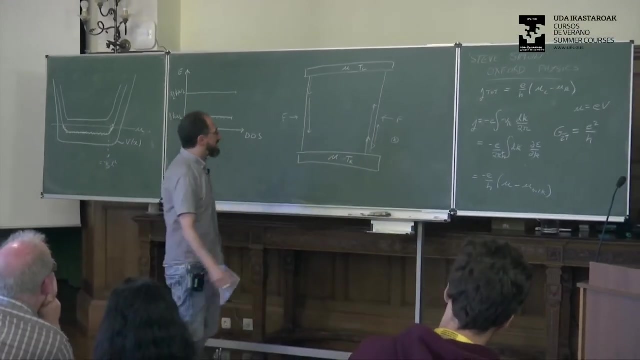 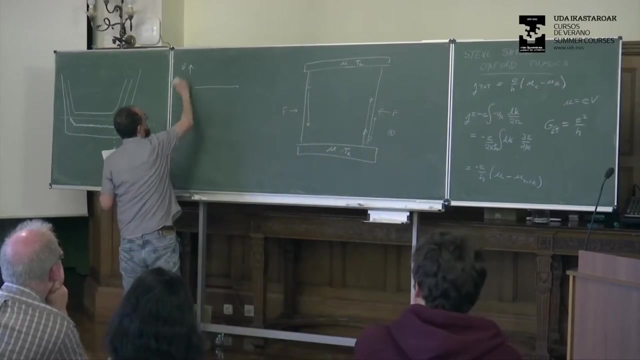 both the top and the bottom. but we're going to have different temperatures- T right and T left, T right here and T left- And we want to calculate the total thermal current that we get flowing from one end to the other. Well, okay, let me erase this and explain how that's going to work. 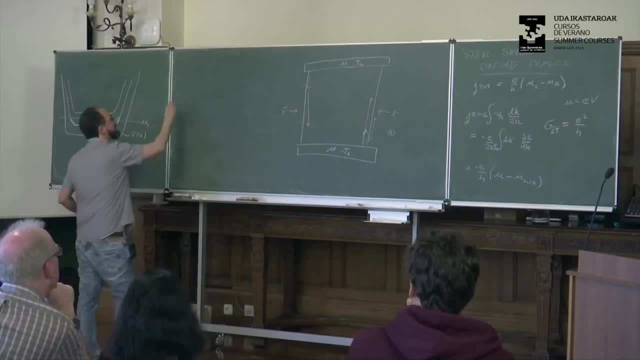 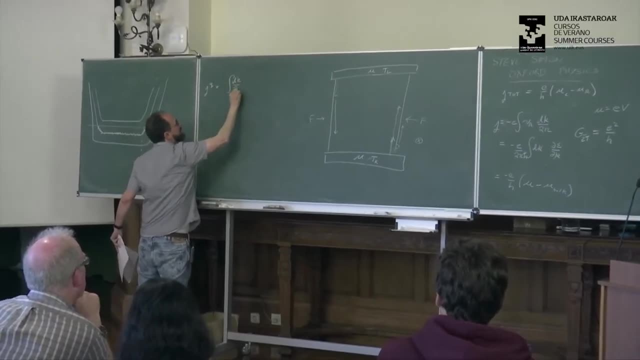 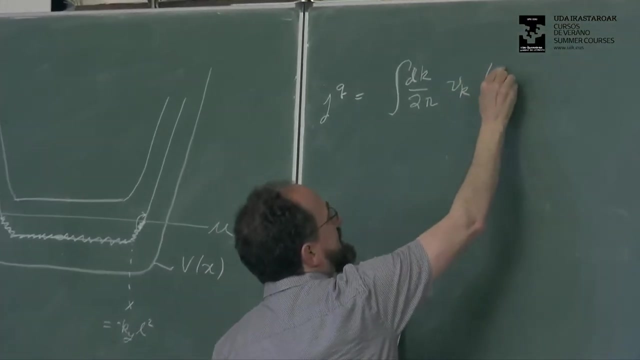 It's very, it's actually very- similar that the total thermal current jq, it's the same integral of the k over two pi. the velocity of each eigenstate, v sub k, and then the energy of the eigenstate, because we want to know how much energy it's carrying. so that's e sub k minus mu. 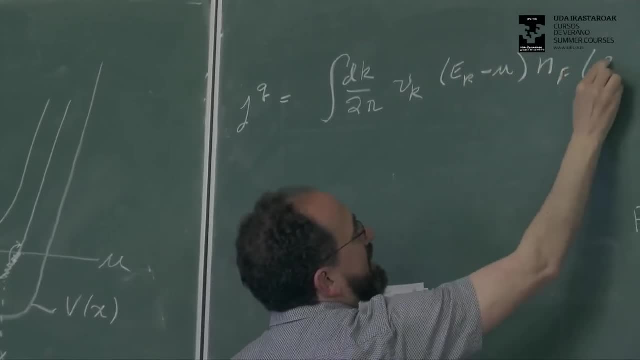 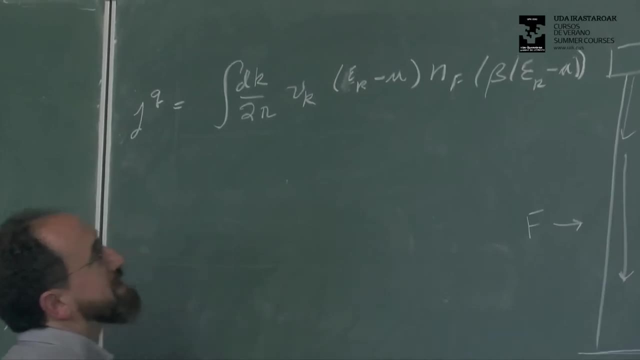 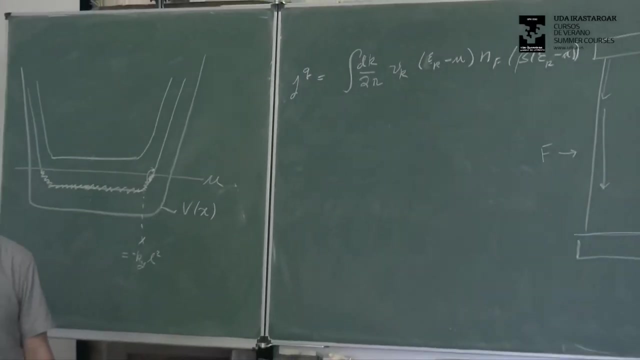 and then how occupied it is. The Fermi occupation factor of beta e k minus mu. use epsilon e sub k like this, and that gives us a formula for how much heat is carried by a quantum Hall edge. Then doing basically exactly the same manipulation, here with a slightly 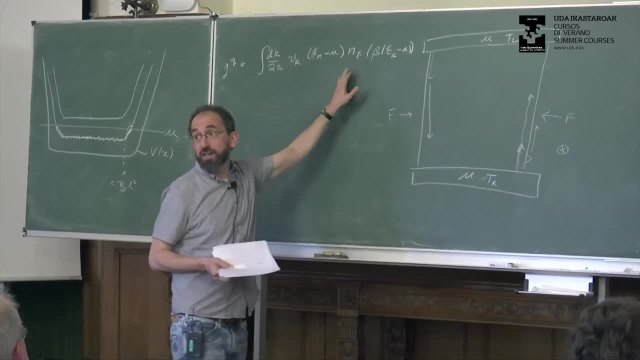 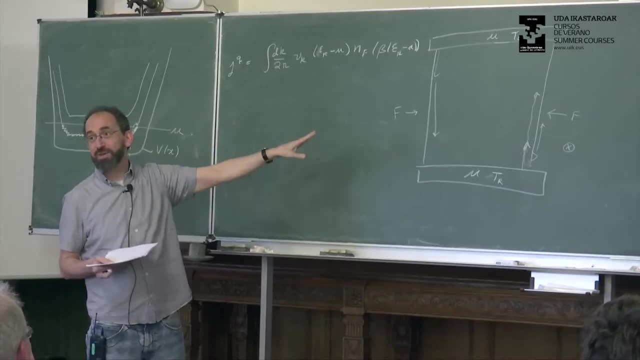 more complicated integral because of this Fermi factor. so those of you who are good with integrals will be able to do the integral. If you're not good with integrals, plug it into Mathematica or you can look on my web page. it gives you a hint of which integral you need to look. 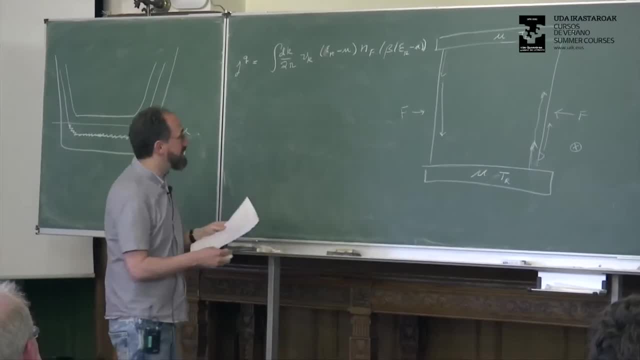 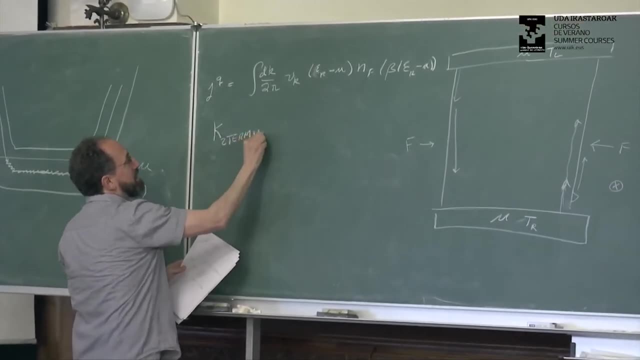 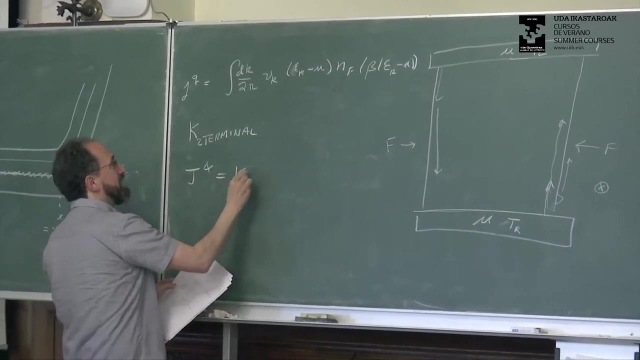 up and then you do this and you can calculate the result that the two terminal, k two terminal. well, that's what we're going to calculate. Let me define that. So the total thermal current is k, two terminal, k two terminal times the 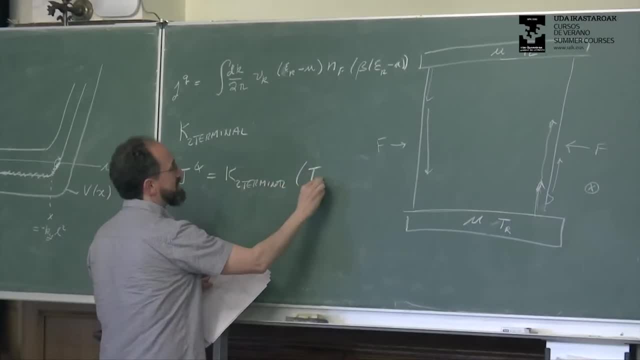 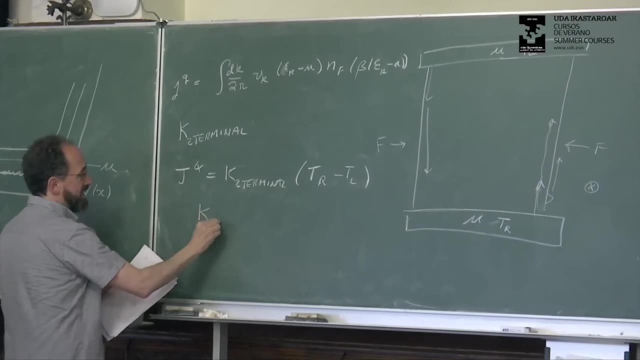 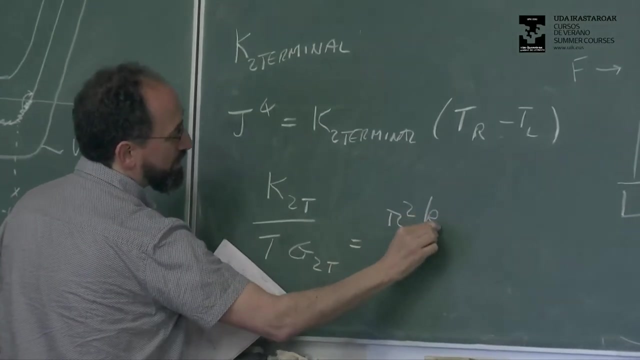 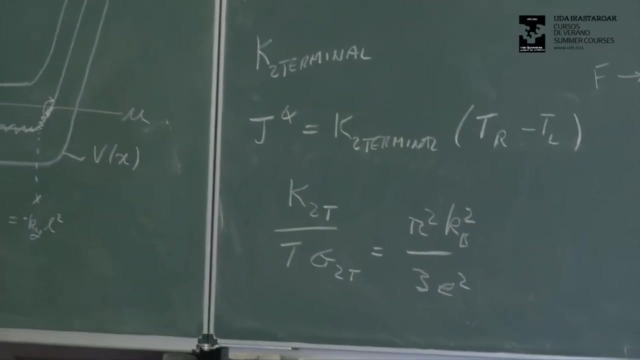 difference in heat, in temperatures t right minus t left, And the statement that you're asked to prove is k two terminal divided by temperature times. g two terminal is pi squared, Boltzmann's constant squared divided by three, e squared. That's known as the Wiedemann-Franz law, which holds in a lot of physical. 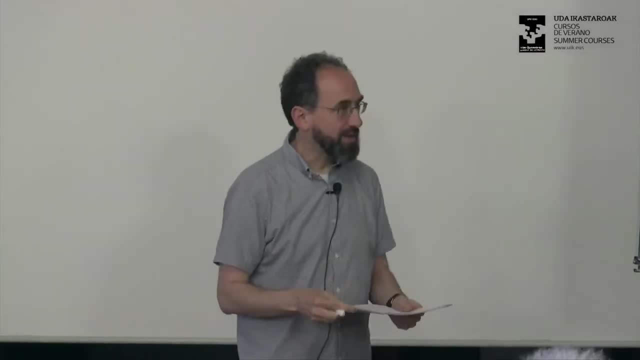 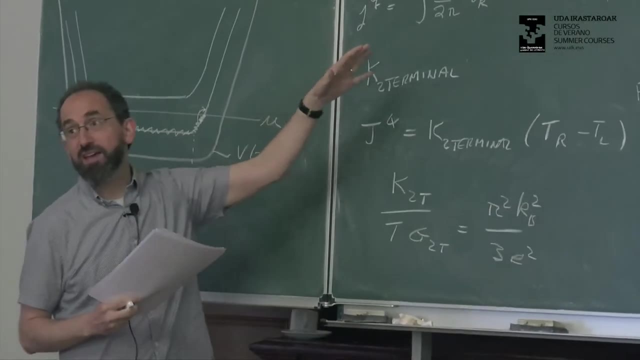 systems, but not all physical systems. And if one is really really aggressive, you can do what Charlie suggested, which is to try to calculate the same thing in boson language and see if you get the same result. and you should, Yes. 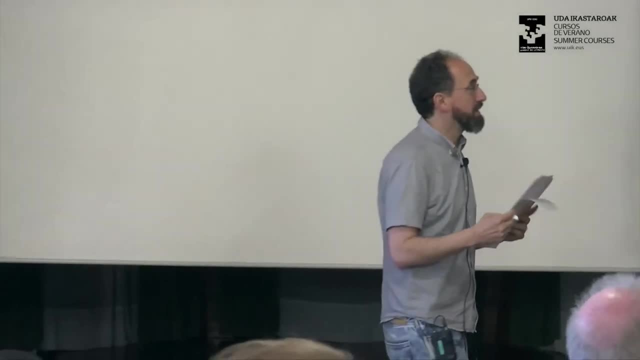 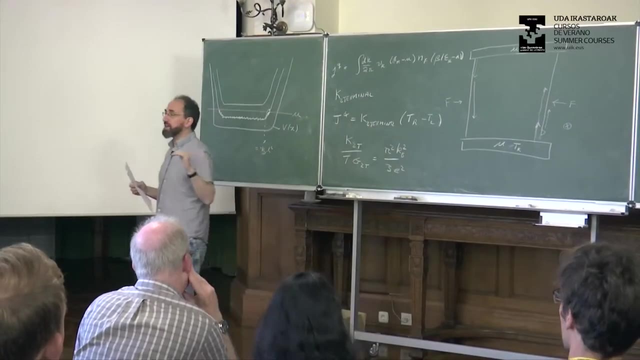 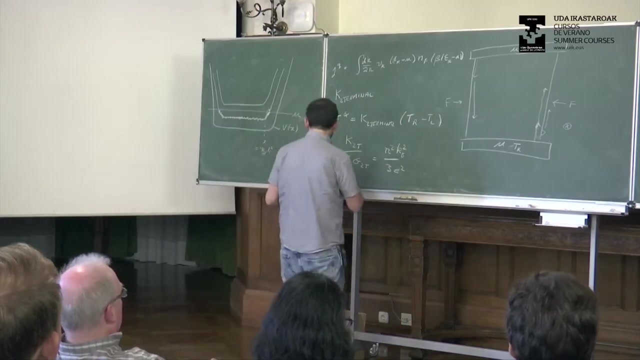 No, it's independent of length, It's temperature difference only. So you're right that this is a conductance, not a conductivity. Yeah, Okay, So this is all I'm going to say about oh. no, there's actually one more thing. 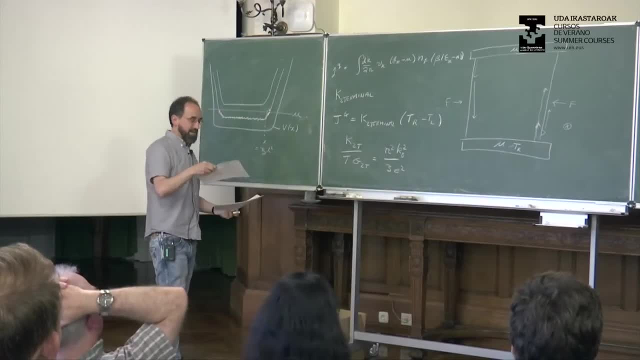 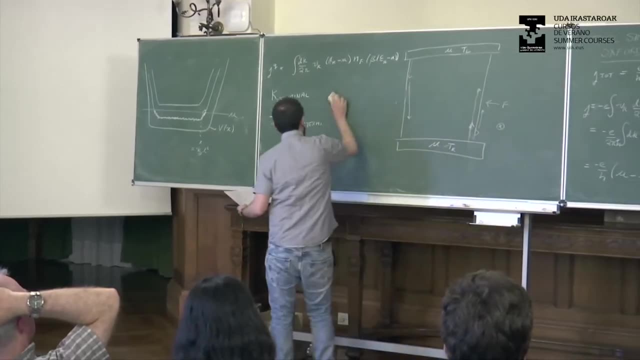 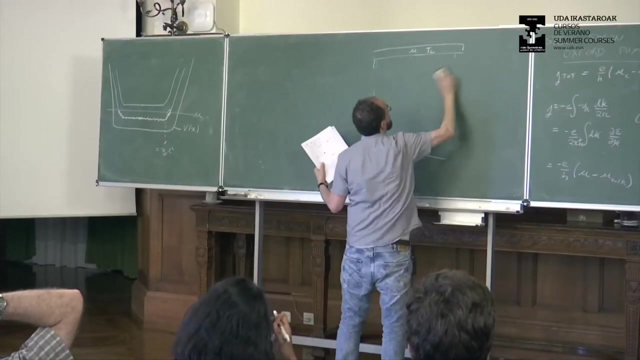 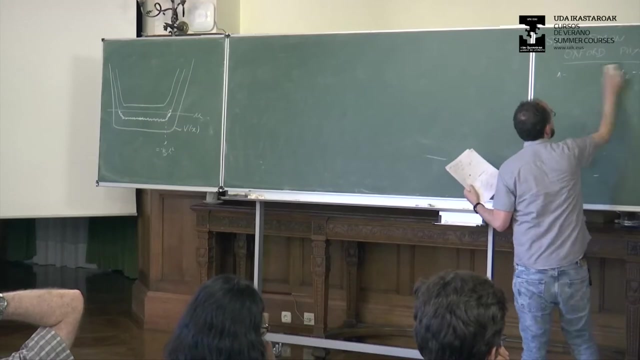 I want to say about edge modes, Which is another homework assignment. So this was one homework assignment. I'm going to get rid of this. now One can look a little bit more closely at the edge modes in detail. Okay Go, You can look a little bit more closely at the edge modes in detail. 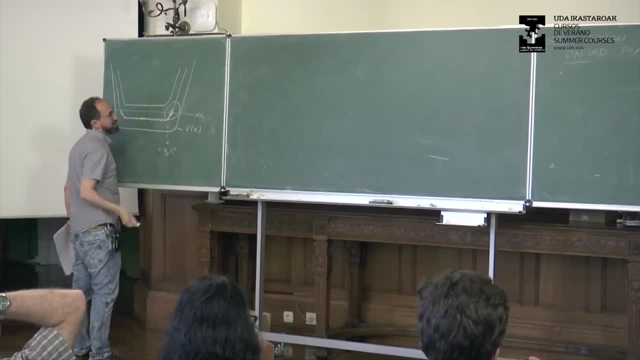 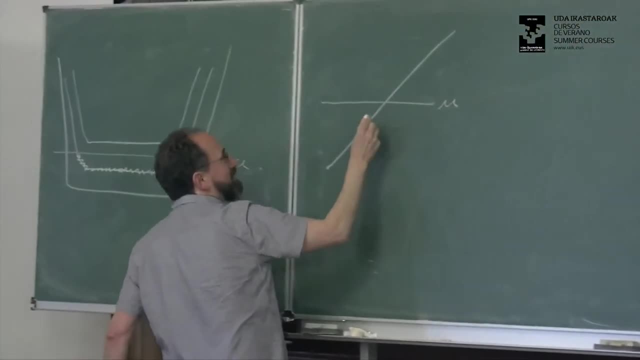 So I'm going to look here and I'm going to blow this up until it's really big. So, looking like this, blowing up until it's really big, Here's the chemical potential mu, And if I look really closely I'll see there are individual k states at different values of k. 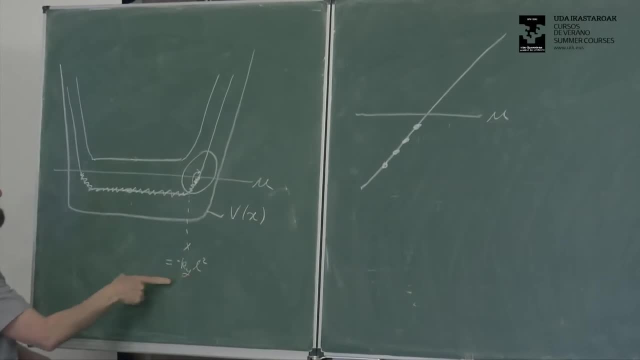 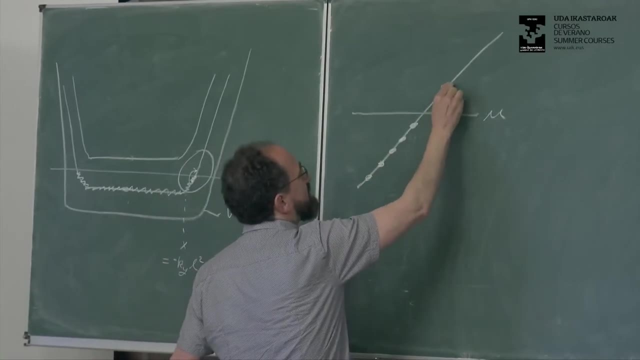 Because, remember, the x direction here and the k direction are really the same thing. So these are individual possible k states, These guys being filled and these guys being empty. And this is in the ground state, because everything below the chemical potential is filled. 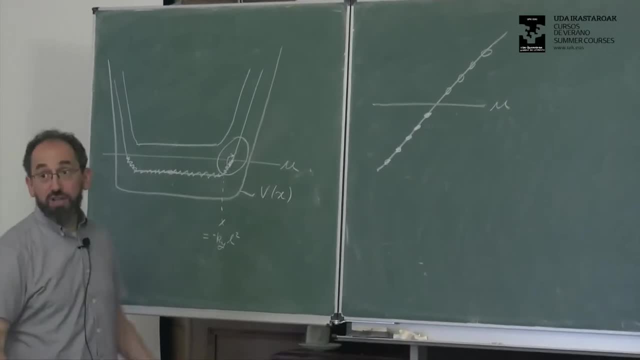 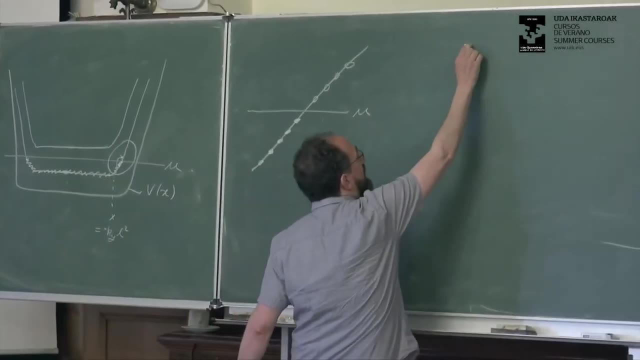 and everyone above the chemical potential is filled. Everything below the chemical potential is empty. And we want to look at what are the low energy excitations of this system. Well, there's one low energy excitation: who has one unit of steps in k's? 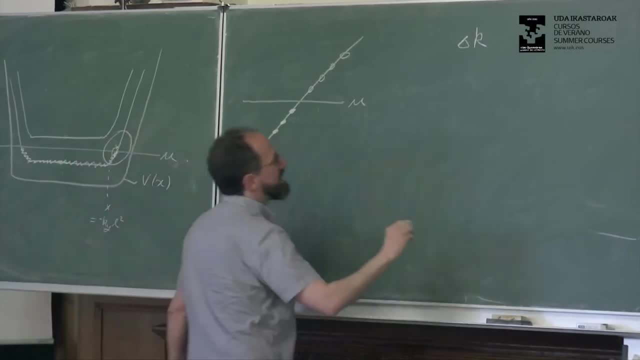 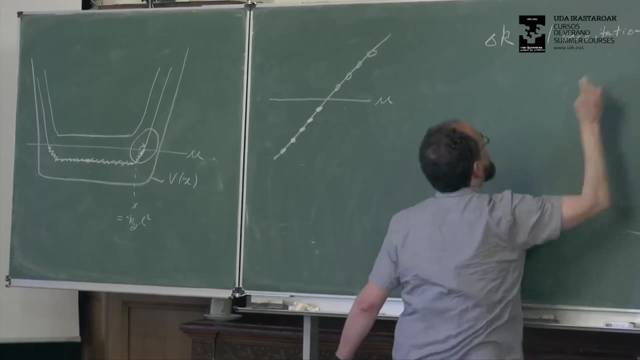 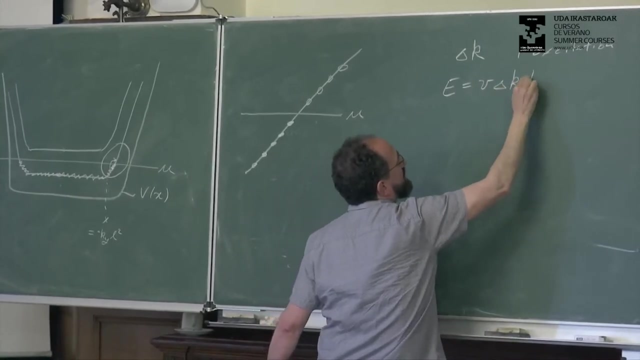 k's are separated by some distance. There's one excitation of unit delta k. One excitation. Its energy will be the velocity of the edge, The slope of the edge, times delta k, I guess, times an h bar. And that excitation is to take this guy who's closest to the chemical potential. 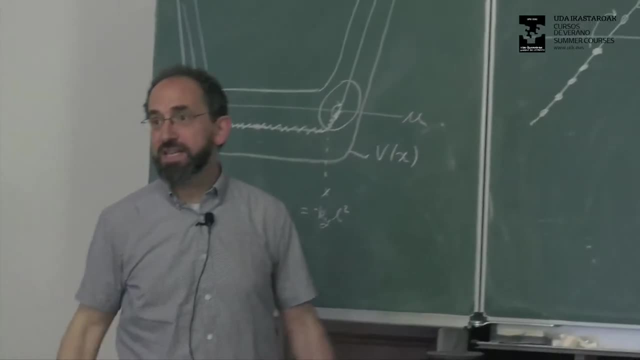 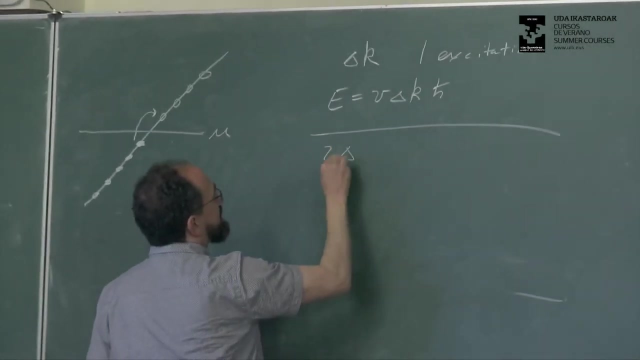 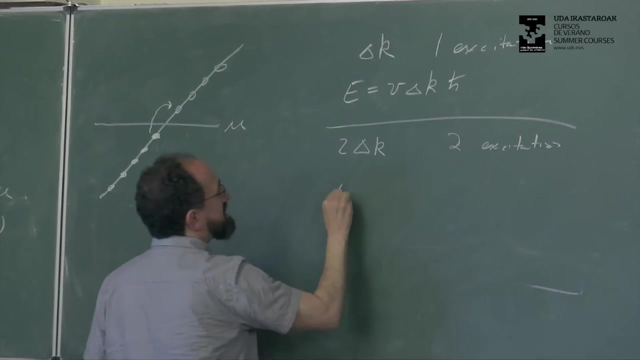 and push him up to here. That's the lowest energy excitation we can have at the edge. The next lowest excitation call it 2 delta k. There are two such excitations that you can make And their energies will be 2 times the delta k total distance. 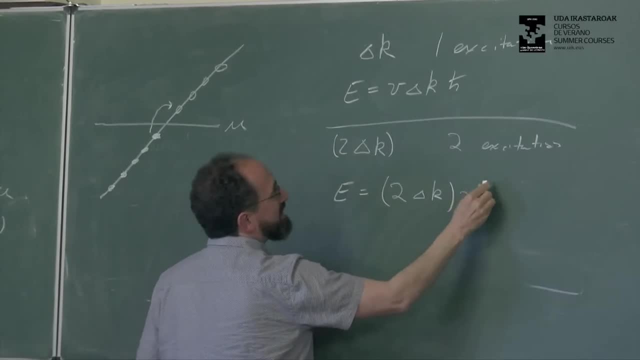 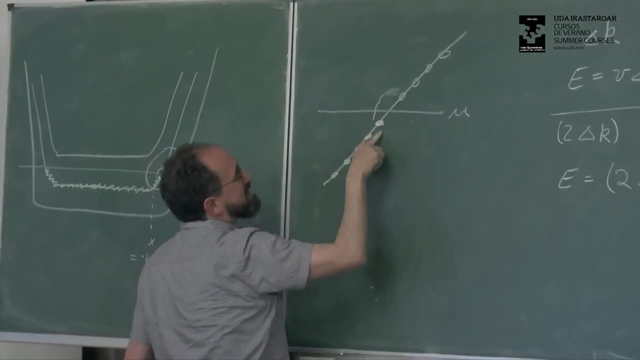 It has total momentum 2 times delta, k times v times h bar. I wrote it in a different order now, And these excitations can be described in the following way: One of them is to take this guy, push him two steps up to here. 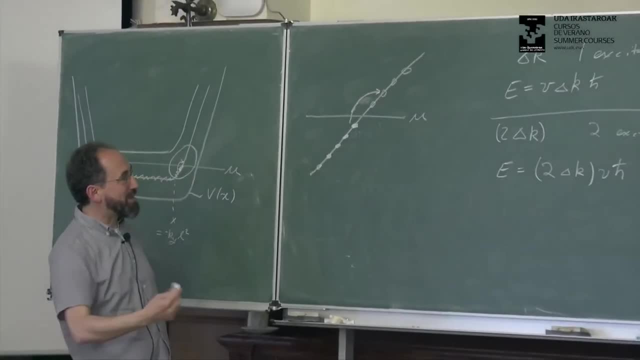 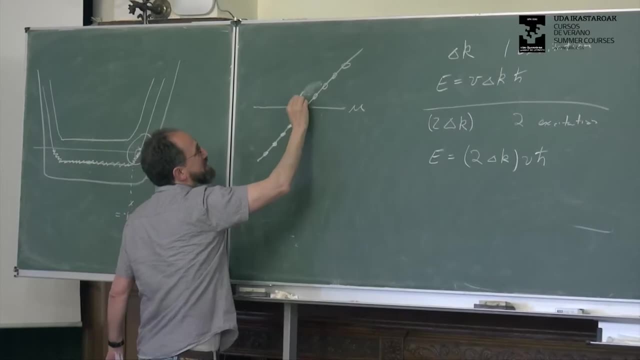 So now it's 2 delta k, 2 units of momentum And it has exactly twice the energy of the last guy. Or there's something else I could have done, which is to push this guy to the left, Which is to push this guy to here. 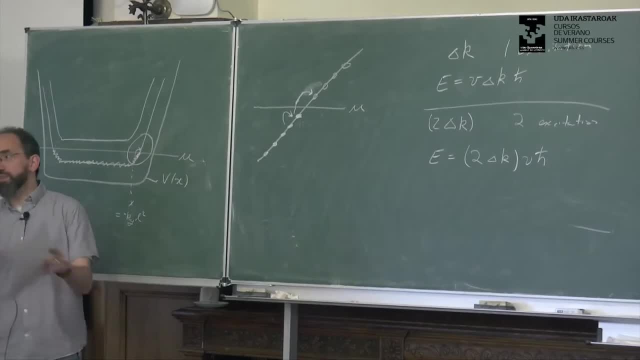 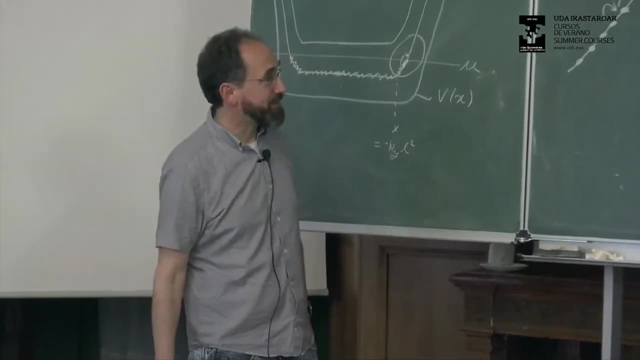 And this guy to here. So push each of two things 1 unit. Or I could have pushed one thing 2 units. Both of these have the same energy and the same momentum, And then we can look for excitations of 3 units. 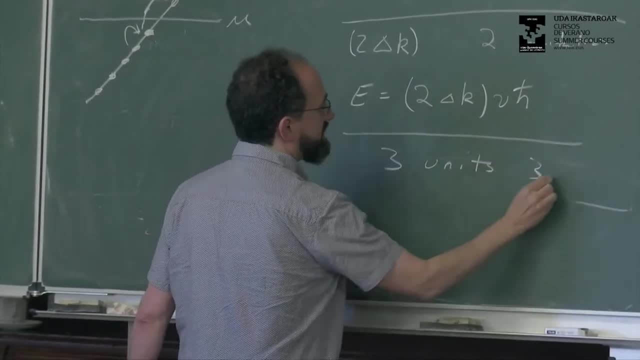 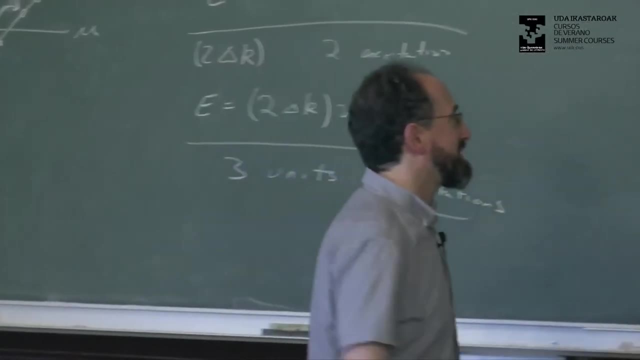 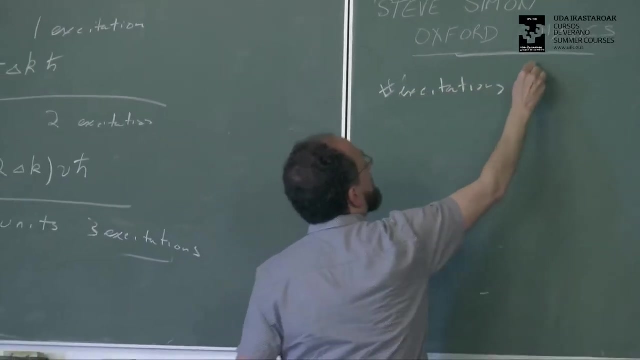 3 units And there's 3 excitations And this gives us a series of the number of excitations at number of units. So number of excitations will make a table Number of units. So there's 1 excitation at 1 unit. 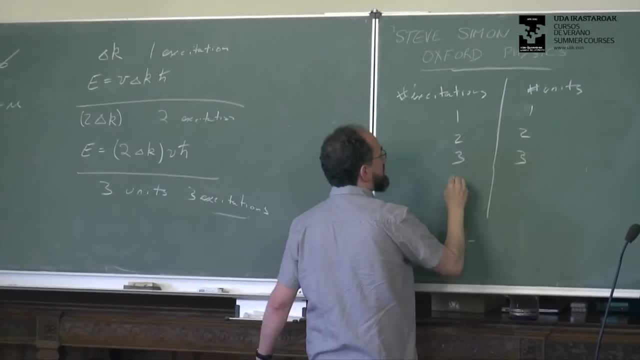 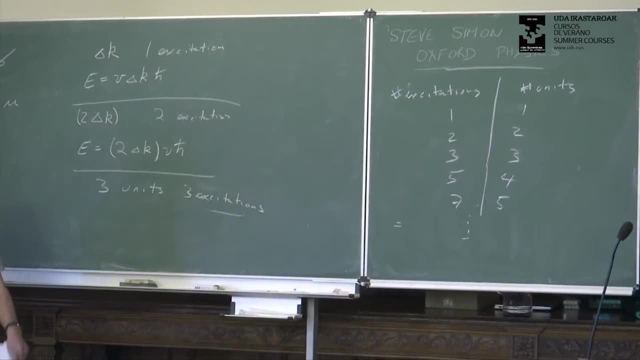 2 excitations at 2 units, 3 excitations at 3 units, There's 5 excitations at 4 units And 7 excitations at 5 units, And so forth and so on, And the exercise which you're supposed to do for homework. 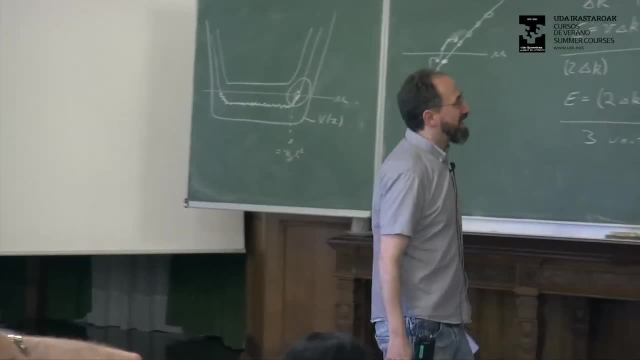 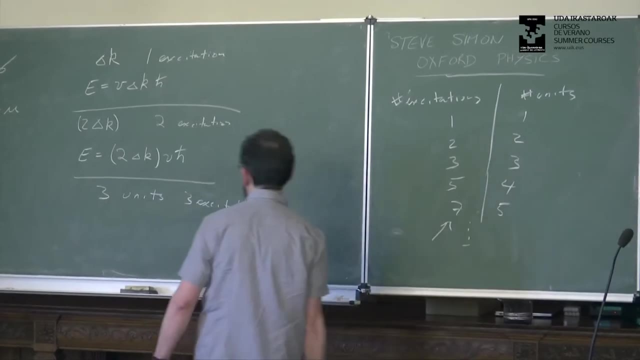 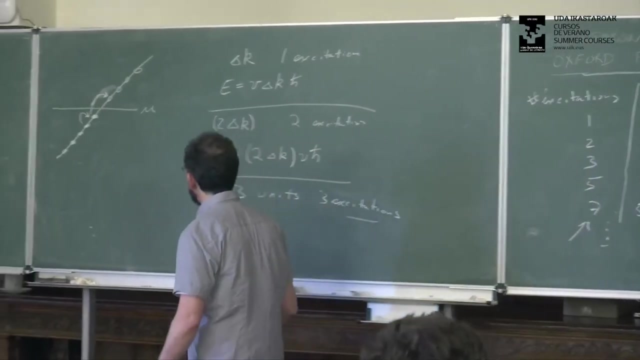 again look up the homework assignment. to give you a hint is to show that this series is a series that describes the number of partitions of the integer over here. So let's give you a hint here. So the partitions of 4, we can write out the partitions of 4 in the following way: 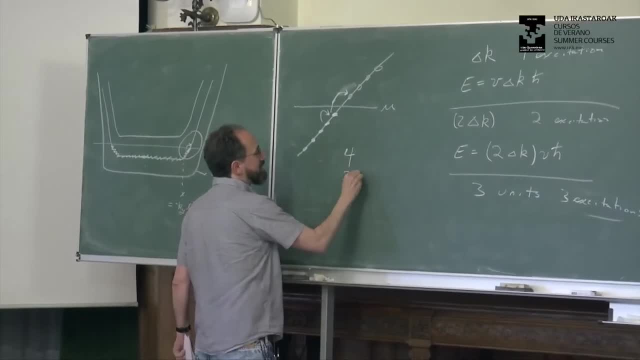 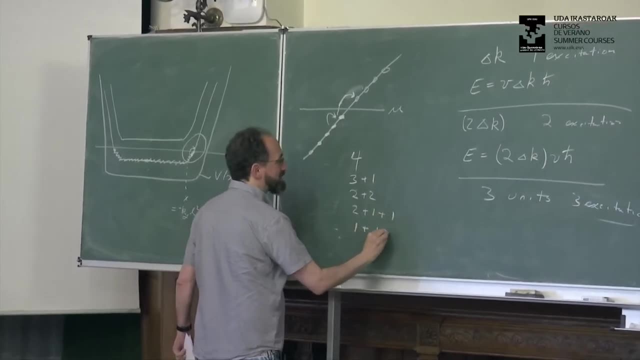 So 4 can be written as 4.. It can be written as 3 plus 1.. It can be written as 2 plus 2.. It can be written as 2 plus 1 plus 1.. Or it can be written as 1 plus 1 plus 1 plus 1.. 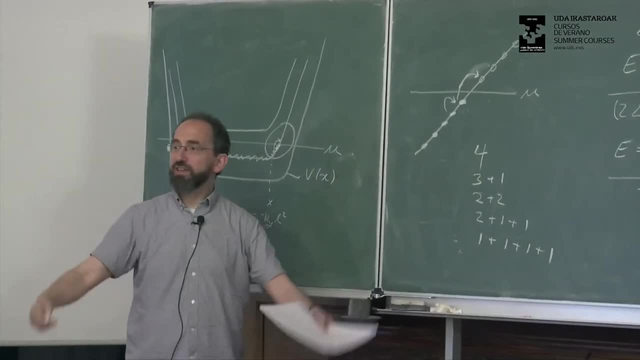 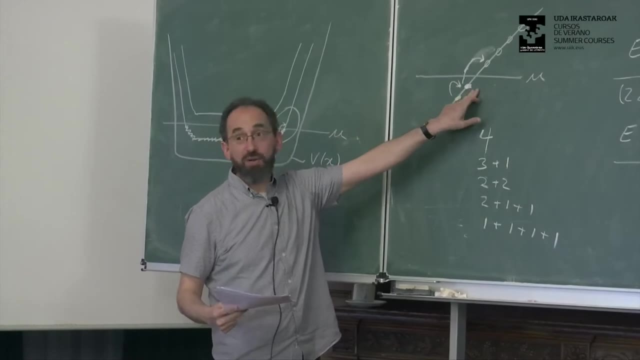 OK, And actually to sort of give away the secret of why these things are there and why these things are the same. if I want to have 4 steps, one thing I could do is I could take one guy, push him 4 steps. 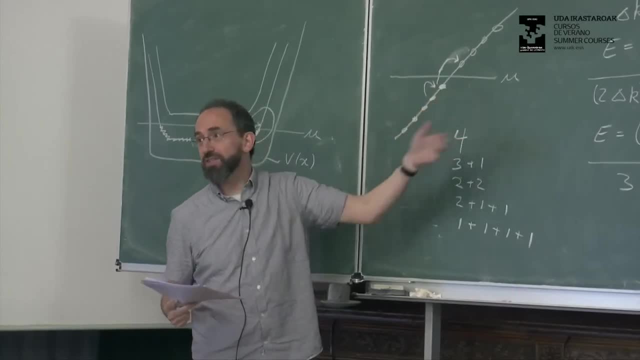 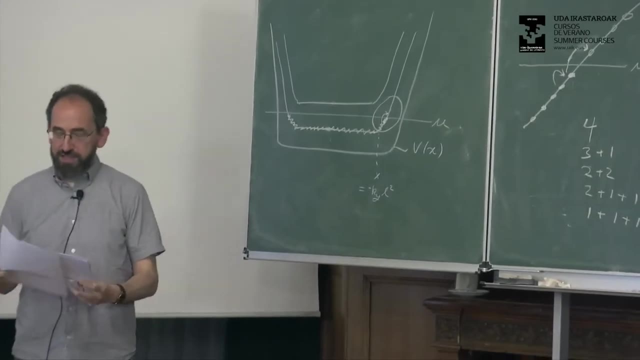 or I could take one guy, push him 3 steps, then another guy push him 1 step, and so forth. OK, And that's why we're looking at partitions of integers. OK, Now, I was going to save this for later in the afternoon. 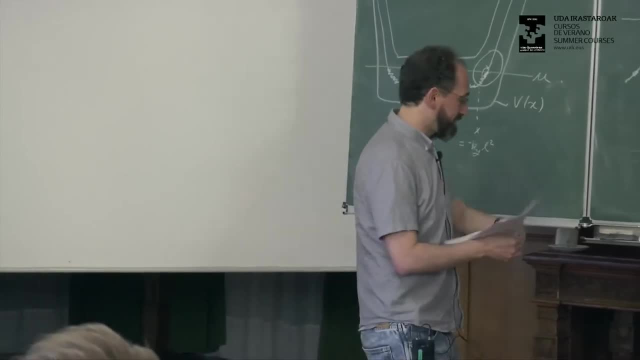 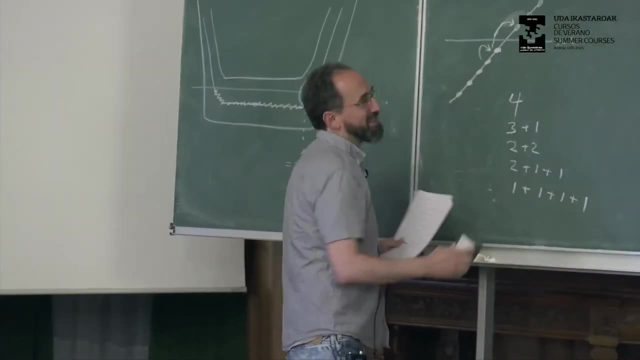 but maybe I'll do it now because it's- Oh my gosh, I only have 15 minutes left. OK, All right, Let me do it now anyway, because Charlie was talking about this earlier and Modi will probably want me to do it. 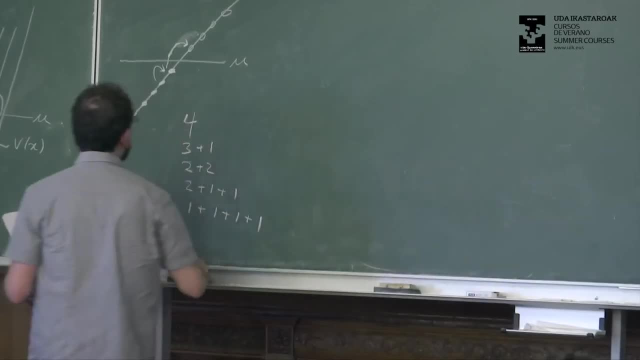 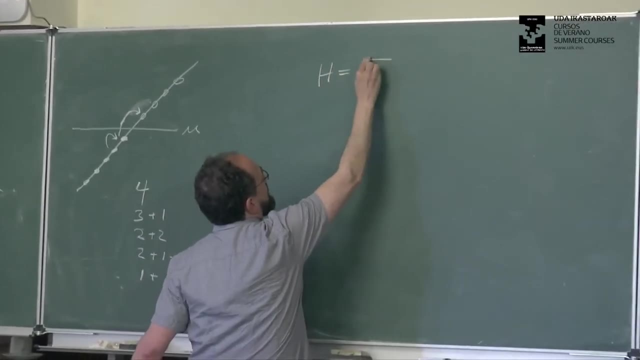 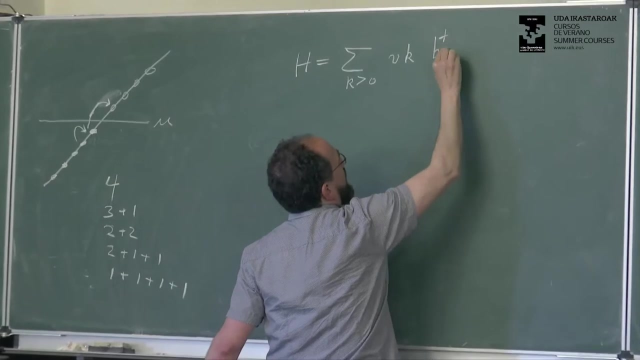 so I'll do it anyway. We'd like to. Charlie promised us that we can write a Hamiltonian for bosons in the following way: k greater than 0, v times k, and then this b dagger, k, b, k, where the b's are bosonic operators. 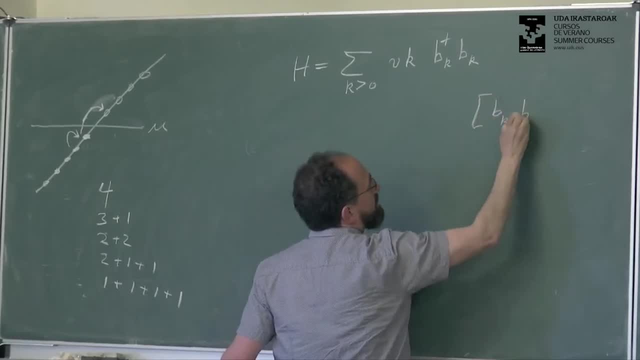 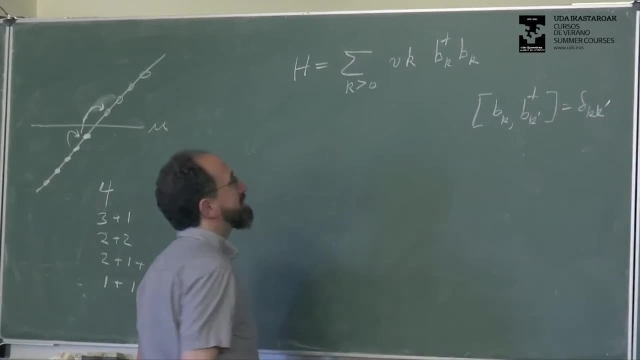 in the usual way: b k b dagger k prime equals delta k k prime. OK, I guess he had a plus 1 half, but I'm going to throw those out. the zero-point energy, just write it like this: 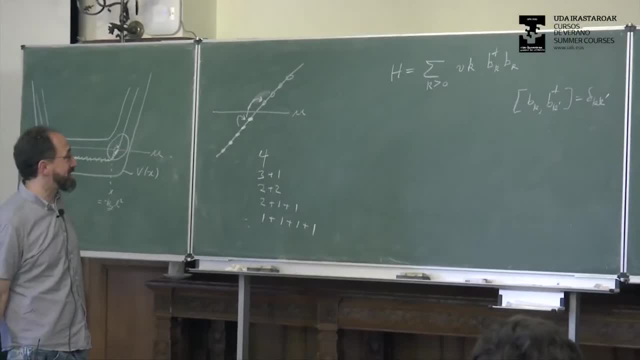 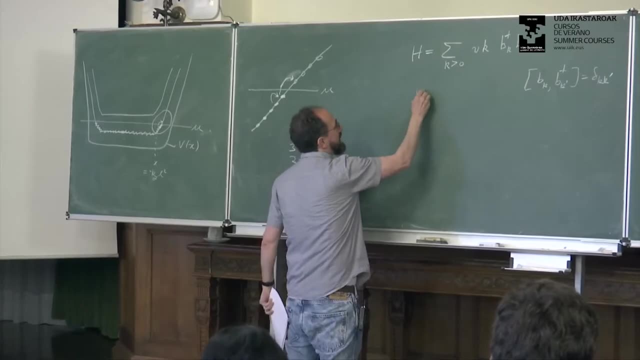 This is like a phonon, a set of phonon excitations, and if we look at the excitations here, the ground. Well, OK, in this bosonic language we have a zero state. That's going to be the ground state. 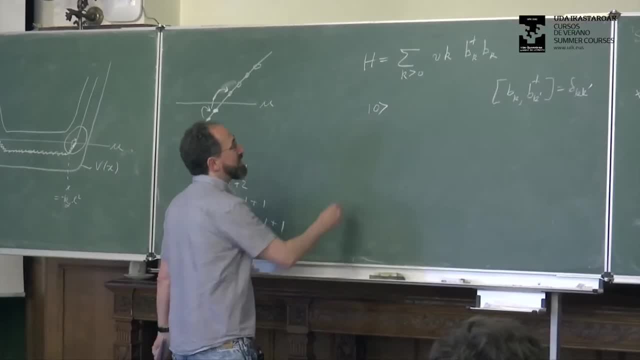 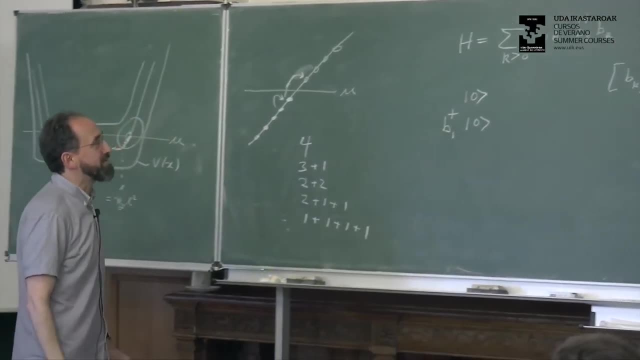 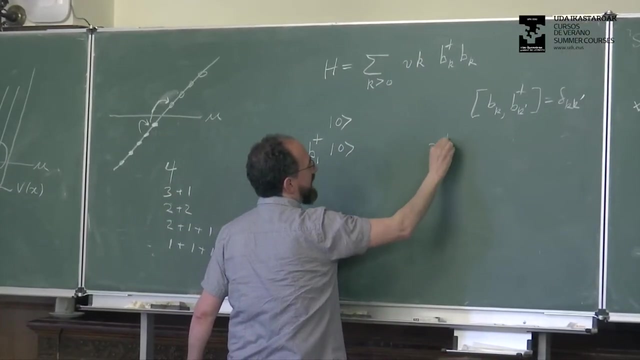 No bosons. OK, We can look at excitations of one unit, which would be b dagger 1 on 0, the lowest This is one unit of energy and it gets. Its energy is v times the minimal k. We'll call it delta k. 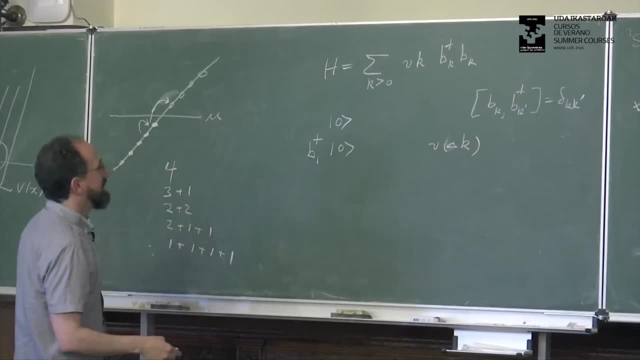 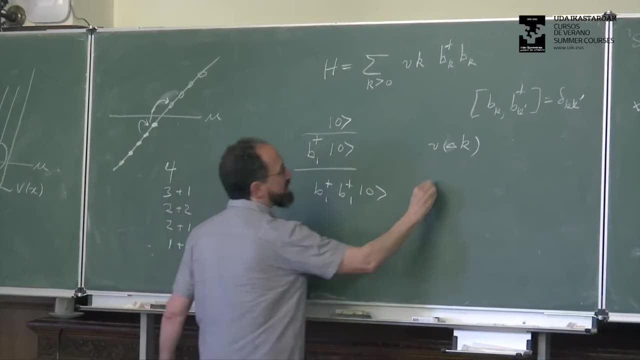 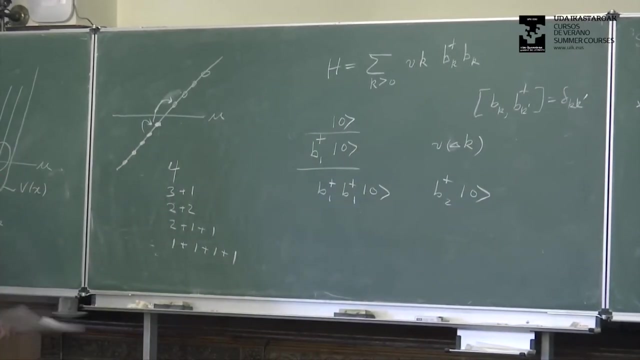 This, just like it was over here, At two units. we could do b dagger 1, b dagger 1 on 0, or we could do b dagger 2 on 0. And these things have exactly the same energy and they both have the same momentum as well. 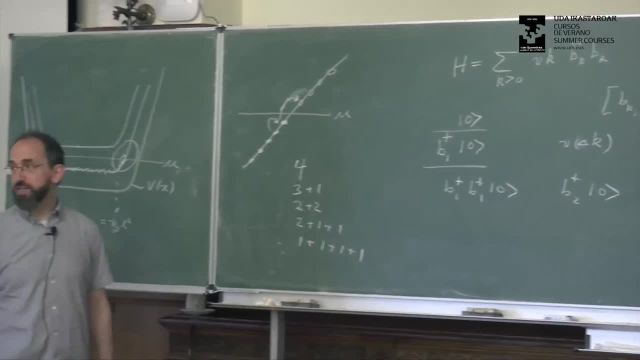 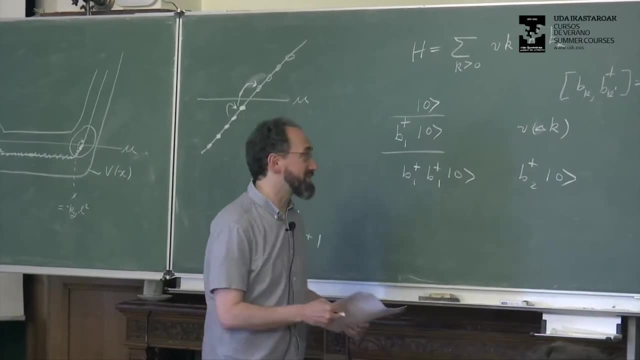 Two steps in momentum and two units of energy. This one gets two units of energy because it's two excitations of one unit, and this one gets two units of energy because it's one excitation of two units. And you can keep going. 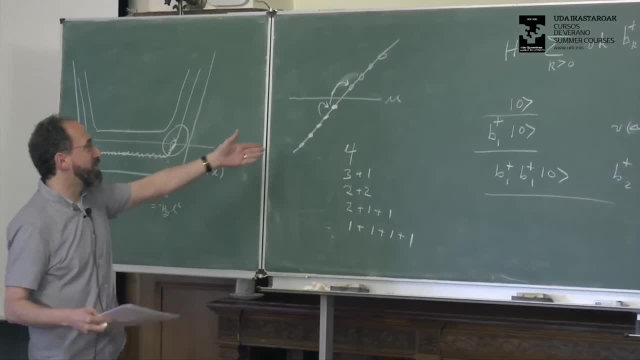 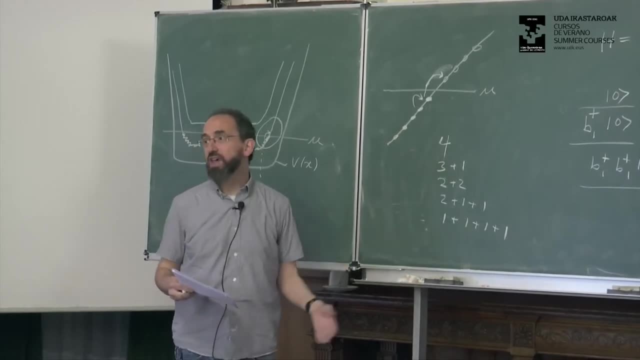 and it's pretty easy to see that if you go up to four units there's four different ways to make excitations. You make b dagger 4 or b dagger 3, b dagger 1, and so forth and so on. So this, you know, sort of gives some flesh. 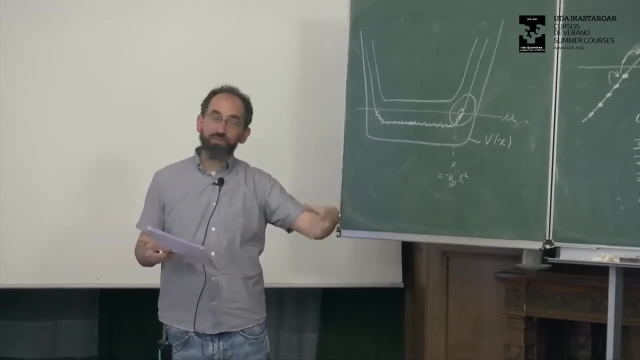 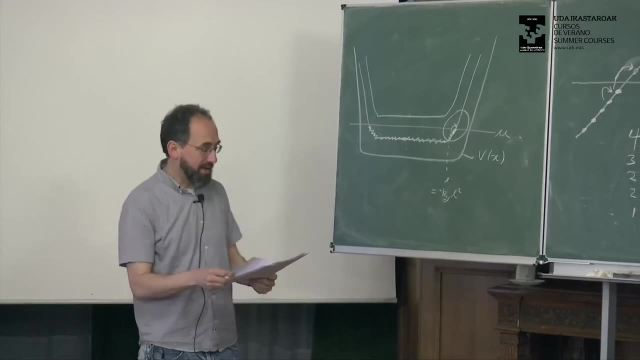 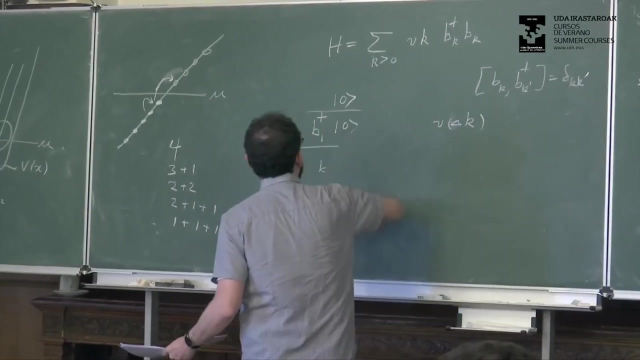 to the mapping between the boson, you know, counting number of boson excitations and counting excitations of fermions on the edge. Okay, All right, Let's see how far we can go here in trying to understand why it is that we have. 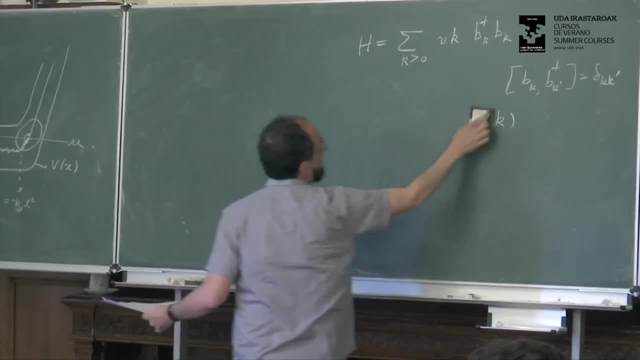 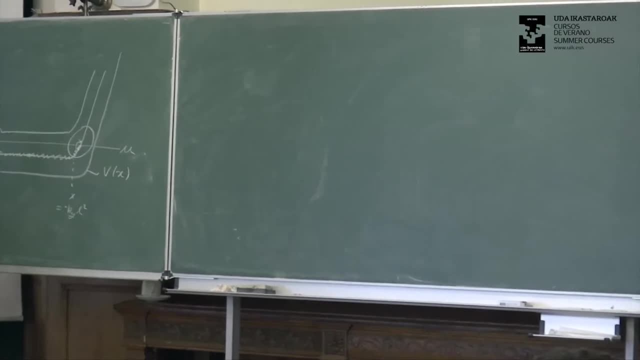 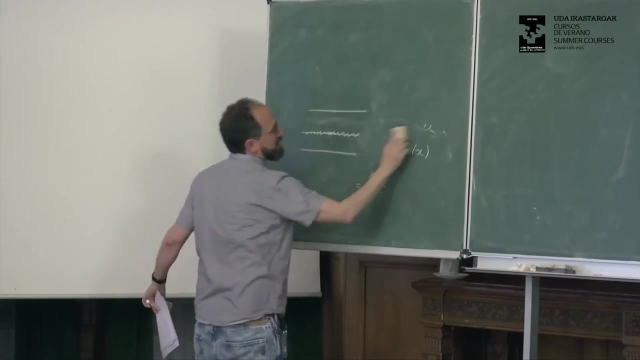 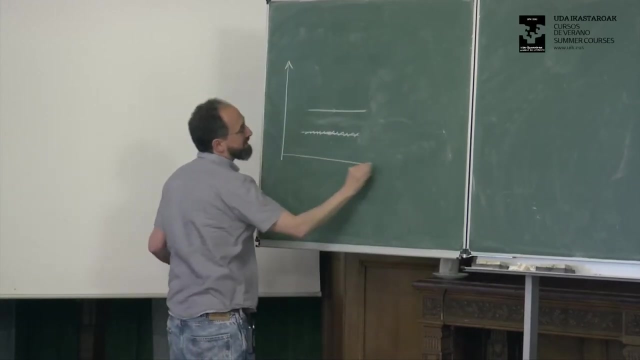 such nice quantization of Hall conductance. So back to this picture here, and I'm going to ignore the edges now for a second- We're back to our Landau levels like this. So we have our energy and density of states like this: 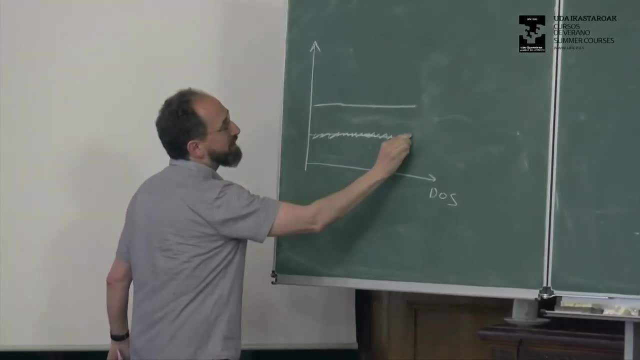 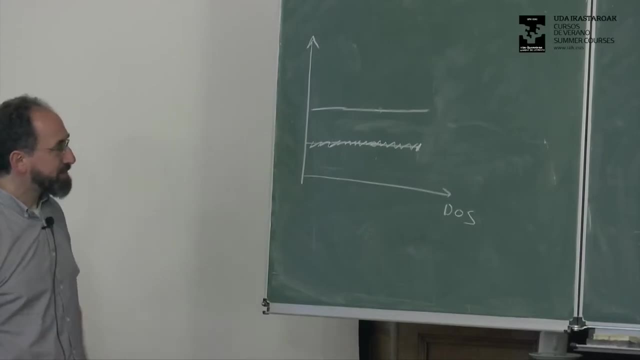 And at exactly nu equals 1,, we filled one Landau level and then there's an h bar, omega c gap to the next Landau level And if we had exactly one filled Landau level, we have a really good insulator. 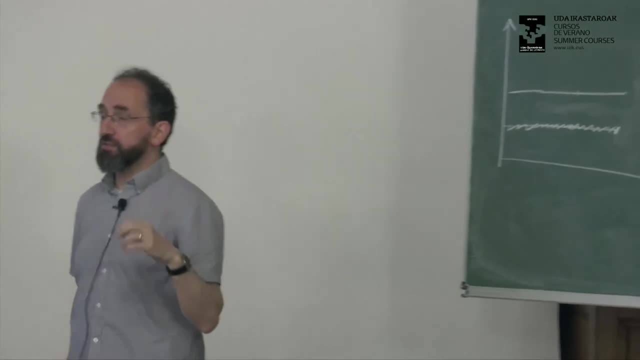 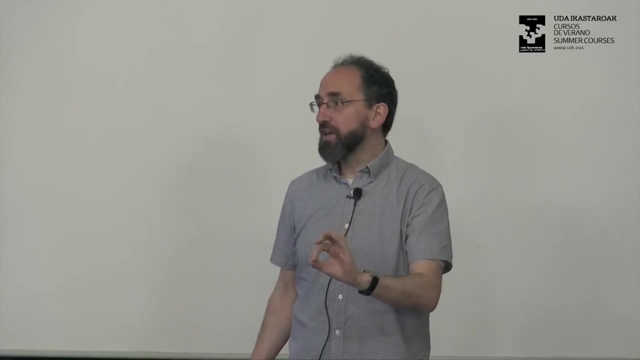 because there's a gap to the next excitation. Now in materials, the kind of thing that many of you think about. it's not unnatural to have exactly one electron per unit cell. That sometimes happens, However, in quantum Hall effect. that's really very fine-tuned because if you change the magnetic field just a little bit, it changes the degeneracy of a Landau level and you'll add either extra electrons or extra holes And you have to tune the magnetic field extremely precisely to land right here. 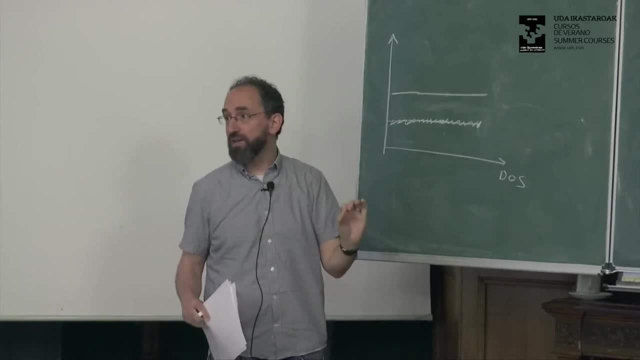 So only at one exact magnetic field do you have nu exactly equal to 1.. So you have really an insulator only at one precise magnetic field, And if you go to a slightly lower magnetic field you start filling the next Landau level with a slightly higher magnetic field. 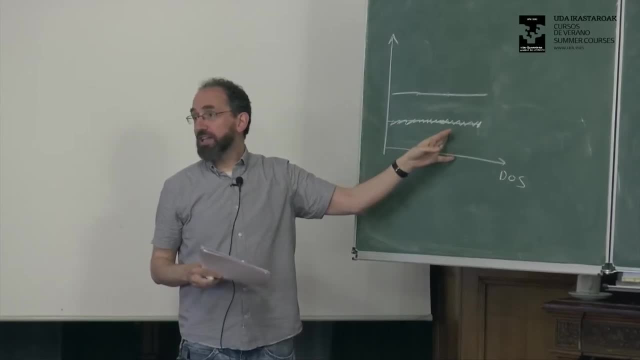 You start putting holes in the lower Landau level. So generically, in fact, this thing isn't an insulator at all. Once you have electrons up here or holes down here, you have low energy excitations and things can move around. 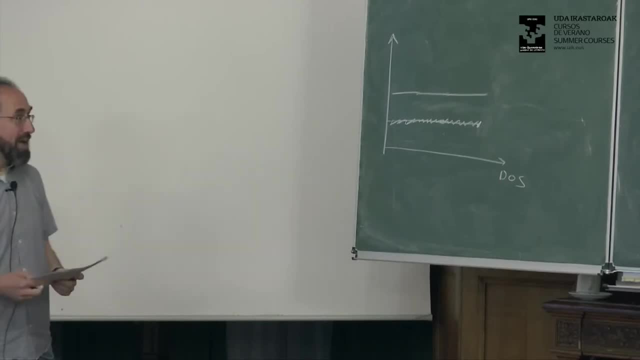 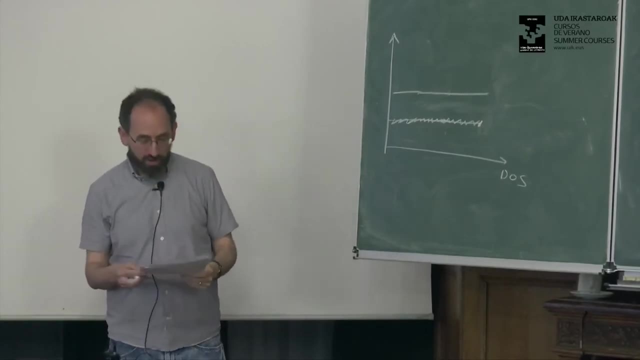 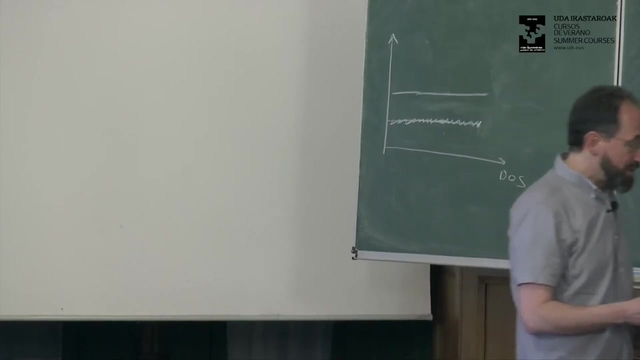 and then you have a problem. So we need some way to understand. why is it? in the experiment we see plateaus in the Hall conductivity and we see zeros in the longitudinal conductivity. So previously, when we were discussing this, we said: well, let's just set the chemical potential. 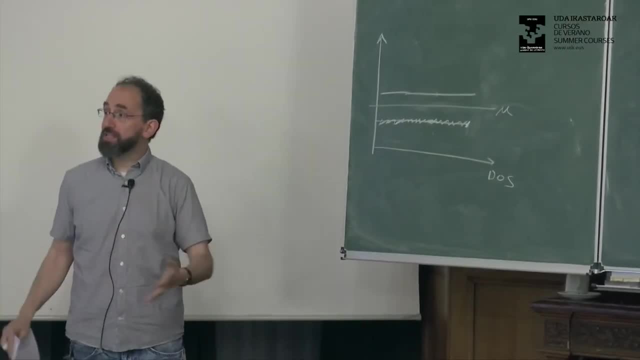 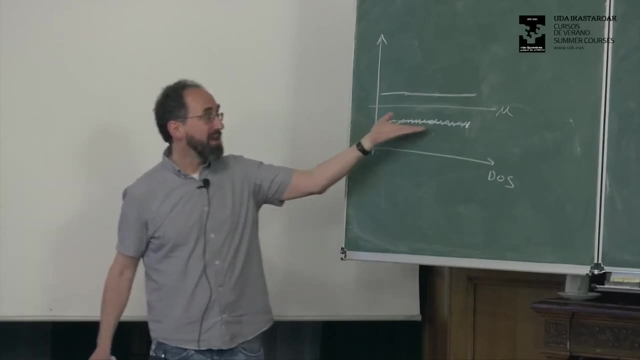 in between the Landau levels. But in the actual experiment this is not what you do. What you actually do is you fix the electron density and you tune the magnetic field and the chemical potential will jump instantly from being down here to being up here. 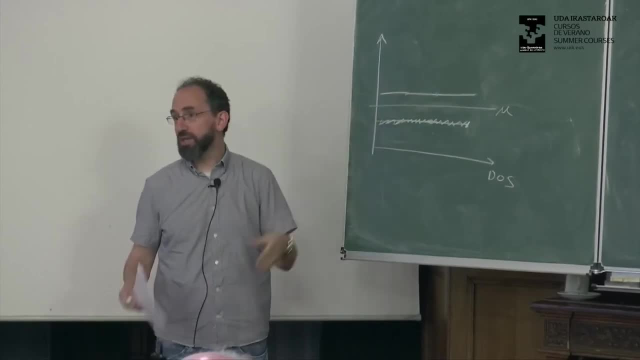 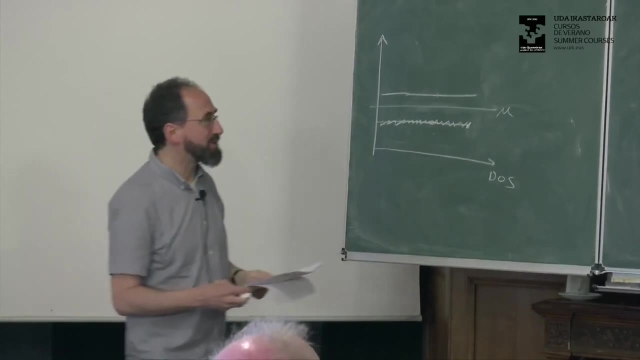 So you can't very easily tune the chemical potential in between Landau levels generically. So what's going to save us here and enable us to have actually quantum Hall plateaus? What's going to save us here is disorder. So we have to understand the effects of disorder. 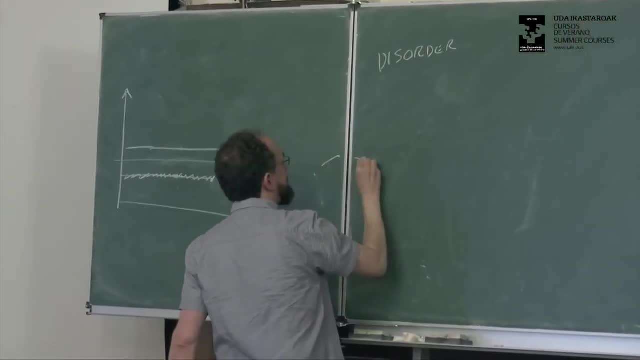 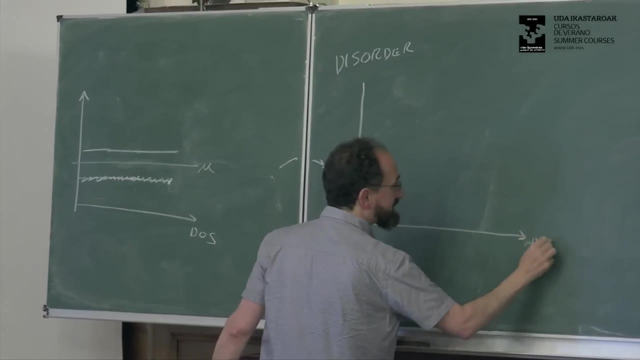 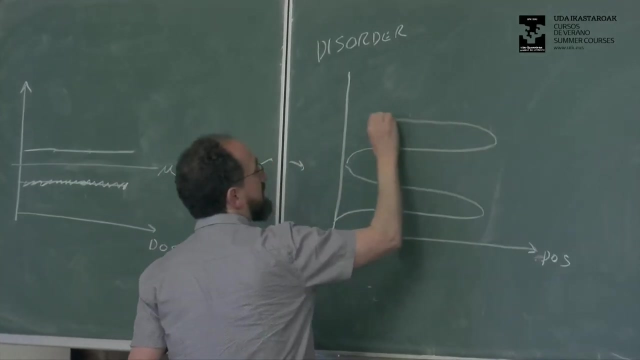 So, instead of the density of states looking like this, the density of states will now look more like this: This is density of states, And each of these bands gets spread out into wider bands like this, And the reason for the spreading is that when you have a disordered system, 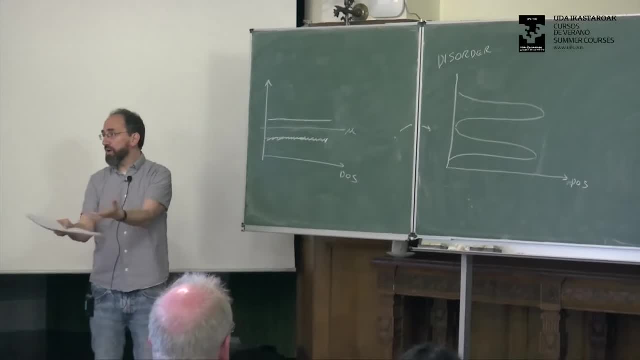 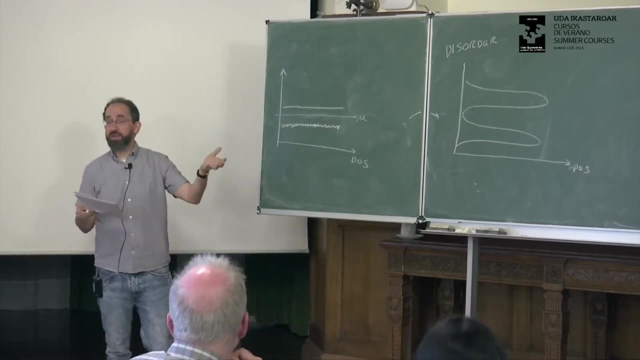 some eigenstates will be in an area where there's lower potential and some eigenstates will be in an area where there's higher potential. So some of these eigenstates get pushed down in energy and some of the eigenstates get pushed up in energy. 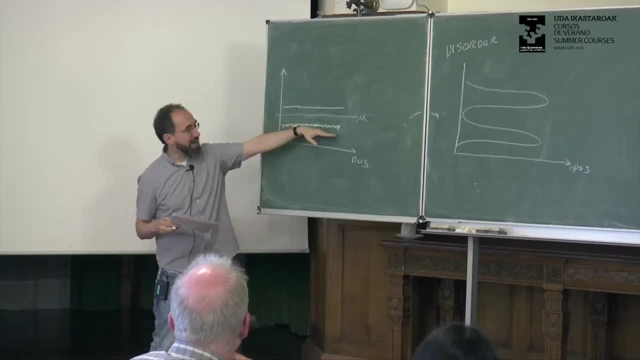 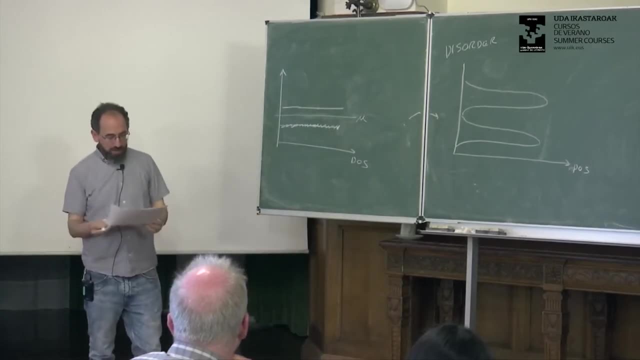 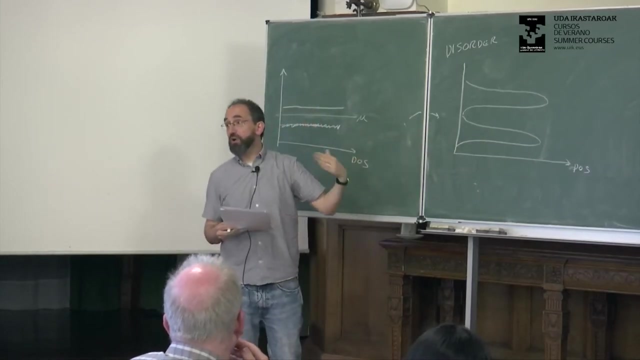 So, instead of having a flat band where everyone has exactly the same energy, you now have a spread of energies. Now, further than just spreading out the energies like this, in fact, what you also do is you localize many of the eigenstates. 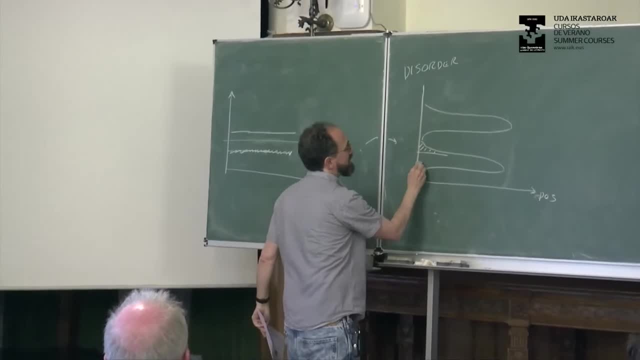 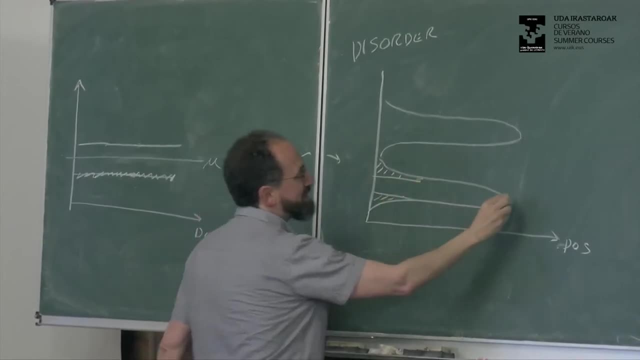 and particularly the eigenstates in the band tails, are certainly going to be localized, And then we can argue about how wide these localized regions are and whether there's going to be some extended states in the middle, extended and then localized on the edges. 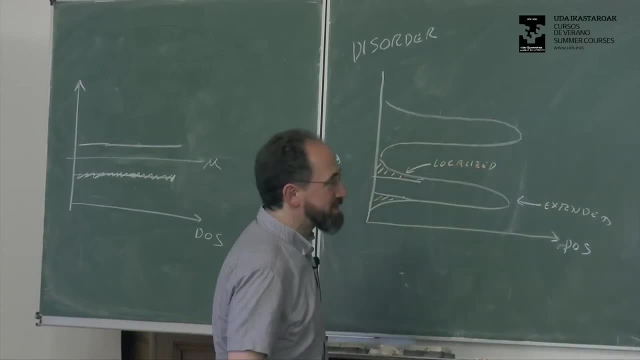 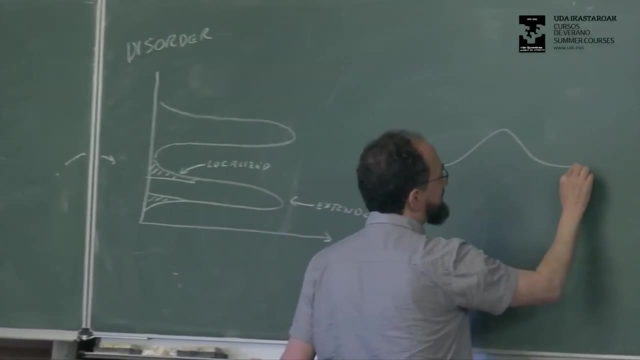 Why is this? Well, there's various ways to think about this, but let's think about, sort of in a semi-classical picture, where there are some hills and there are some valleys in the potential, like this, And if you think about an electron, 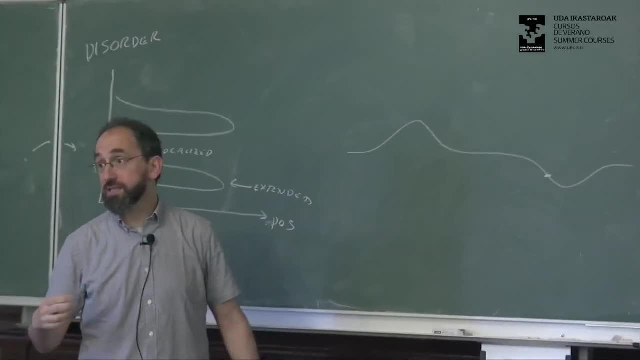 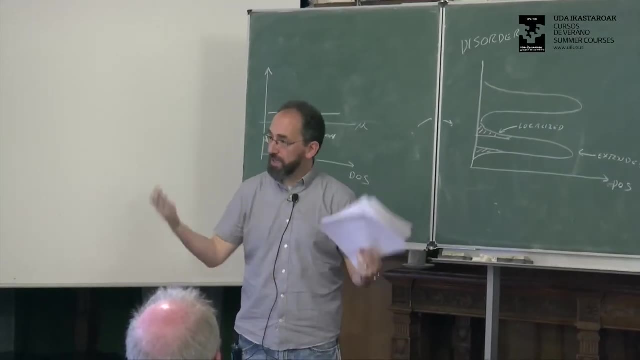 living in this valley, or an eigenstate living in this valley. what does he do? Well, he's an electron living in a potential, and we know from our previous discussion that when an electron lives in a potential, in a magnetic field, he travels perpendicular to the potential. 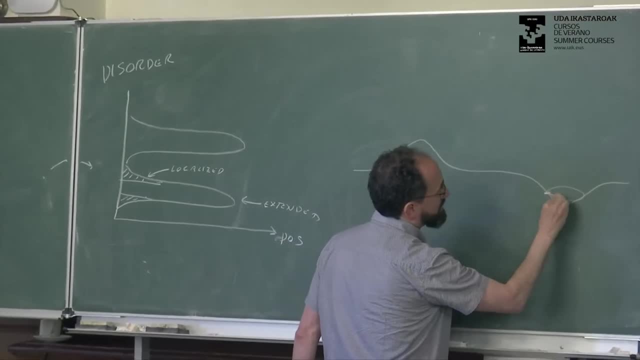 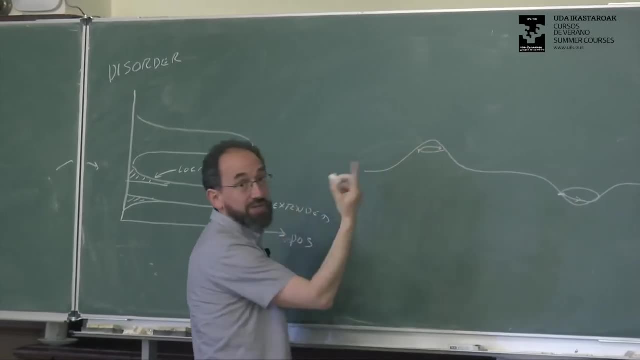 So he's going to actually run around sort of in a circle around the minimum of this valley And similarly, an electron up here is going to run around in a circle around this maximum. So, instead of being these nice straight lines that we had when we solved the problem, 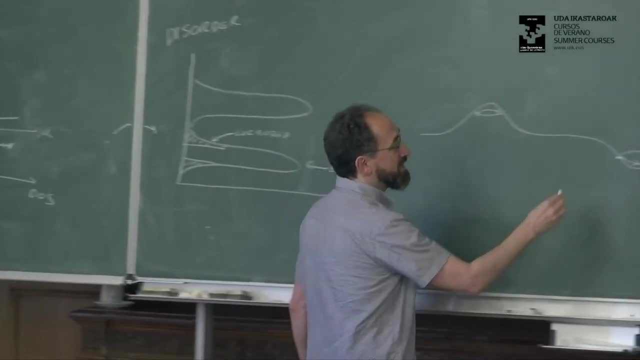 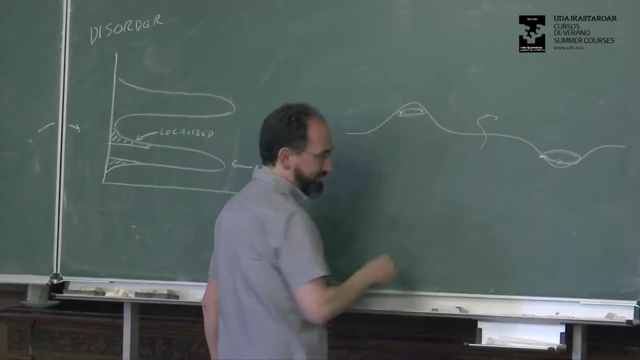 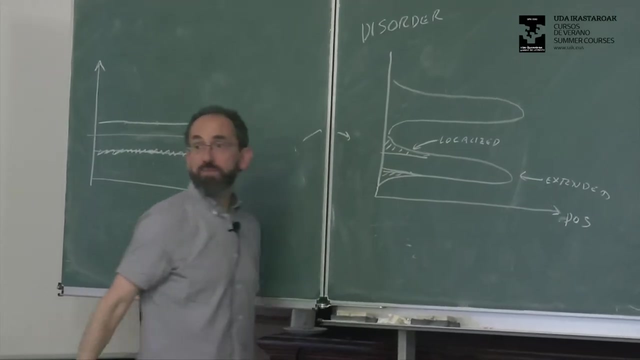 in Lando gauge we'll have localized states, sort of stuck or trapped in these minima, or trapped in these maxima, And somewhere in the middle there will be electrons that go throughout the system, sort of living at the intermediate energies. Okay. 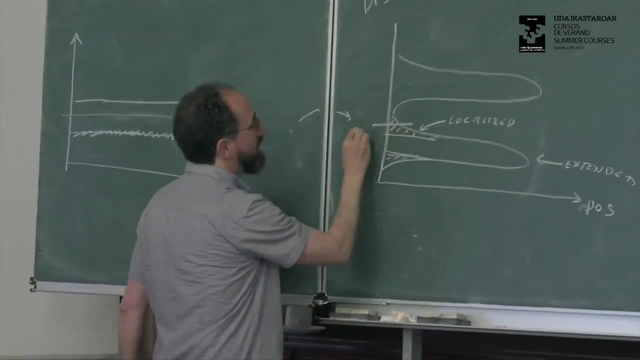 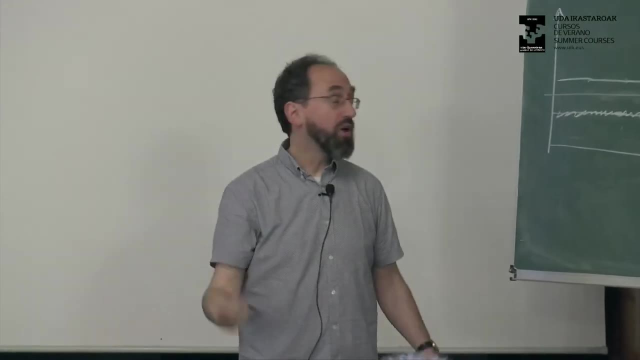 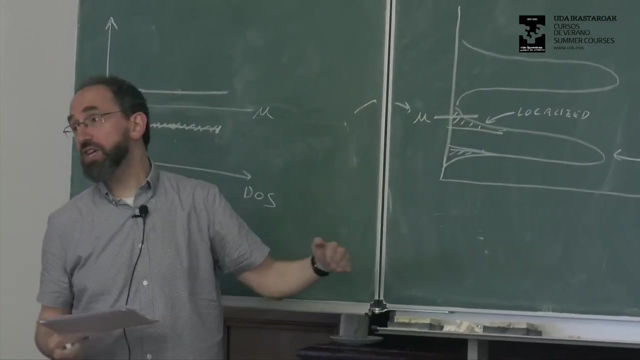 So now, if you put our chemical potential or our number of electrons somewhere within the localized band, we can then change the number of electrons a little bit, or change the magnetic field a little bit, as the chemical potential stays in the localized states, and that's not going to change. 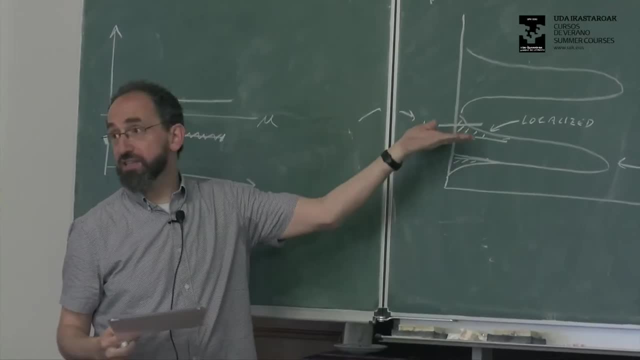 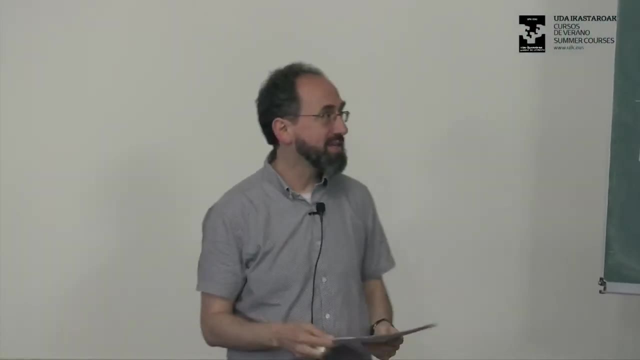 the conduction properties at all, because you're just adding electrons into localized states and the localized states don't participate in any of the conductivity, They just sit there. That's what it means to be localized. So the point here is that by adding disorder to the system, 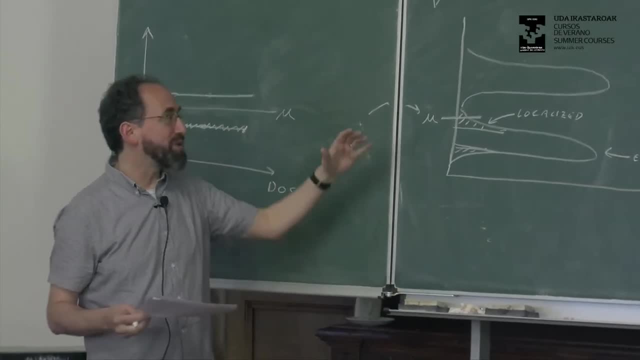 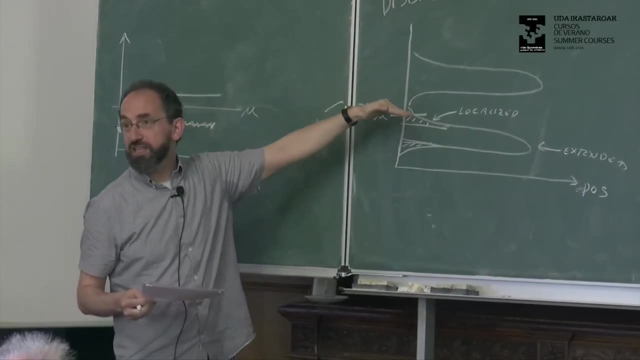 and putting your chemical potential in the localized states, you've managed to sort of preserve the properties of these extended states for sort of a longer period, over a region of changing the chemical potential or the density of electrons And at least within a range of filling fractions. 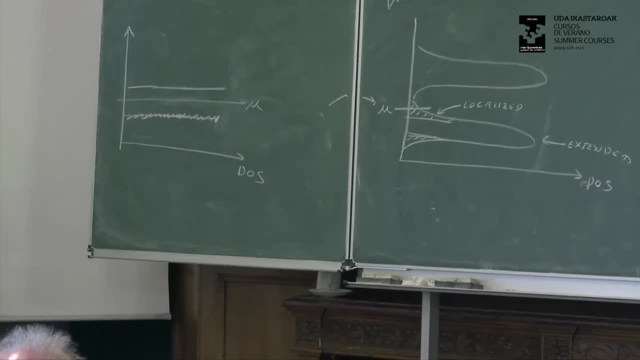 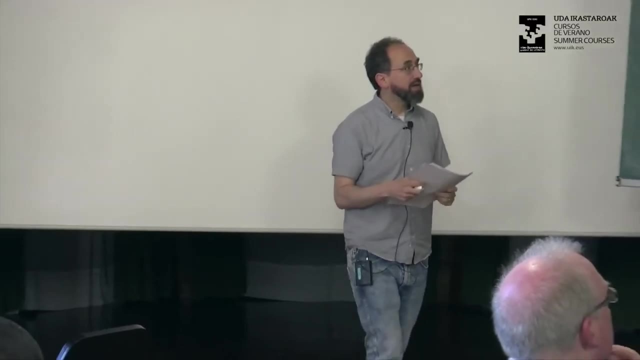 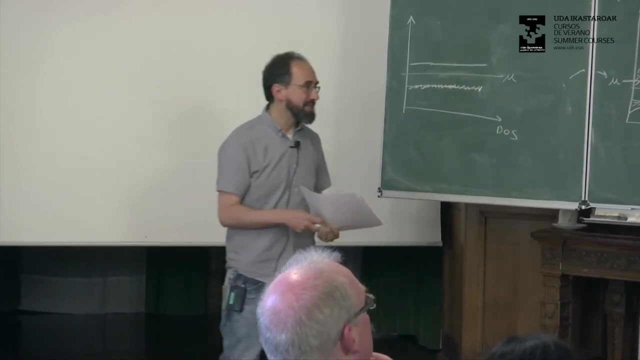 you'll have the same conductivity properties. Okay, Does that make sense? Everyone good with that. Okay, So we still need a reason why the conductivity is quantized so precisely to one part in 10, to the tens. We need sort of a strong principle. 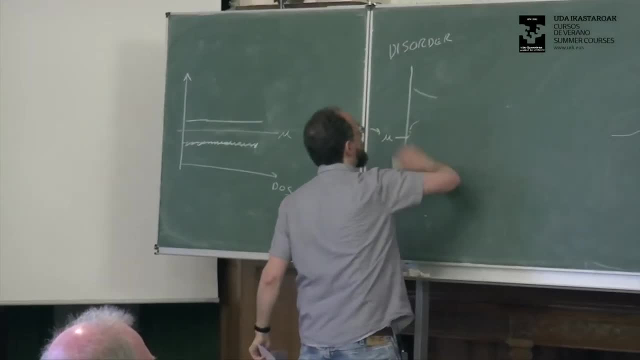 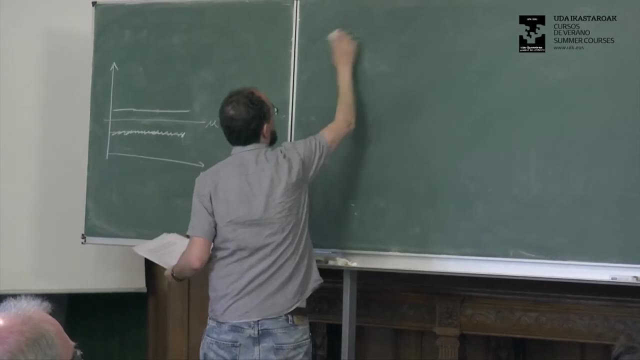 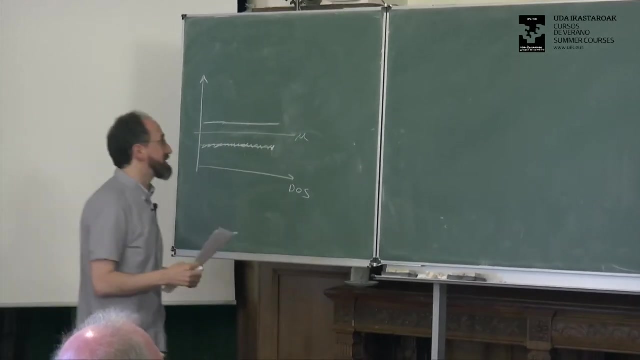 and the strong principle I mean. so Charlie already gave the you know the rough Laughlin argument, but the strong principle that we need to mention is that it's really what protects the integer. quantum Hall conductivity is actually gauge invariance And this was something that was realized. 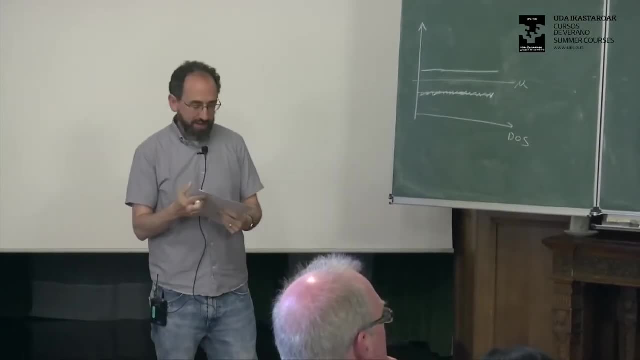 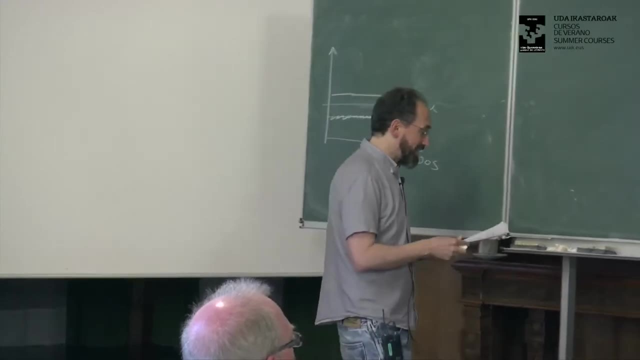 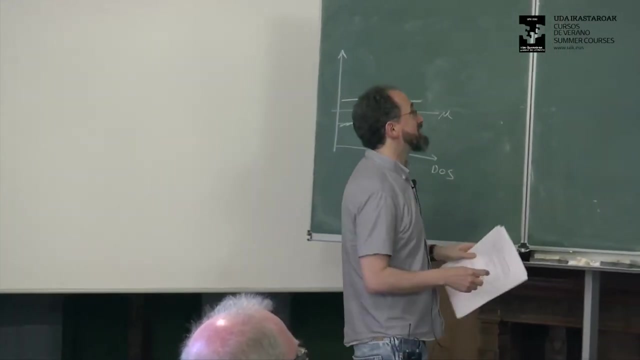 by Bob Laughlin shortly after the discovery of the integer quantum Hall effect, that if you need something to be quantized extremely precisely, there has to be something extremely strong which is preserving it. And the key theorem which Laughlin used is known as the Byers-Yang theorem. 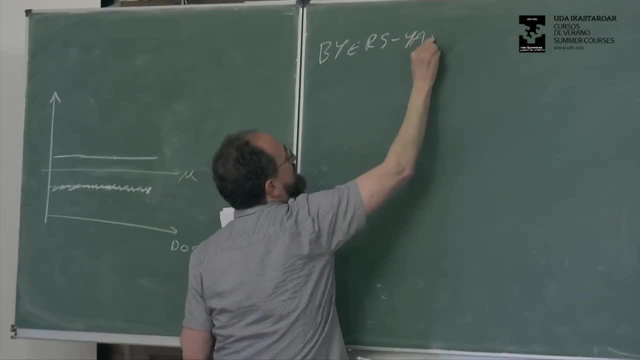 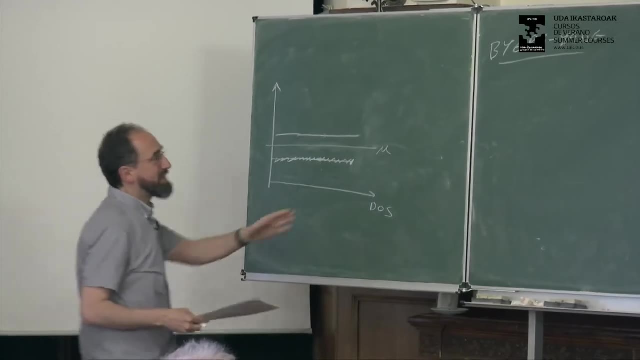 Byers-Yang, which I believe was from 1961. And it's a bit of an extension of the Aharonov-Bohm effect, which you might be familiar with. So Yang is CN Yang, the guy with the Nobel Prize. 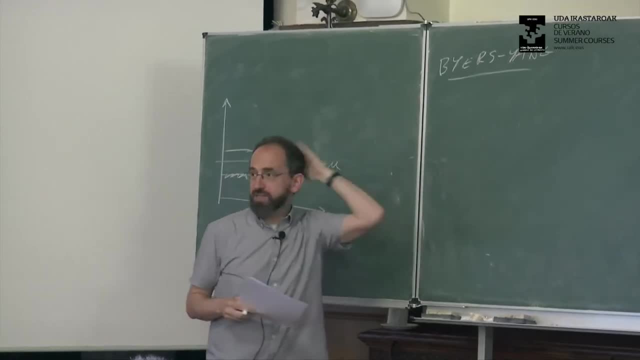 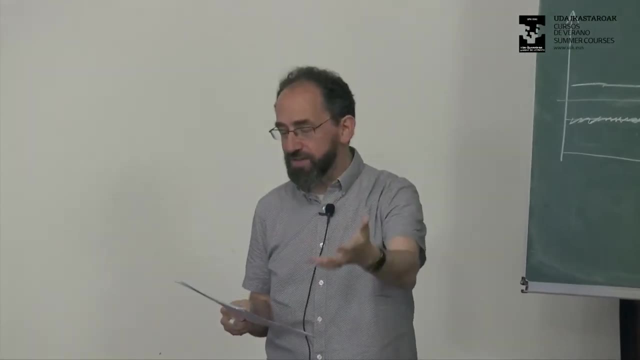 for parity, breaking in weak interactions. Byers is Nina Byers, who is actually. she was a member of my college at Oxford for a long time but eventually ended up in the early 70s at UCLA where she spent the rest of her career. as a nuclear physicist- Although she did. she passed away just a couple years ago, but she told me personally that she always thought it was a huge mistake to have left Oxford because she loved it so much. But anyway, she was at UCLA. 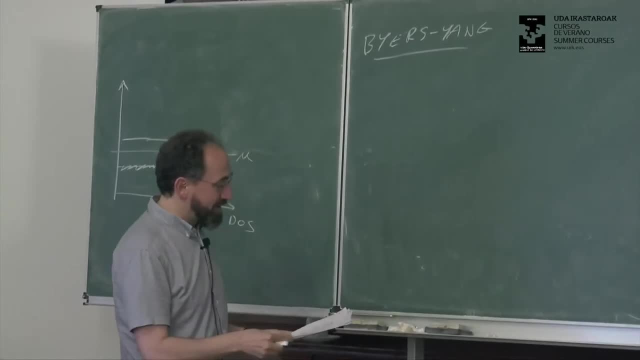 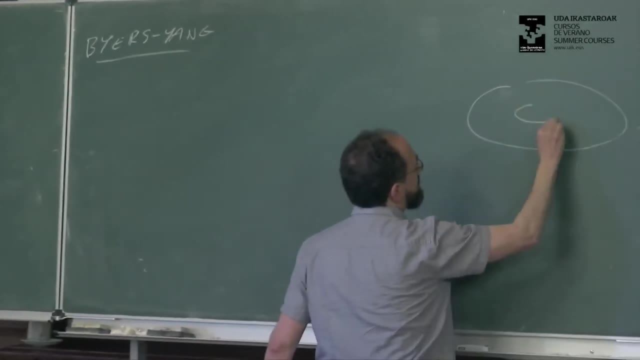 Anyway. so the statement of the theorem is basically is the following: If you take any physical system, I'll draw it as two-dimensional, but it could be a three-dimensional system. You cut a hole in the middle of the system and there could be magnetic fields in the system. 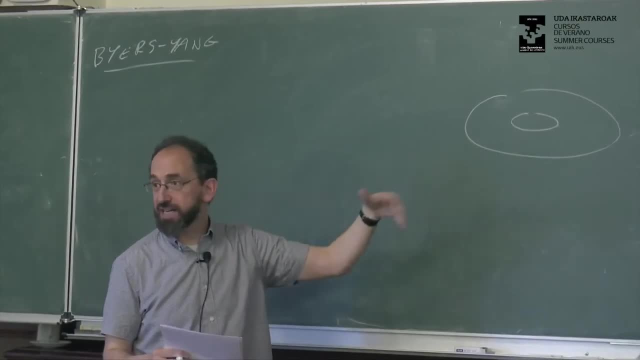 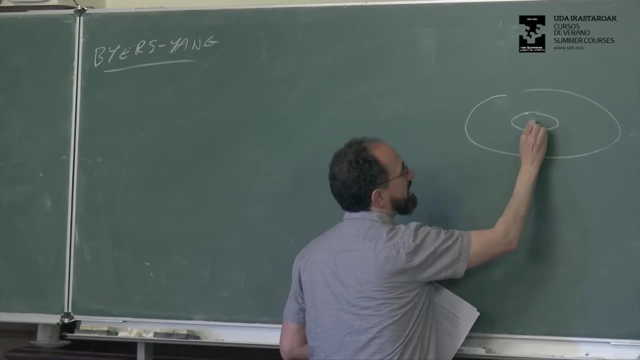 It doesn't matter, You can have any interactions or spin orbit or whatever you want, It doesn't matter. We're going to take this system, cut a hole in the middle of it and we're going to add a flux quantum through the middle. 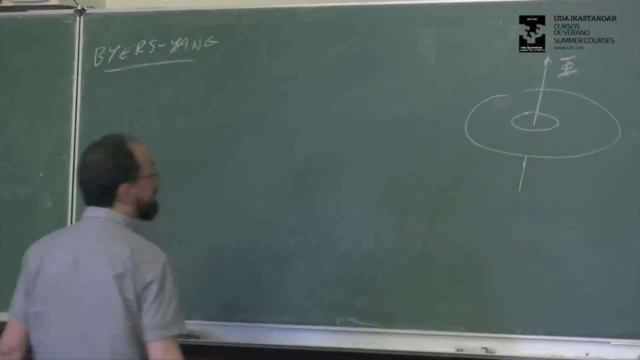 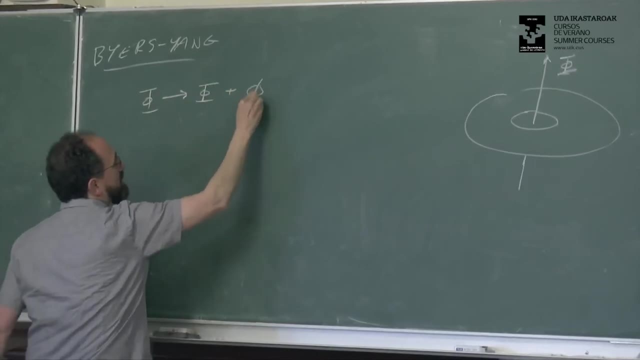 We're going to add some flux through the middle. The statement is the following: If you take the flux and you change that flux by exactly one flux quantum- this flux quantum, remember, was H over E- you add that much flux through the middle. 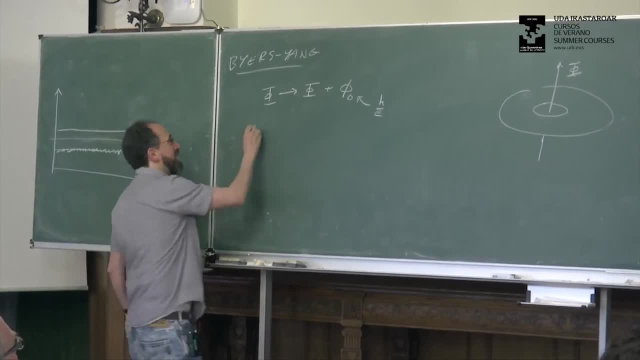 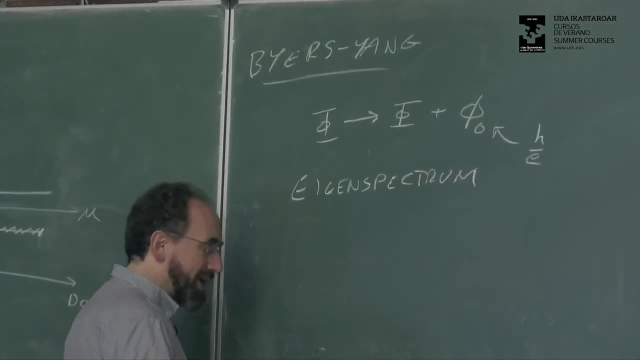 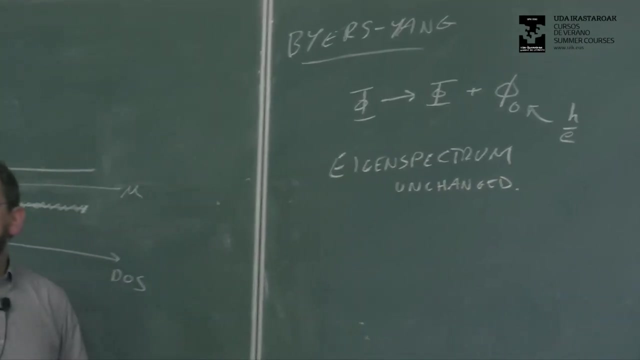 then the eigenspectrum is completely unchanged. Eigenspectrum unchanged, In other words, all the eigenstates and the eigenfunctions are unchanged. to a gauge transform. Okay, And it's actually. it's very similar to the Aharonov-Bohm effect. 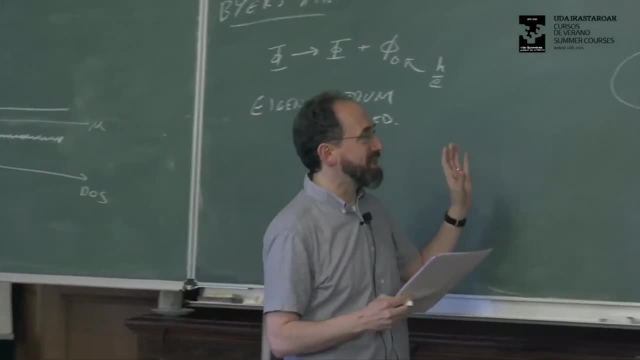 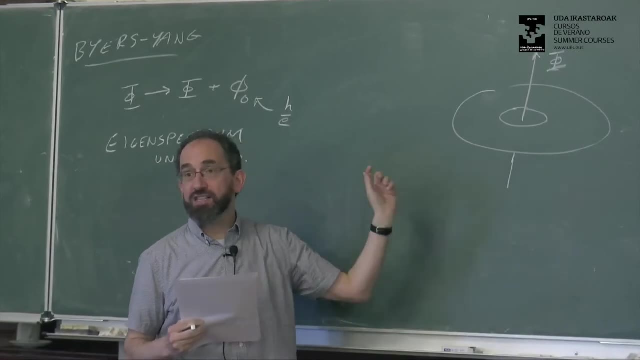 If you remember the Aharonov-Bohm effect. basically, you do something like this: You have some sort of interference around a flux, some amount of flux, and you can see that the flux is there, as long as the flux is not an integer number. 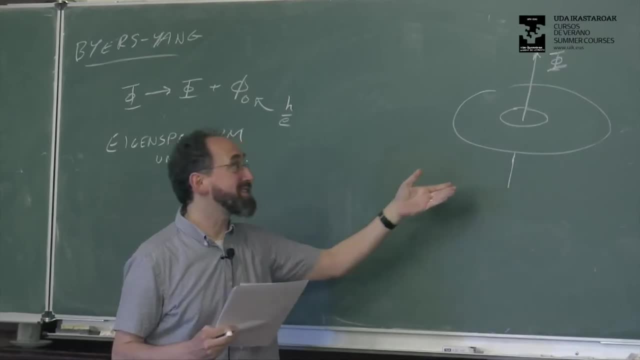 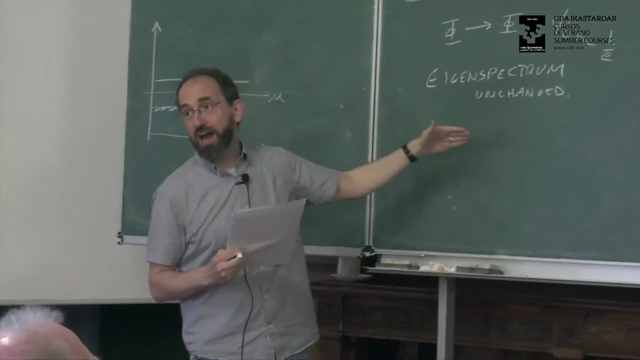 of flux quanta where you can't see it anymore. And this is sort of an upgrade of that statement which says: not only can you not see the flux if it's an integer number of flux quanta in the middle, in fact the entire eigenspectrum. 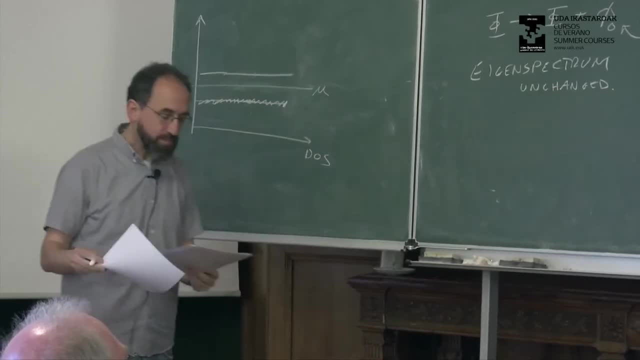 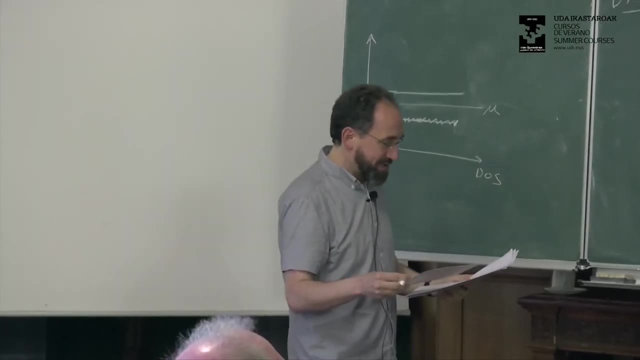 is completely unchanged. Okay, So since I'm down to two minutes, I'll not give the proof of this theorem, just state it. But then, once we have this theorem, we can then do the Laughlin pumping argument. So Charlie did it. 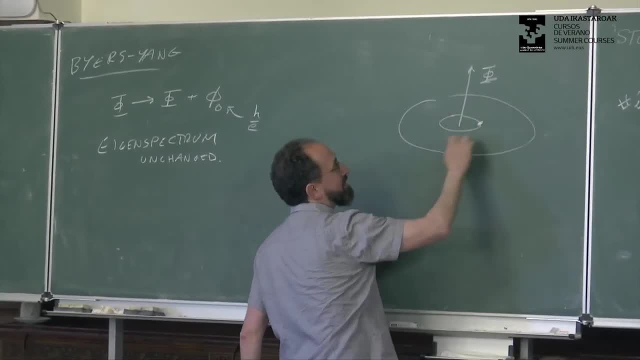 on a cylinder. I'm going to do it on this annulus here, So I'm going to think of this as a two-dimensional system. There's a uniform magnetic field which I'm not going to change. I'm going to leave that fixed. 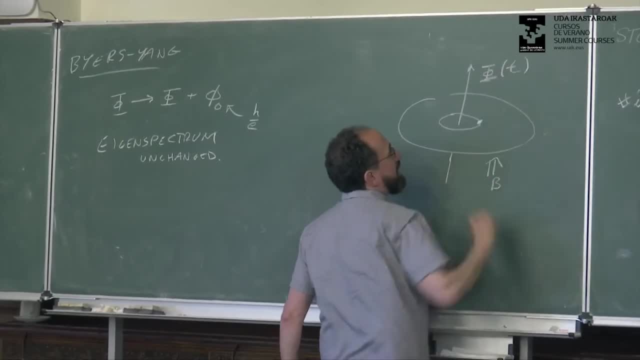 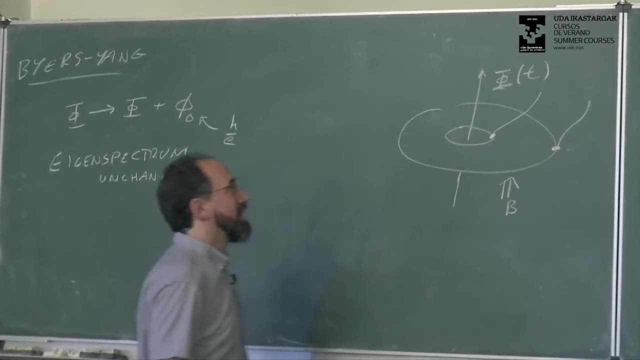 The flux to the middle I'm going to have be a function of time. I'm going to change it adiabatically. I'm going to measure current flowing from the inside to the outside of the disk. Okay, So we're going to start. 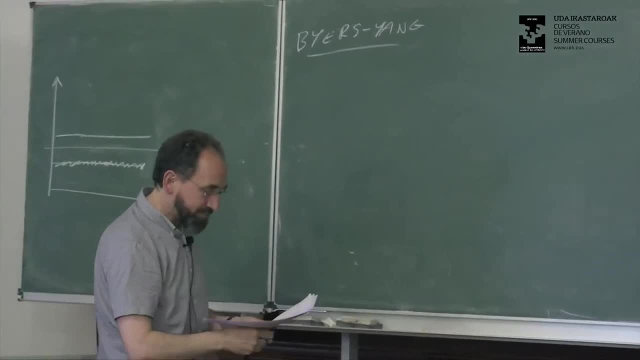 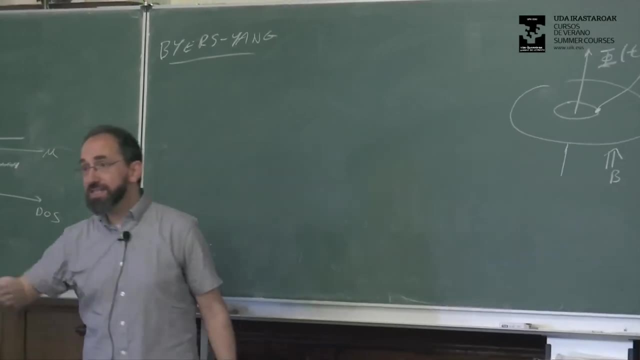 the system in um in the ground state, And then we're going to slowly adiabatically change phi of t And it's going to stay in the ground state the entire way through the, through the process, By keeping the chemical potential. 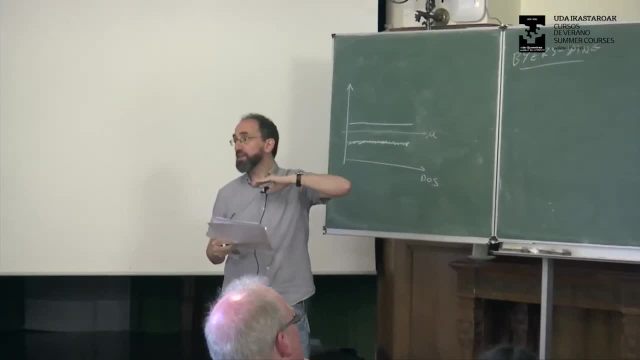 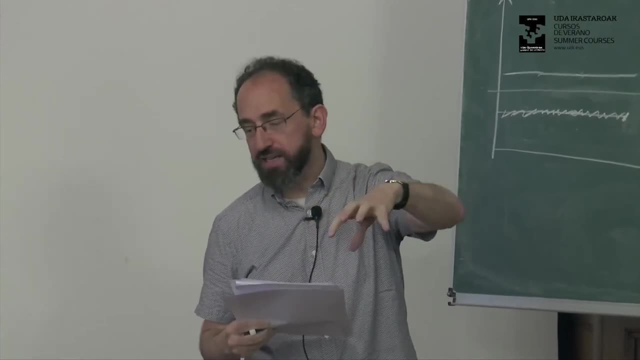 in one of these localized bands. we know that there will be no longitudinal conductivity, There's going to be no dissipation of energy. No one's allowed to carry current in the direction that will dissipate energy, So nothing is allowed to move current. 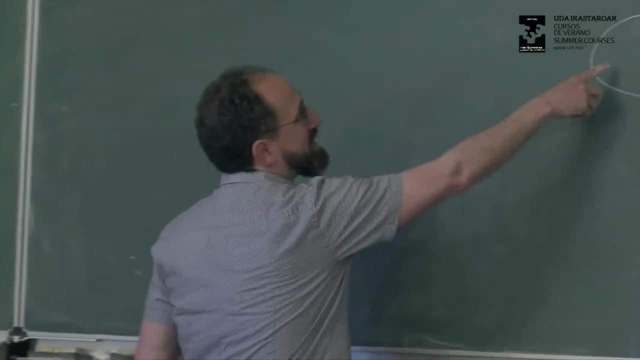 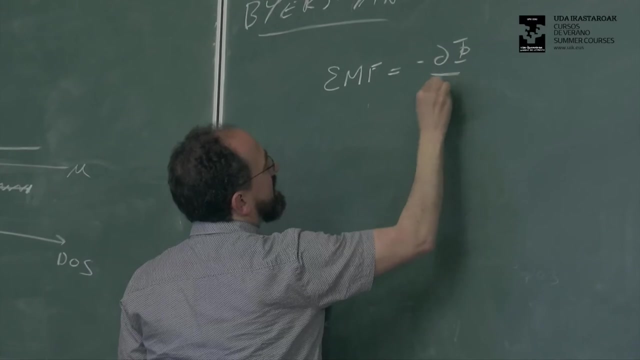 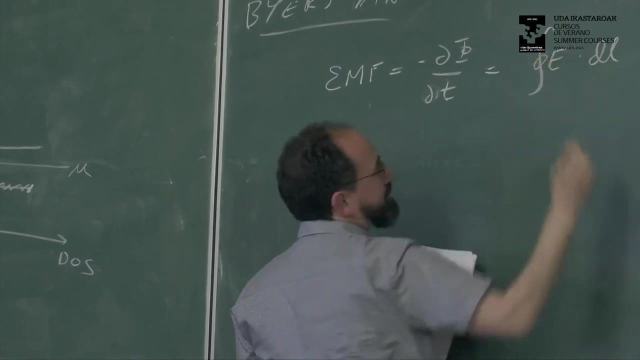 in the longitudinal direction. But as we change phi we know that there will be an emf. emf is minus d, phi, dt by faraday, dt, that's just integral of e, dot, dl around the loop. So that will be going. 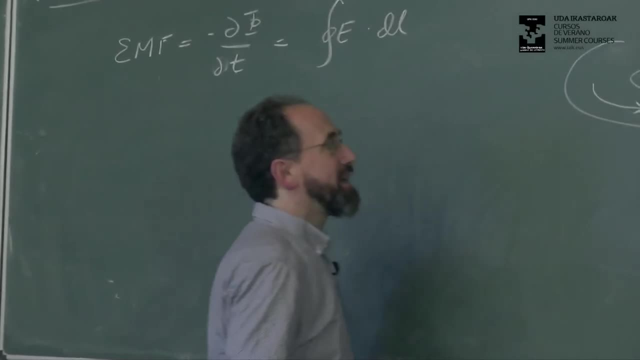 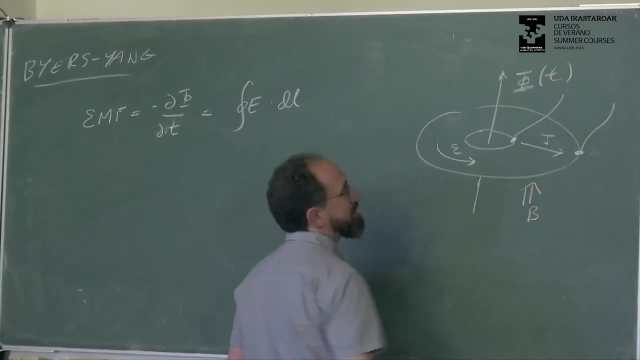 in this direction And then, if there is a Hall conduction, it will. so this is e going this way. If there is a Hall conduction, it will make a current from the inside to the outside. So j Hall is going to be. 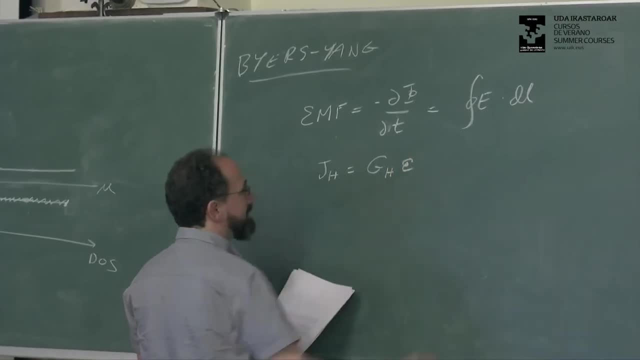 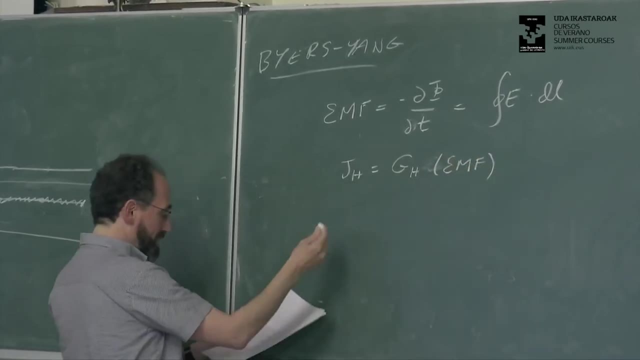 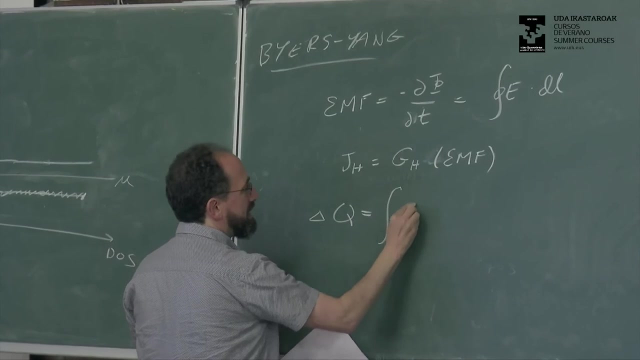 whatever the Hall conduction is, times the emf from the inside to the outside times emf And then we will just calculate the total charge that's moved from the inside to the outside. It's integral dt. j Hall of t. j. Hall of t. 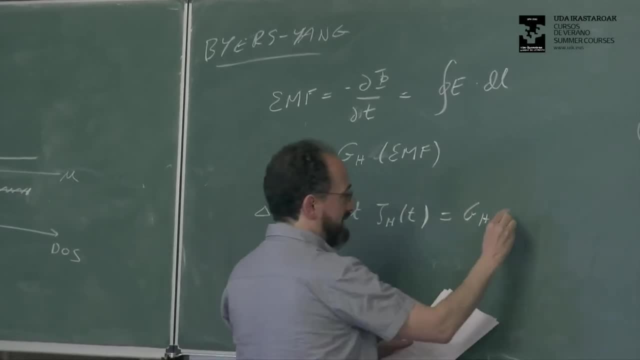 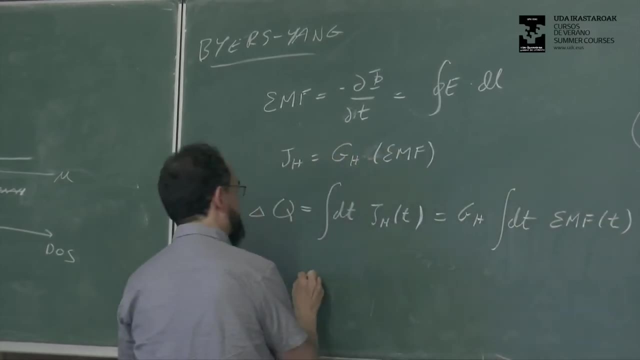 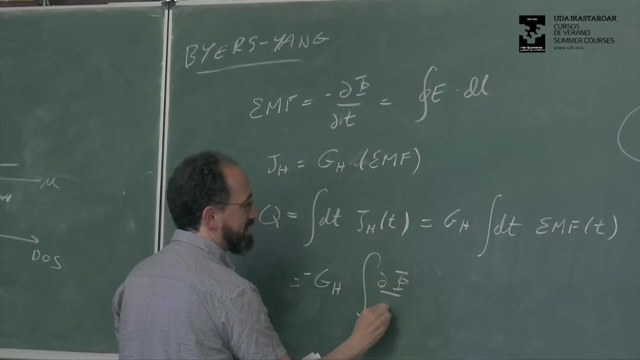 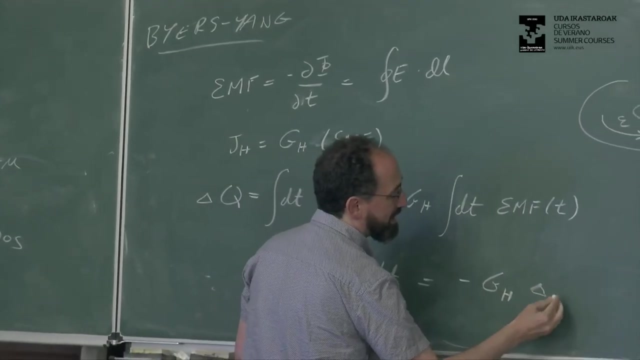 is. so this is j Hall times. integral dt, emf of t. The emf is d phi, dt. So this is now gh, I guess, with a minus sign. integral d phi, dt, dt. So this is now minus gh times delta phi. 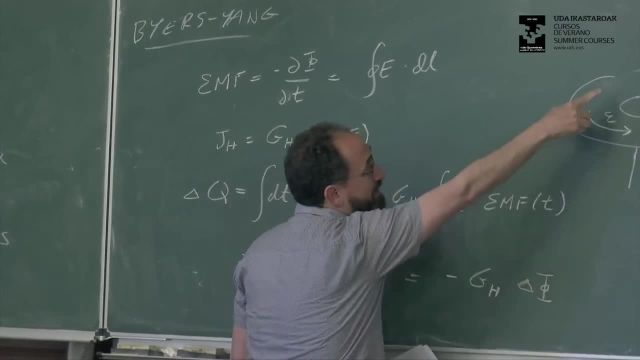 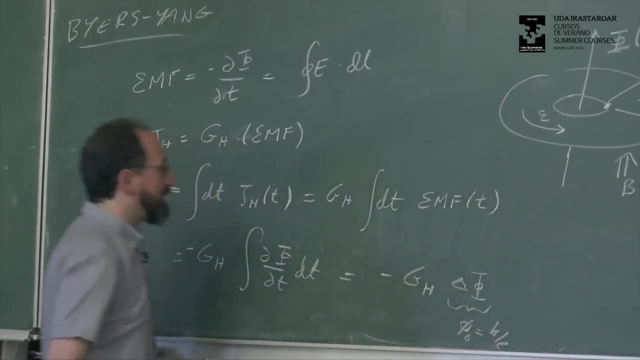 which we will set equal to one flux quantum. So we're charging up that flux until it's exactly one flux quantum phi naught, which is h over e. Okay, So the amount of charge is given by the Hall conduction times the flux quantum. 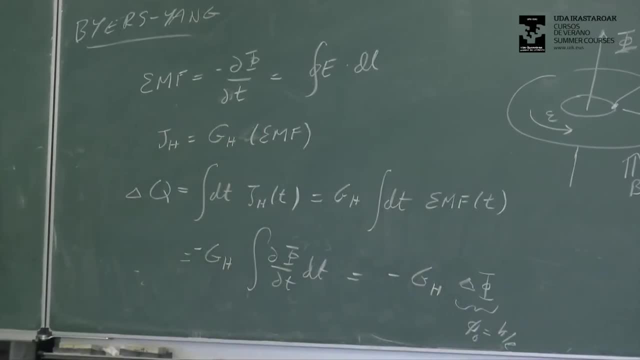 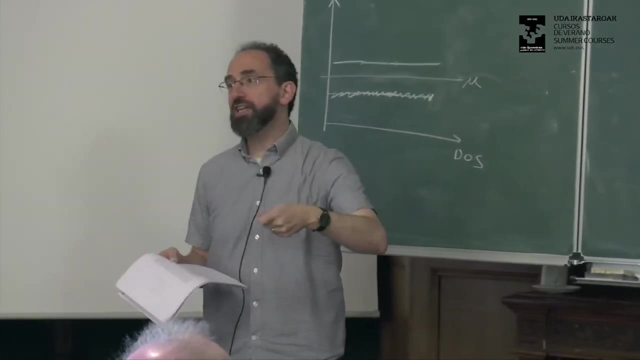 h over e is moved from the inside to the outside. Now the point is that we start in the ground state of the system. we adiabatically change until we get at exactly one flux, What we're guaranteed by the Byers and Yang theorem. 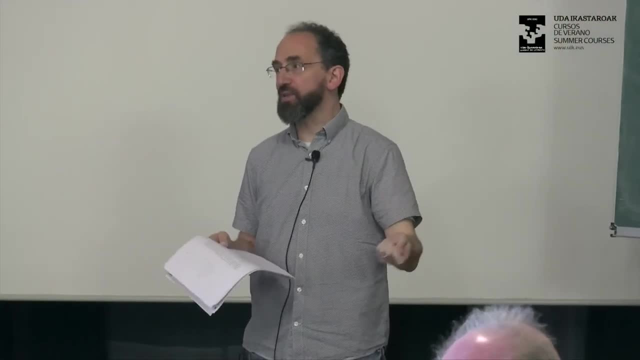 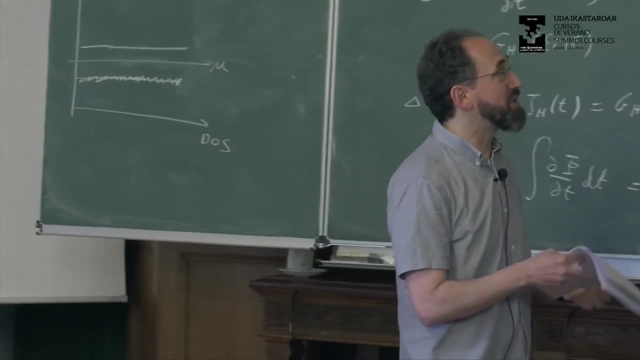 is that after adding one flux, you're back to exactly the same ground state. The only thing you possibly could have done in going from the ground state back to exactly the same ground state is you could have moved an integer number of electrons from the inside. 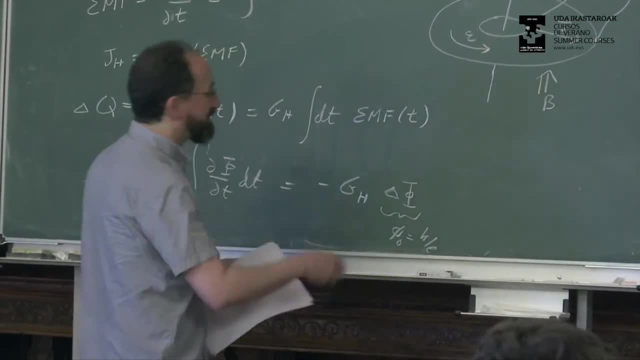 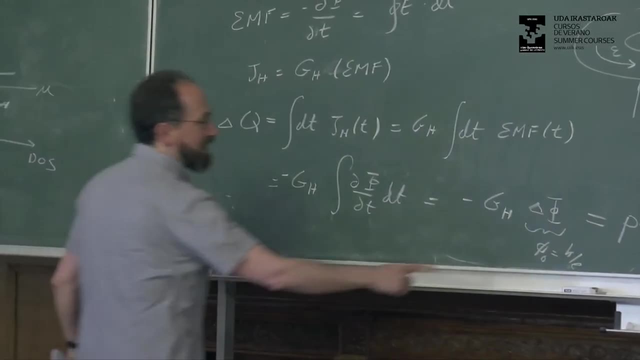 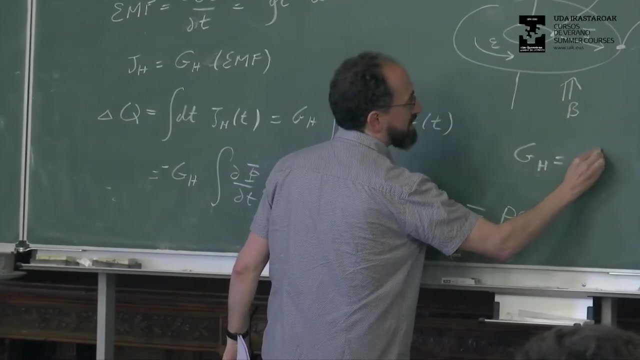 to the outside, The only thing that could possibly have happened from one reservoir to the other. So we'll set this now to an integer number of electrons and then, when we solve this equal to this, we get gh. is e squared over h? 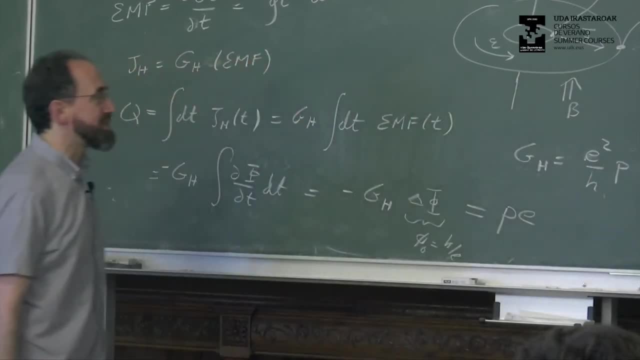 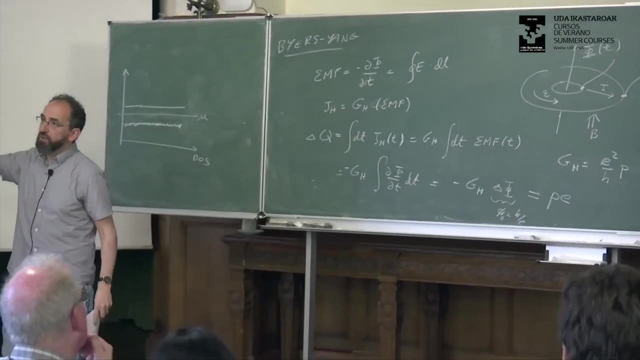 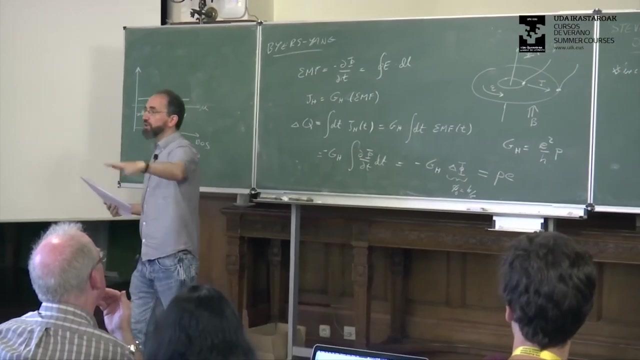 times p, where p is an integer. So the only thing we used is the fact that we put the chemical potential in the localized state. so there can be no current except Hall current. There can be no current that dissipates energy. There's no low energy excitations. 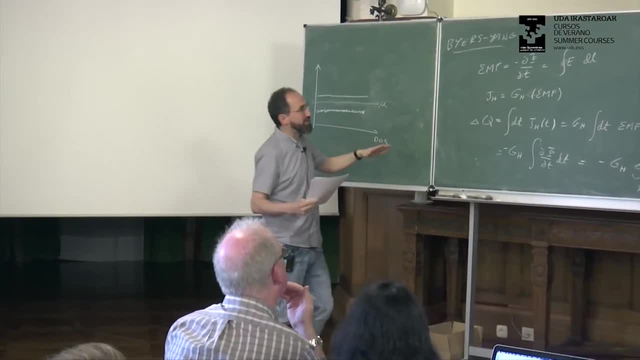 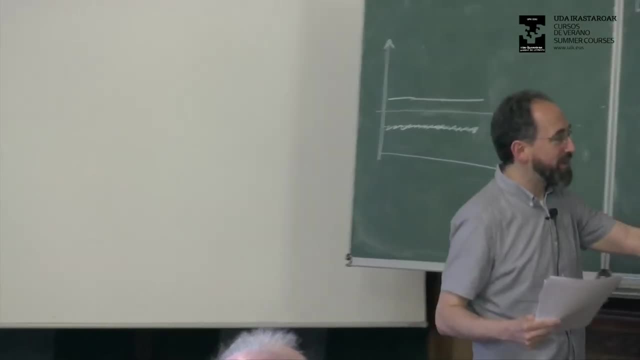 the whole way through the process- And we used gauge invariance- that you start in the ground state, you stay in the ground state the whole way and after you add one quantum of flux, you have to get back to exactly the same ground state. 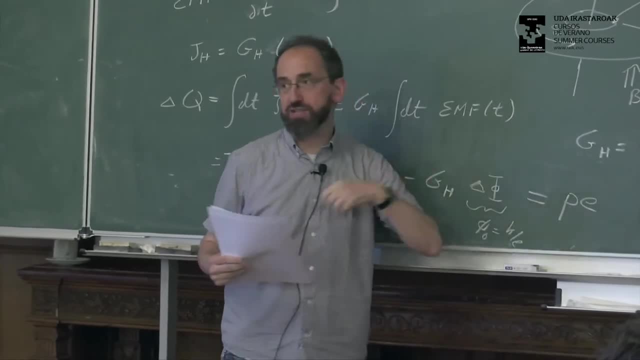 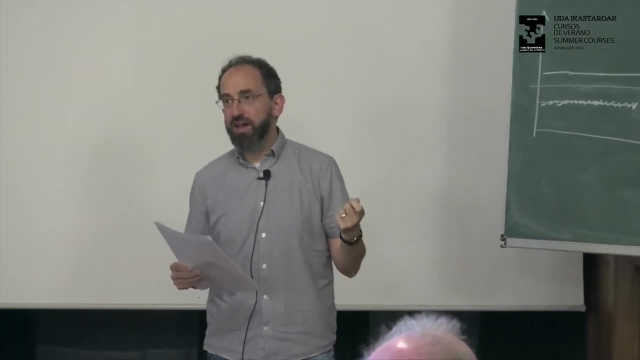 So the only thing that could have happened is that an integer number of electrons is moved from the inside to the outside. So in some sense the quantized Hall conduction is doing some sort of spectroscopy on the charge of the electron. You're measuring the charge. 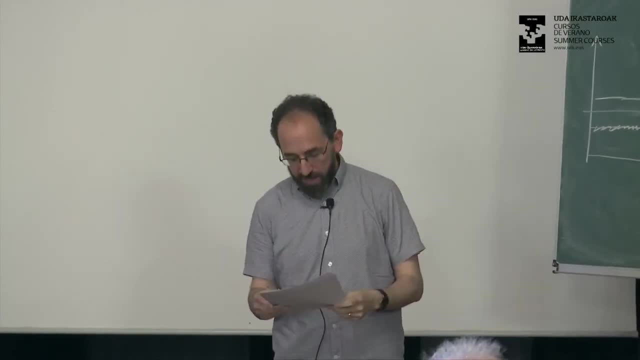 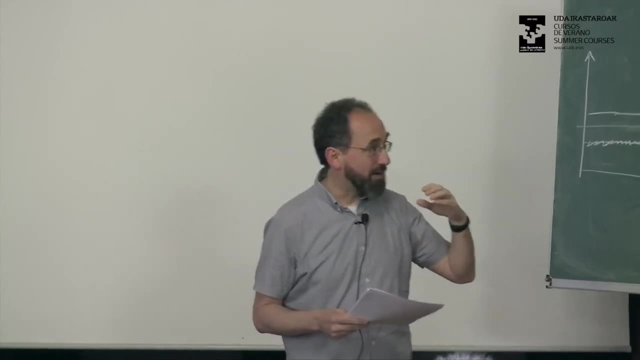 of the electron. You're counting electrons moved from one end to the other And this gives you the strength of the integer quantum Hall effect. And why it is that it doesn't matter if you add interactions between your electrons and you add spin orbit coupling. 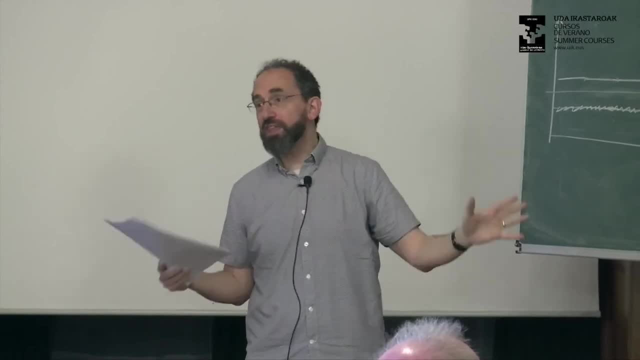 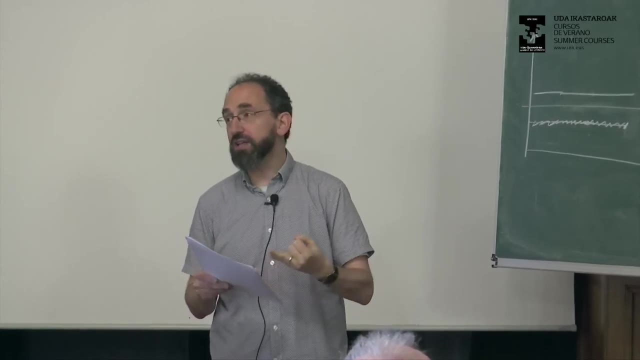 it doesn't matter if you add phonons. Almost nothing you can think of could possibly matter, because all we used is that you have localized electrons at the chemical potential and you have gauge invariance and that's it. Okay, I think I've already overrun. 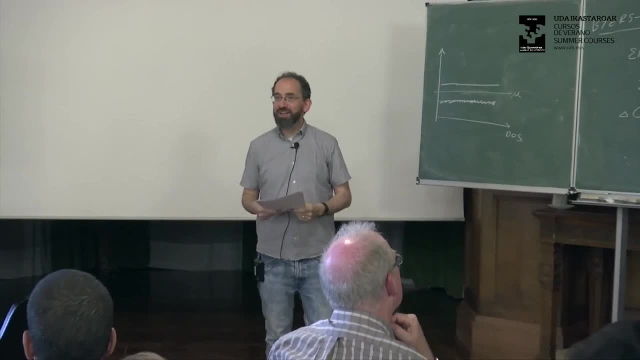 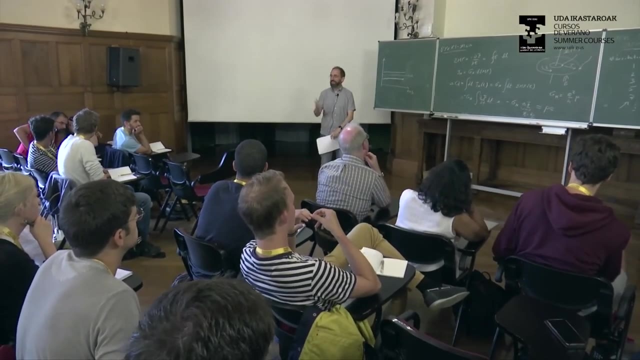 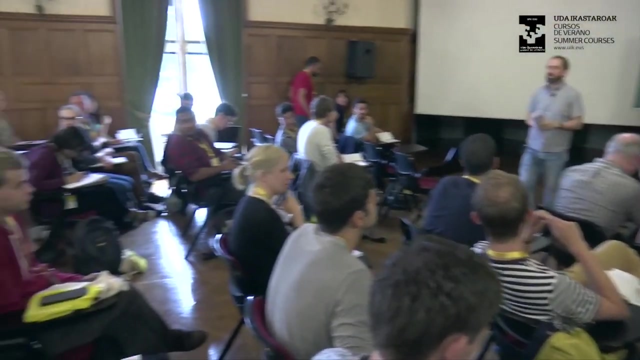 Have I overrun? I've overrun, Yeah, Okay, But I'll. And if there are any questions, please ask them now or over lunch, and then I'll start again after lunch. No questions? Yes, one question. So I don't have lecture notes. 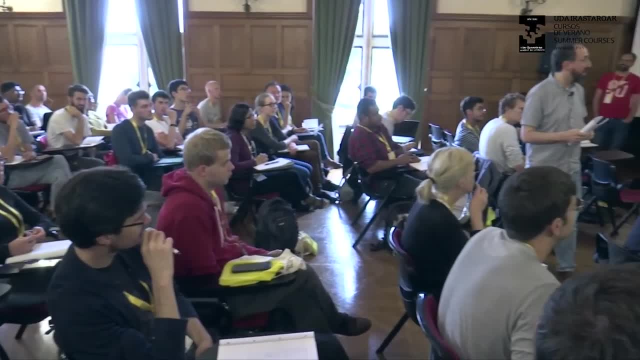 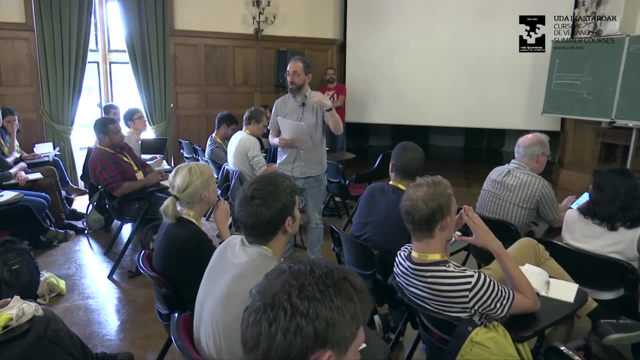 I only have homework problems on my website, But if you want, I actually do have. I have a book that I'm working on that you can also download from my website, which has a lot of this material on it as well. So it starts. 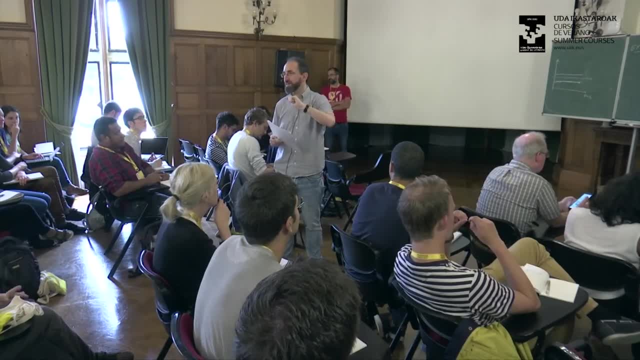 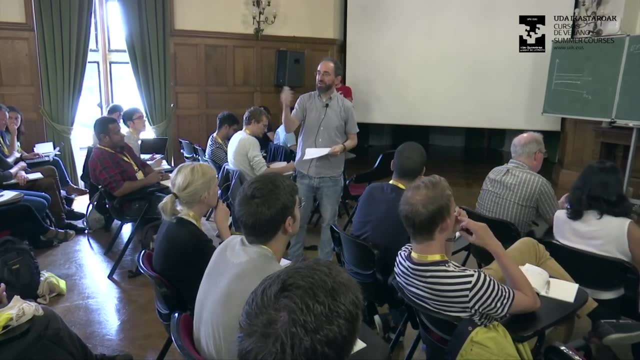 I mean it starts with all sorts of topological nonsense. but if you just skip ahead to chapter like 15 or something, it starts with integer quantum Hall effect there. So you can ignore the first 14 chapters, You'll be fine. 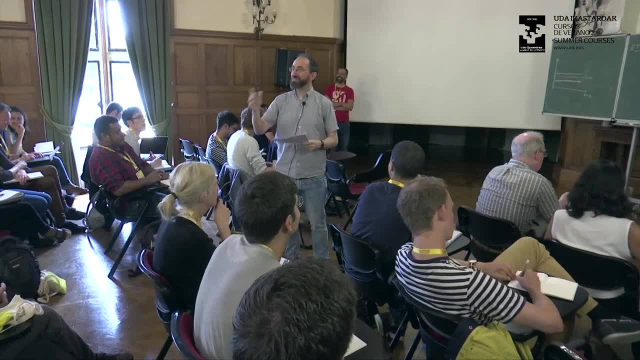 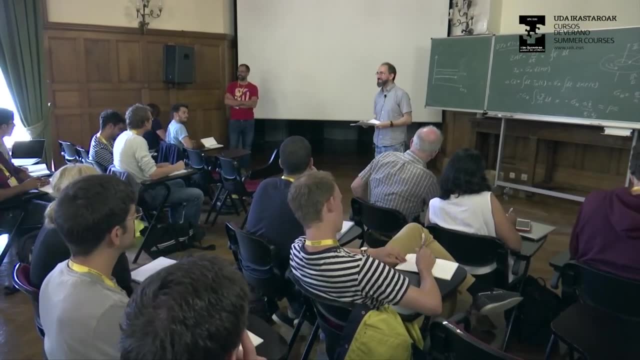 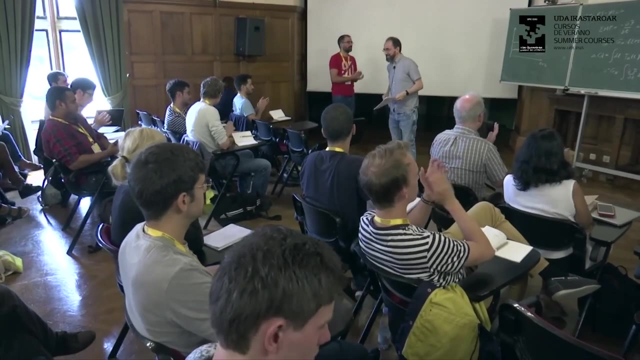 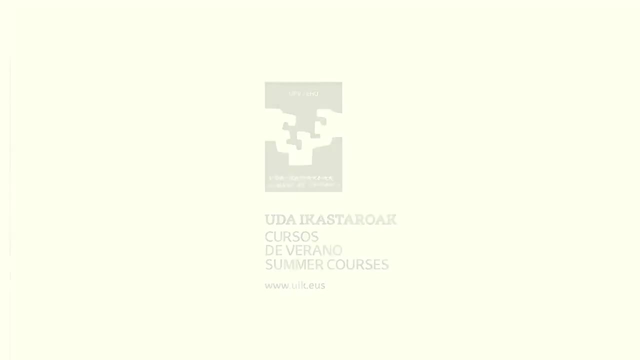 Okay, Thank you, Thank you, Thank you.